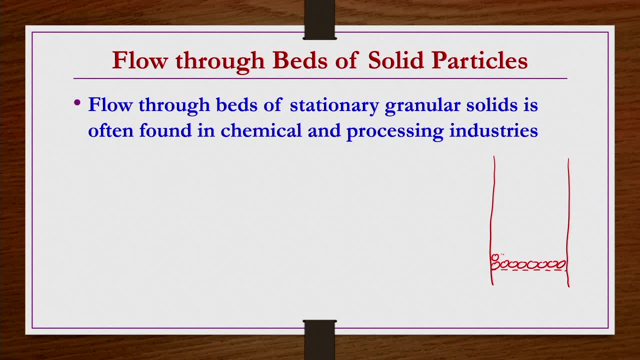 that you know we want. We are using them as a kind of a packing. They are placed on this perforated plate So that you know particle sizes should be, you know, more than the opening of the perforation or perforation plate opening, whatever these openings are there, So that should be smaller. 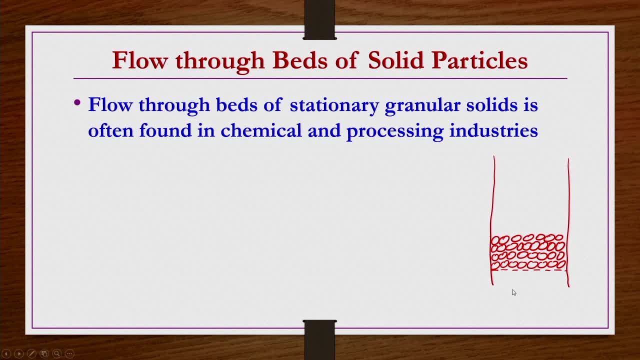 and then particle size should be larger so that you know they should not fall down. So then the particles are, you know, arranged like this. So sometimes you know this top perforated plate is also closed with a kind of perforation plate. So sometimes it does not, it not necessary. 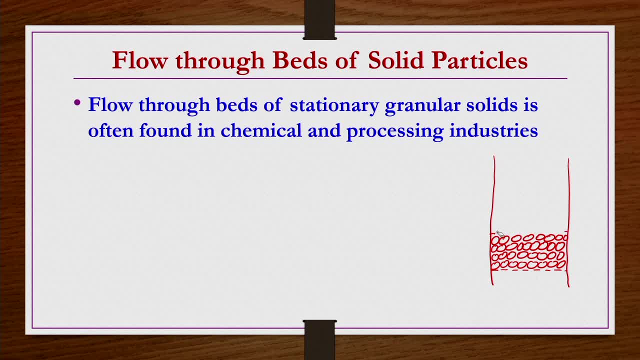 like you know, there is a kind of a closing at, you know, at the top. So when the fluid is allowed to flow through bottom like this, you know, if this bed is packed or closed from the top, then these particles will not move. They will be a kind of stationary granular. 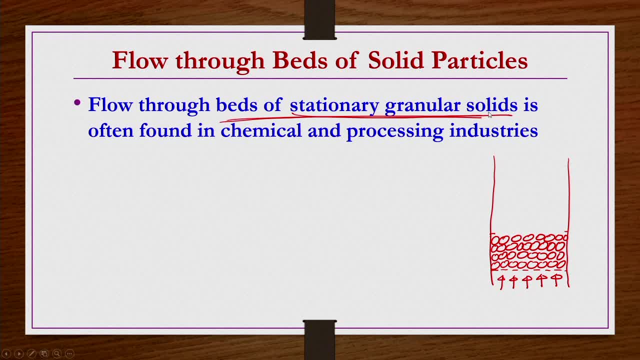 solids, like you know, bed of stationary granular solids. So that means fluid flow is only taking place or the only one phase, single phase flow, that is, liquid phase flow is taking place If it is not closed at top. sometimes what happens? you know kind of particles will raise, will come to the some kind of fluidizing conditions. 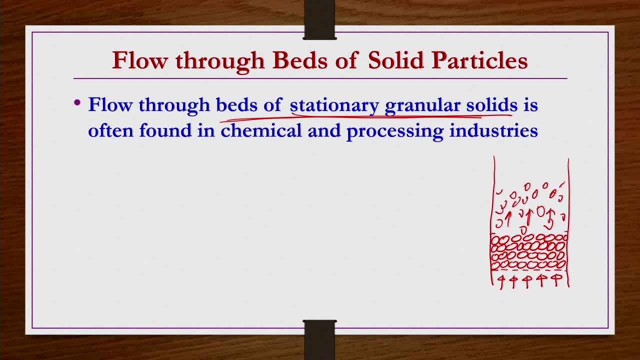 and then they will raise and then the motion take place. you know both the phases, like you know solid and then liquid phases. both phases will start flowing. or you know, solids are, you know, floated in a kind of floated conditions and liquids are flowing at a kind of certain 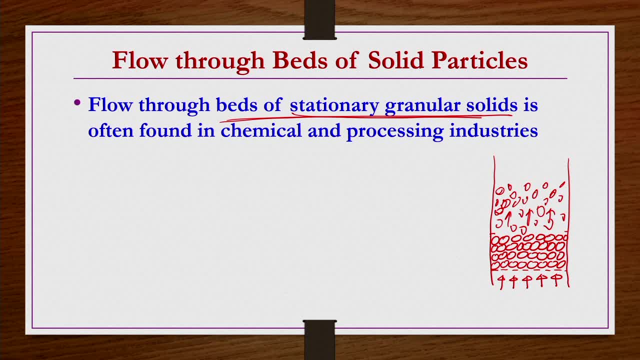 high velocities. So these kind of situations are, you know, usually known as the fluidized bed that we will be discussing in, you know, after couple of lectures. So let us restrict our discussions in this lecture only to the case where, you know, we have a kind of packed beds. 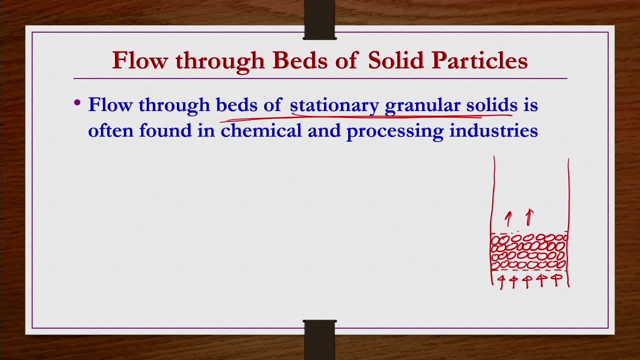 Right. So that is the top of these beds, you know are also closed with a kind of perforation plate, something like this. So these fluids are, you know, flowing through bottom and then passing through this perforated plate and then passing through this particle packing structure and then going out of the bed, Right. So in general, you know what we have, if you. 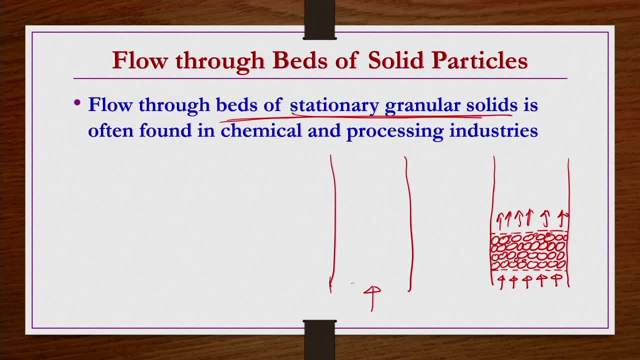 have a kind of single column like this. you know, the fluid just flows through and then fluid elements will travel The distance equal to the length of the pipe or the column, whatever we have taken Right. But here now, part of the column is, you know, packed or you know, mostly most of the sometimes. 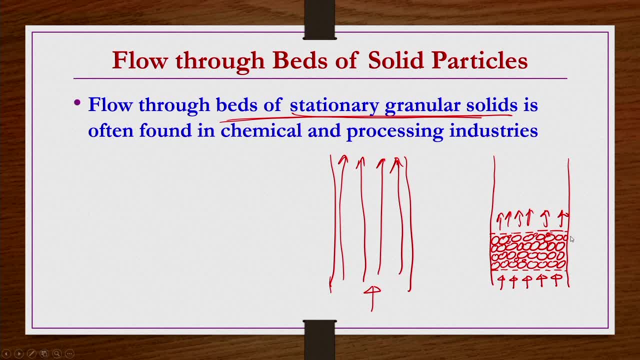 you know, entire column is also packed, you know. So let us take only this part, only packed. So then what happen? let us say, the fluid element coming here that may go from here like this, take this part and then go from this corner like this, or the same fluid element will take. 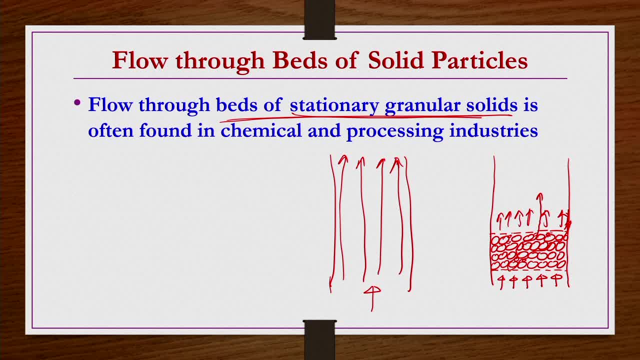 this part. So this one may go like this and then come out like this, or this one may go like this, like this and then like this, and then go this path like this, whatever that I have drawn, So that means you know it may take any part, depending on the resistance offered by the. 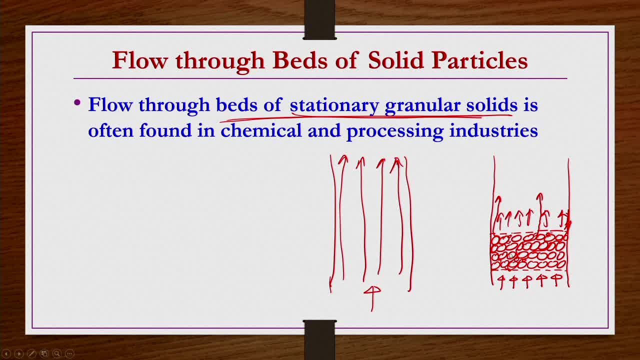 neighboring particle and depending on the size and shape of the neighboring particles and all that. Okay, So that means you know the packing length. let us say the packing length is L, So it is possible that you know particles are traveling more than this L distance. Right, So that. 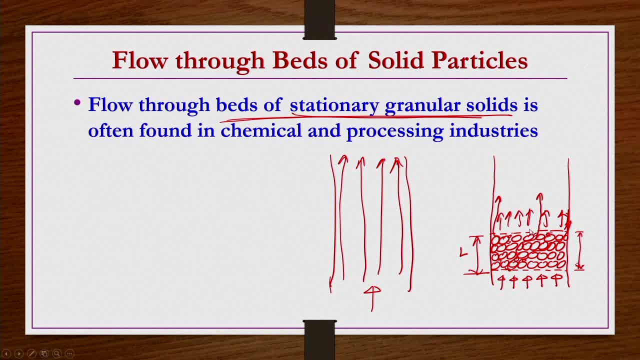 is possible distance more than this L distance because of this tortuous path. So that is one thing. So now, coming to the applications. why should we need kind of this kind of flow through packed bed should be studied. there are several applications. So here what we are going to. 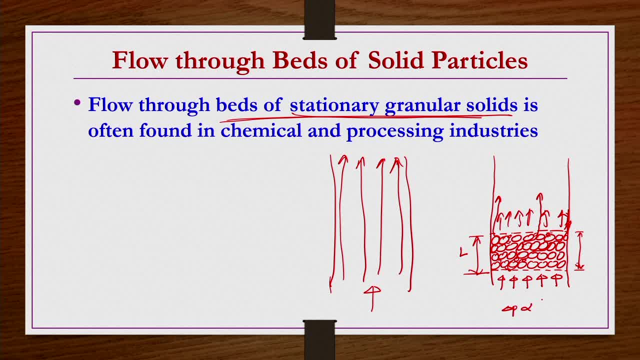 do? we are going to measure a kind of expression for pressure drop as a function of packing characteristics like porosity, tortuosity etc. and then particle size that has been used for the packing shape of the particle, then the density, viscosity of the fluid, etc. 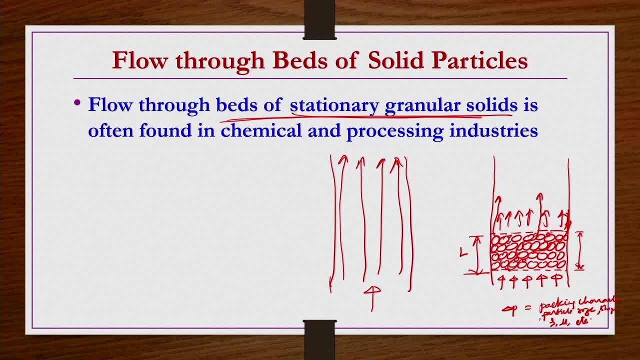 in terms of measurable parameters, including this L, also the height of the packing. So, in terms of measurable parameters, we are going to develop an expression for pressure drop, similar way, like you know, for a pipe flow, if it is a kind of, you know, laminar flow. 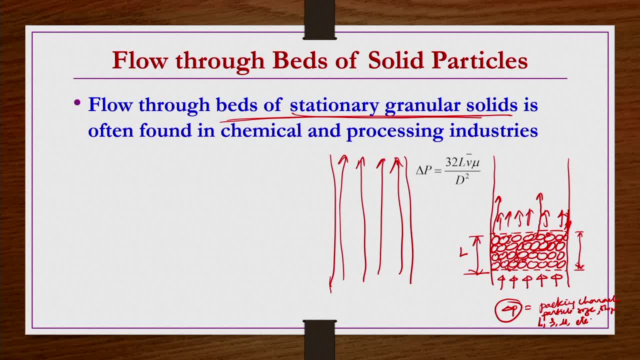 delta P by L is equals to 32 mu V by D square, or delta P is equals to 32 mu V L by D square. This is what we have already seen for Huygen Poiseuille equation. So corresponding equation here. what should it be? because here, in the case of packing, there is no kind of abstraction. 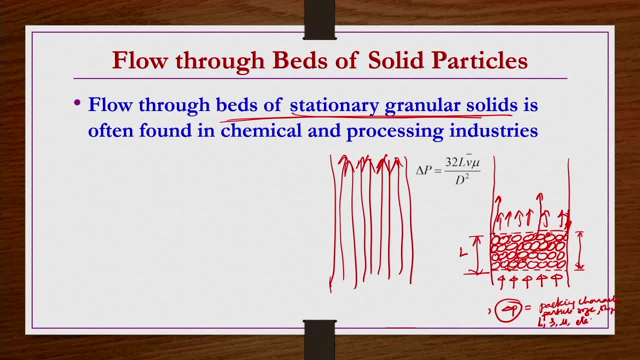 So they are simply flowing through. But here there are large numbers, There are large number of particles are there. Each particle may be offering some kind of resistance to the motion of the fluid. So the overall resistance offered by the early particle, that should be the overall resistance. 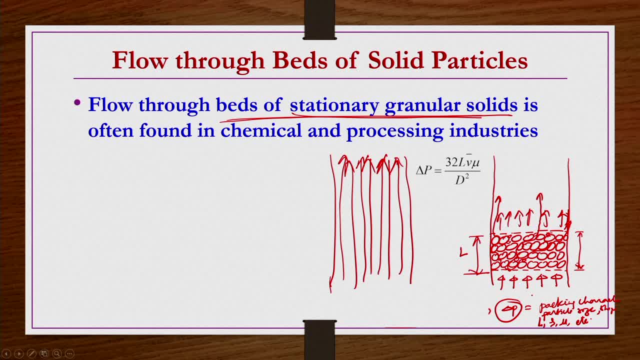 experienced by the fluid particle to pass through this kind of channel. So this is what we are going to see, basically, right. Then coming to the applications in general: what happens? So, catalytic bed reactor, let us say, in H2SO4 plant, what happens? 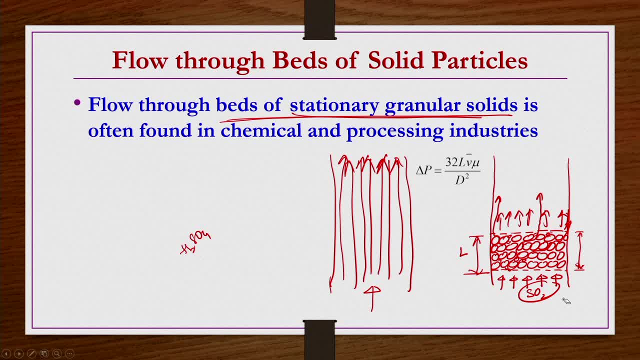 So there is a SO2.. So in general SO2 is in H2SO4.. Right, So in H2SO4 plant SO2 is there that will be passing through a kind of a catalytic bed. So catalytic bed, so that is catalytic bed or catalytic reactor. 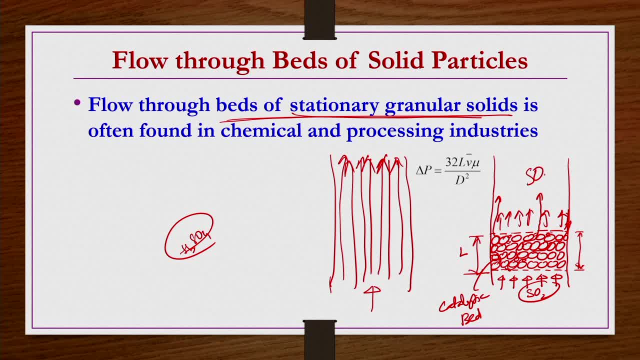 So then here. so whatever the SO2 comes out, that will be reacting in the presence of this catalytic bed, So that will be forming SO3 and then that will be further absorbed into water in order to produce the H2SO4, like that. 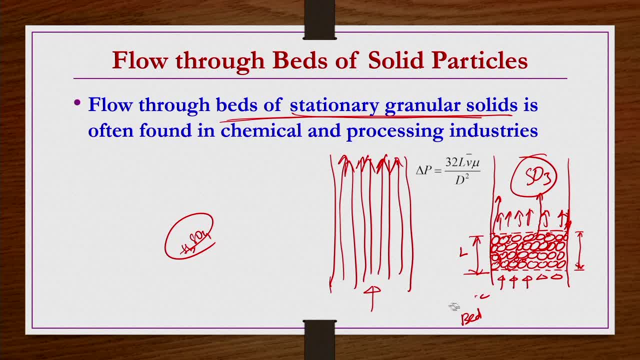 That is one kind of example. So another examples: you know, drying, drying of materials, you know. you know, sometimes you have a kind of a silica gel, et cetera, molecular sieves, et cetera. here in order. 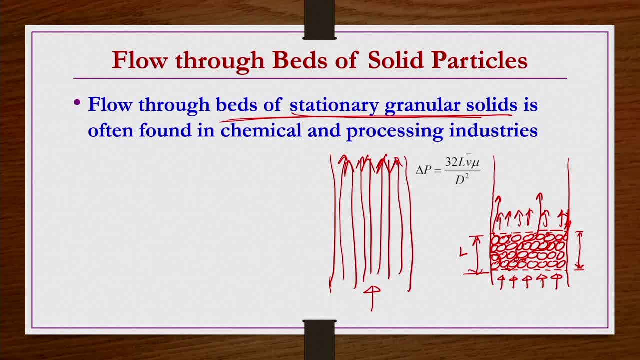 to fulfill this drying aspects. And then also we have a kind of some time. you know this, you know heat recovery system. So let us say high temperature fluid is coming here, So whatever the heat that high temperature fluid is carrying, that will be absorbed by. 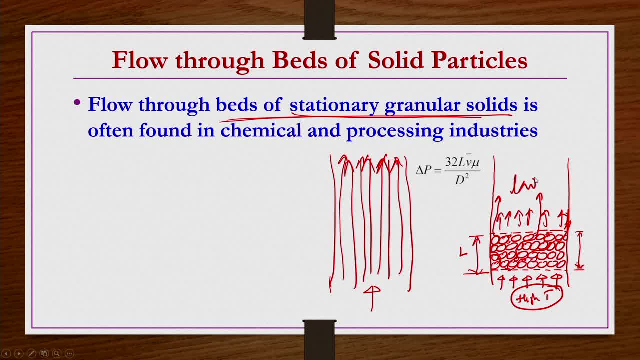 this packing material here and then the fluid will be going as a kind of low temperature or ambient temperature fluid after passing through this bed, right? So then whatever the heat is there, that will be heat storage kind of things. So this heat storage maybe sometimes, when required, that can be, you know, recovered. 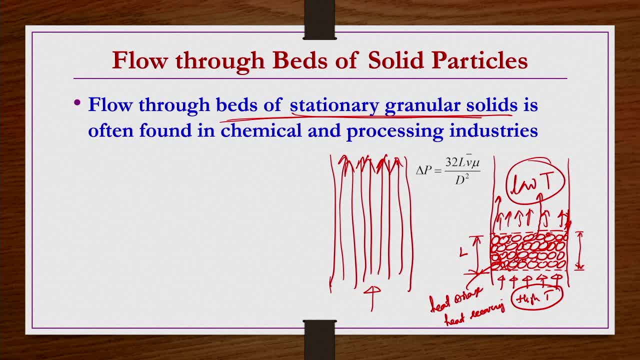 for the. you know some other applications. let us say Then, when you wanted to do the recovery of the heat, You can pass through a fluid. There is a fluid which is having the low temperature and then, when it pass through, it may be carrying. 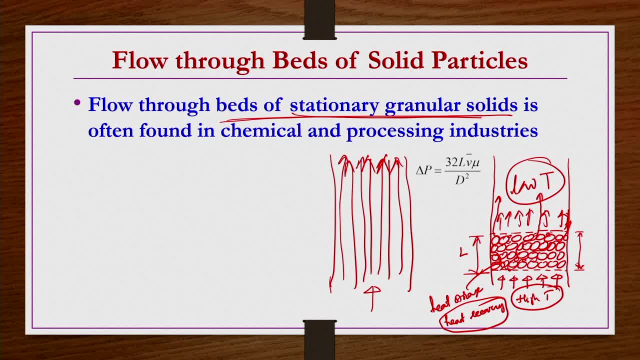 the energy from the, this heat stored, packing material and then maybe going out as a high temperature. that is also possible. So both heat storage and then heat recovery. also this packed and fluidized beds are in general used. Then we have a kind of- in general you know- filtrations. like you know, when we do the 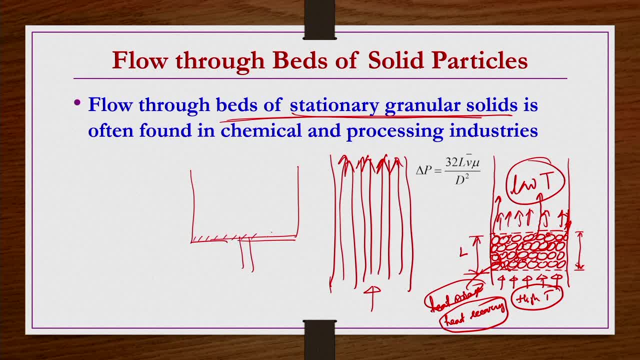 filtration. there is a kind of filter paper here in general, like this at the bottom in a container, Right, So this slurry or this suspension comes out here, right, And then some kind of pressure- you know delta P- is applied. you know some pressure. 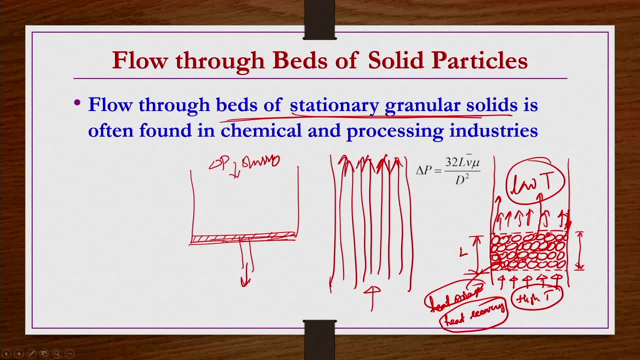 is applied or there is a kind of vacuum at the bottom. either way it is possible, right? So then when you take this slurry here, so the particles, you know they may be settled at the bottom here like this. Okay. 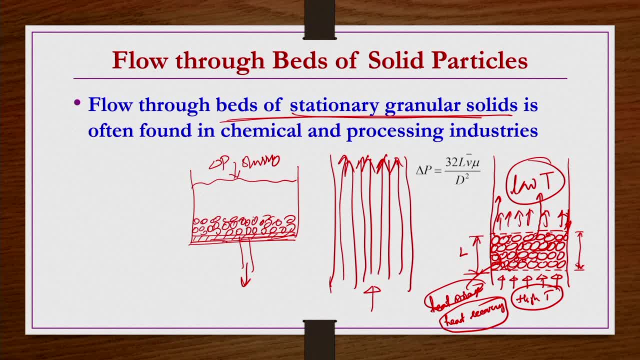 Okay, Okay, And then clear liquid may be collected at the bottom. So in these cases also, this is you know down flow. this can be treated as a kind of down flow packed bed. Whatever, the examples I have shown here are kind of you know up flow packed bed kind. 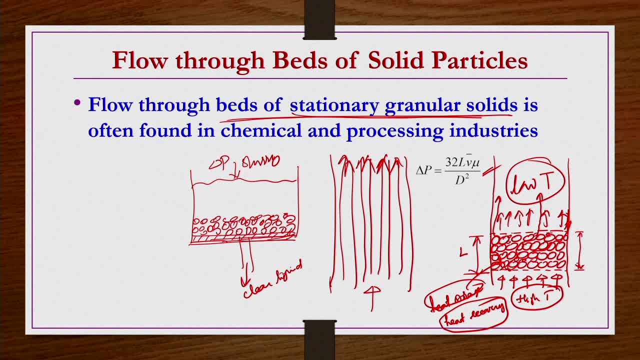 of things. So it is possible: down flow, up flow. both of them are possible, depending on the applications. Okay, So here this: whatever the particles these present in the suspension, They are going to offer some kind of resistance once they settle on a kind of filter medium. 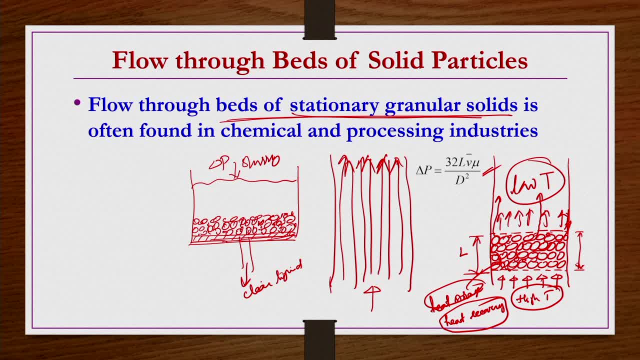 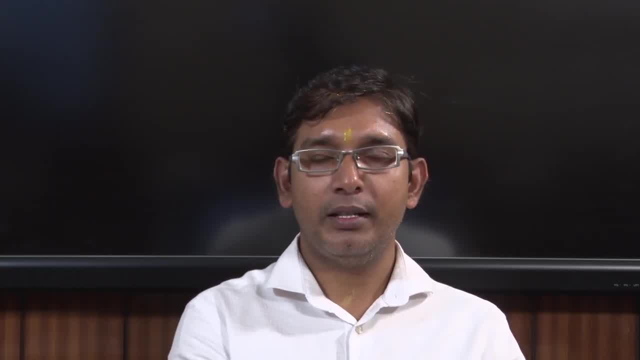 So this can also be taken as a kind of an example. where packed bed flow through packed bed is taking place, Initially only the filter medium is resisting, providing the resistance to the flow. So that is allowing only fluid element to pass through and then retaining the particles. 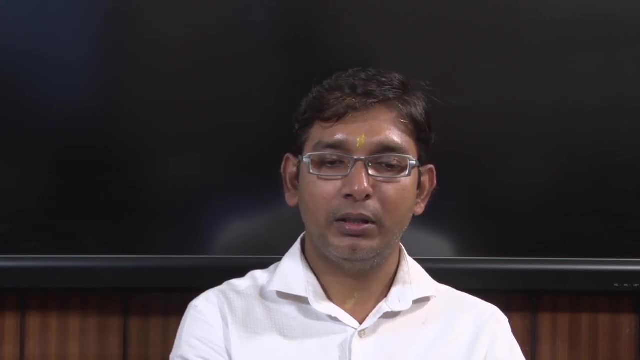 so that the separation is taking place, But gradually, as the process progressing- Okay, As the process progressing- these particles may be settling on the surface of this filter medium, So they are also additionally adding resistance to the flow for the later coming in slurry. 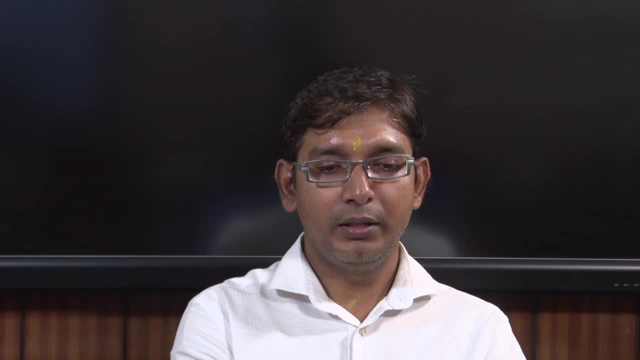 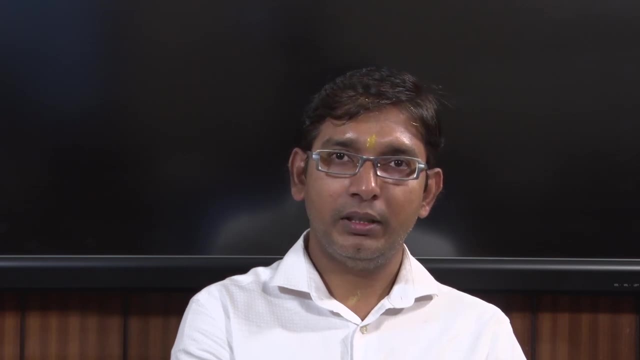 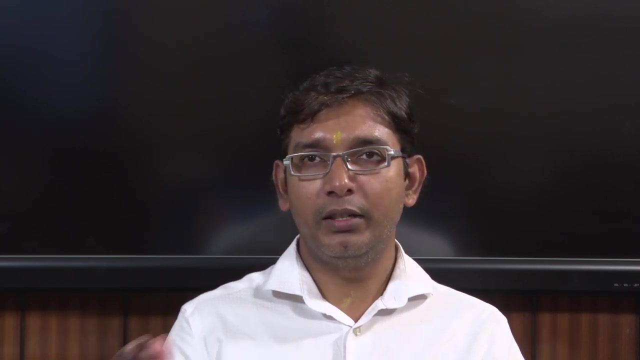 Right, So there will be two resistances: One resistance due to the filter medium, another resistance due to the settled particles. Okay, So in the next module we are going to discuss the filtration aspect. So there we are going to see the equation that we are developing in this lecture. 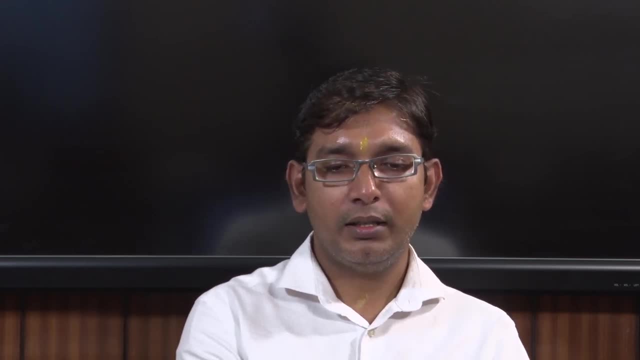 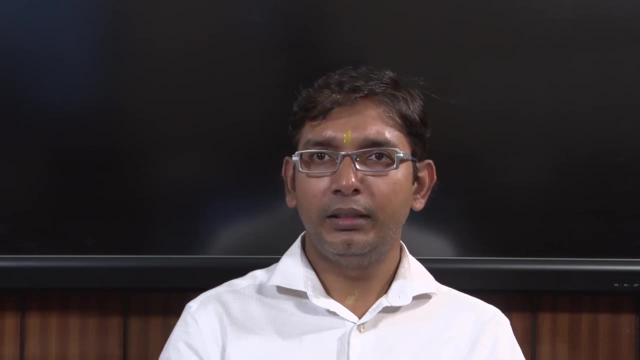 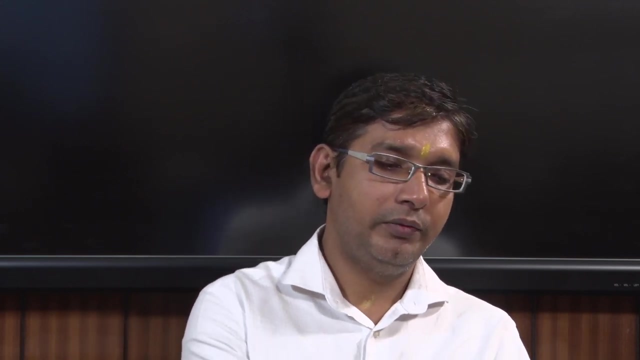 Are going to be useful in order to understand what is the resistance offered by these particles in designing of this filtration equipment. Okay, So there are only a few reactions or few examples I have shown here. We have a kind of you know, some examples we have seen there is a kind of reaction taking. 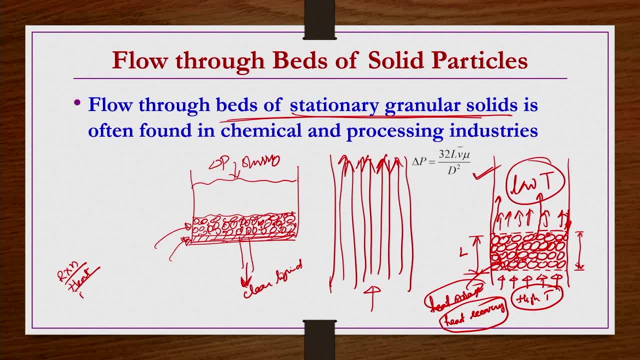 place. There may be a kind of heat transfer, heat recovery. There may be sometimes some kind of mass transfer also taking place, Right, Okay, Okay, So all these three may be taking place or individually, or they may be taking place together along with the momentum transfer. 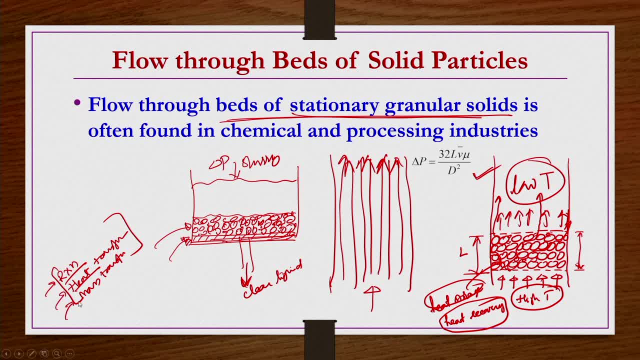 So, whether the reaction is taking place or heat transfer is taking place, mass transfer is also taking place in addition to the momentum transfer. So, whatever this study that we are going to do here, or analysis that we are going to do, that is going to be there in all of these things. 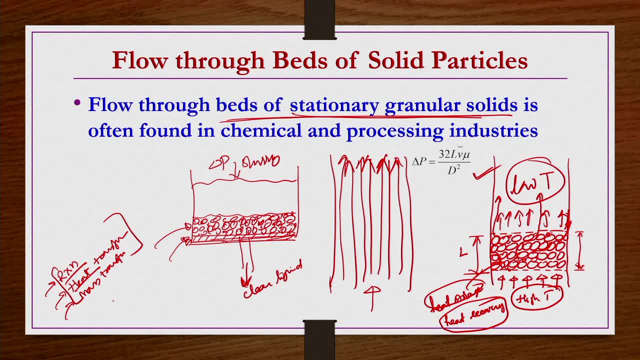 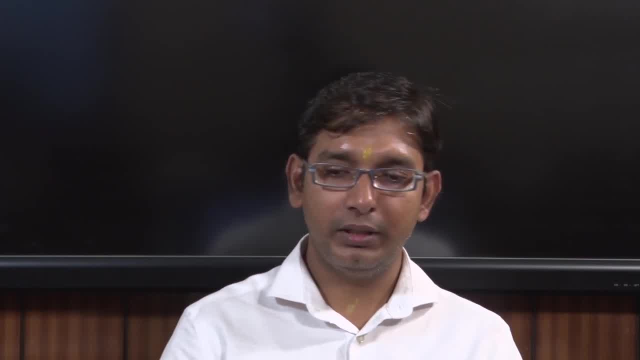 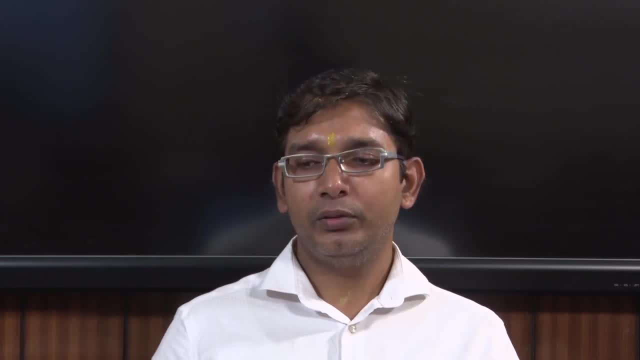 Right. So that is whatever this reaction, heat and mass transfer are expected to carry out here in this packed bed. They will not be possible unless there is a kind of momentum transfer. So there is a transfer of the momentum. So how much pressure drop is required for a given flow rate of liquid to flow through? 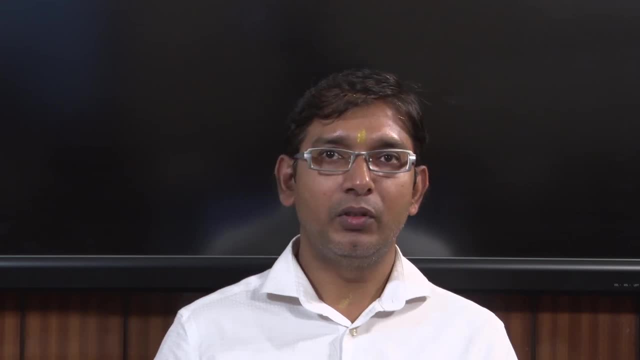 a packed bed of having certain characteristics, like you know: void, age, particle size, packing particle size, dp, etc. those kind of things. So this dp, we are going to find out. Okay, Right, So this is the purpose that you know. we need to understand flow through beds. 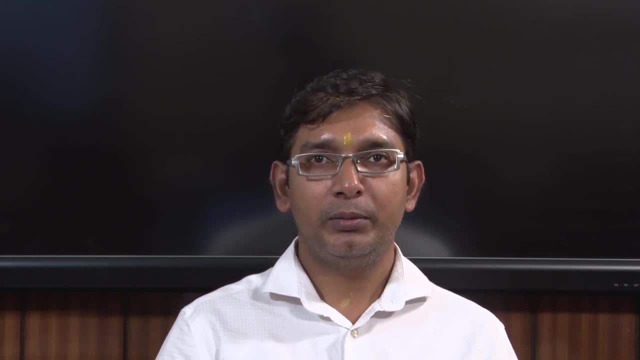 Beds of solid particles, though we know the settling of individual particles or free settling, and inter-settling of particles or suspension we have already seen. So, despite of that one, we need to understand flow through beds of solid particles because of given so many examples here. 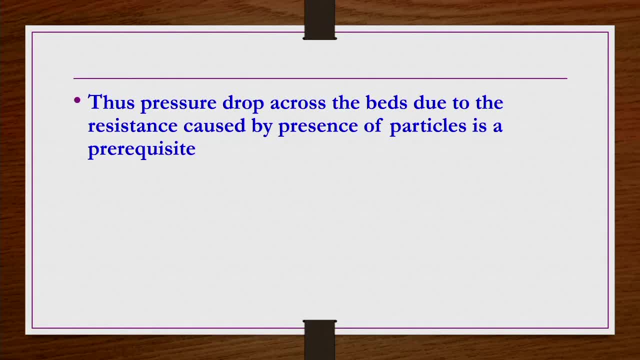 Okay, So what we understand, the pressure drop across the beds due to the resistance caused by presence of particles is a kind of prerequisite, because we have seen, you know, these examples, several examples. For example, the fluid is flowing through packed bed and then, when it is flowing through, 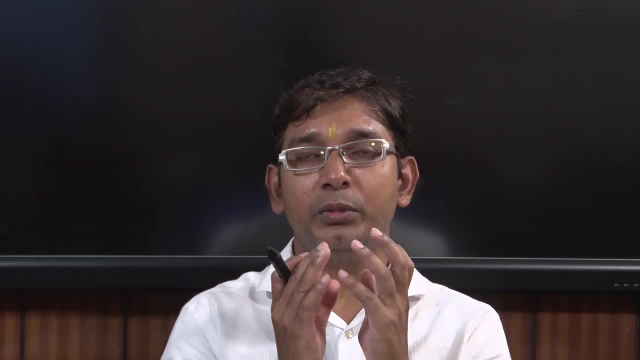 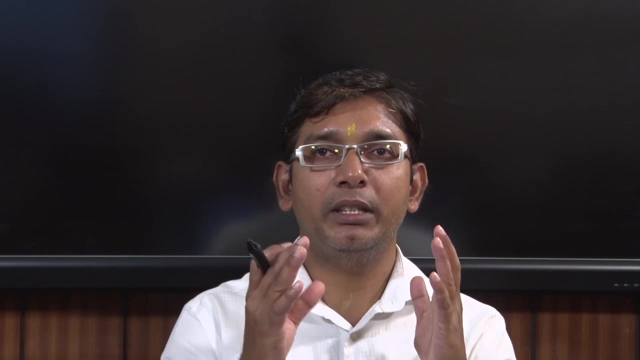 the bed it is offering or it is receiving so much of resistance because of the particles that are, you know, used for the packing of the column, which is forming a kind of packed bed Right, So this particle are offering a huge amount of resistance in general. 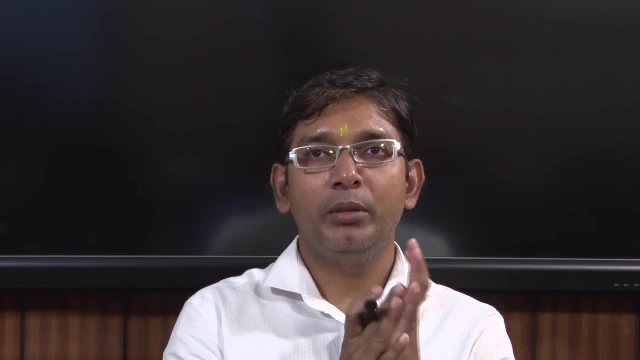 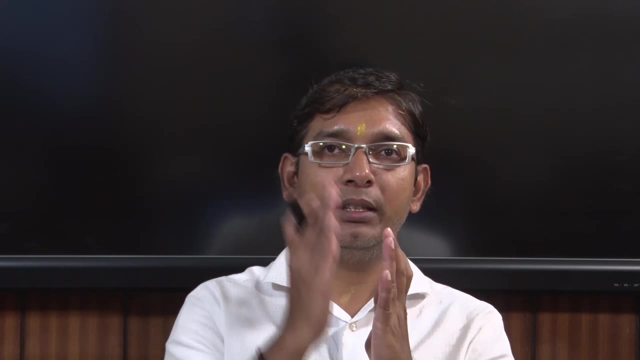 So that is going to be very much important. Let us say: you know pressure drop for the same pressure drop. you know, if you allow a fluid to flow through a single column You may be getting higher velocity, something like you know, 1 meter per second. 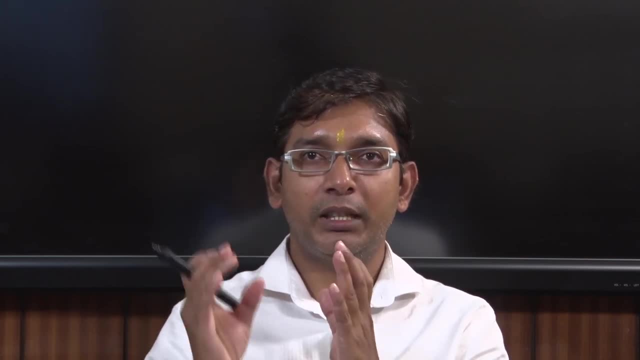 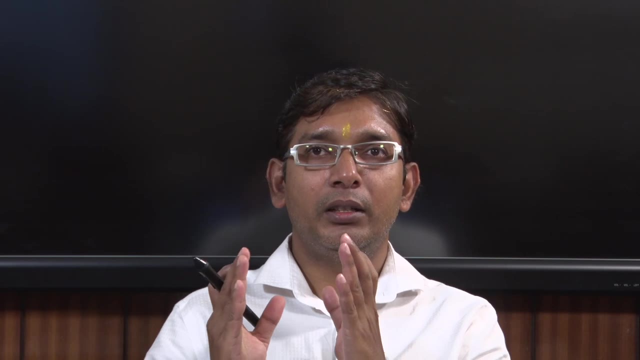 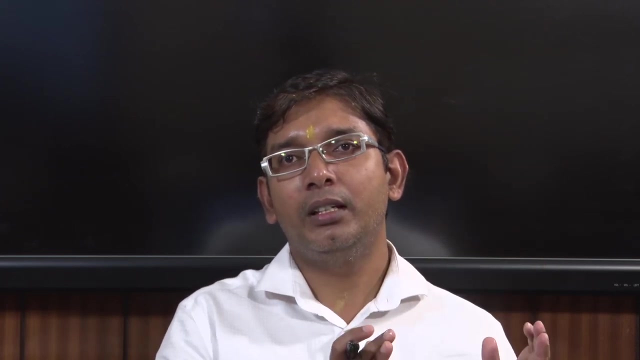 But under the same pressure. and if you do the column with some kind of packing of, let us say, void is 0.4 or 0.5, and then you apply the same pressure, then whatever the velocity that you get, that will be much more lesser than the 1 meter per second of the individual. 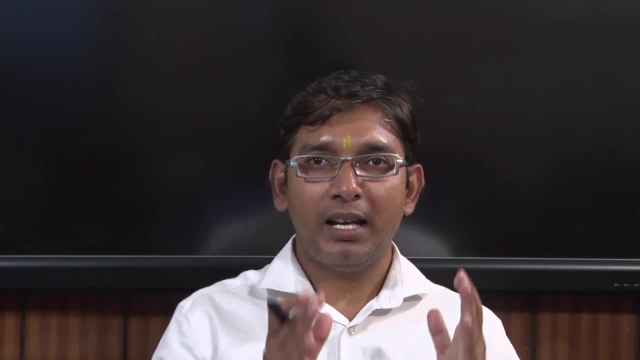 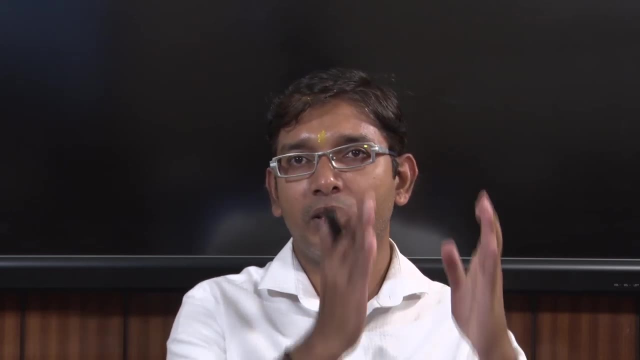 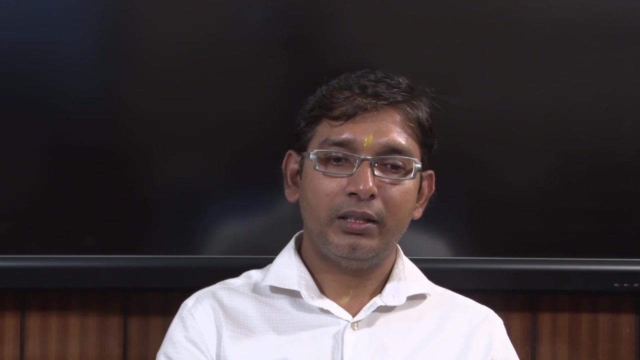 column without any packing, right. So that means you know the velocity. the average velocity in a kind of packing is also very much different compared to the average velocity. whatever we expect to have a kind of single column without any packing, okay. So that is the reason. so pressure drop here is going to be very much important in designing. 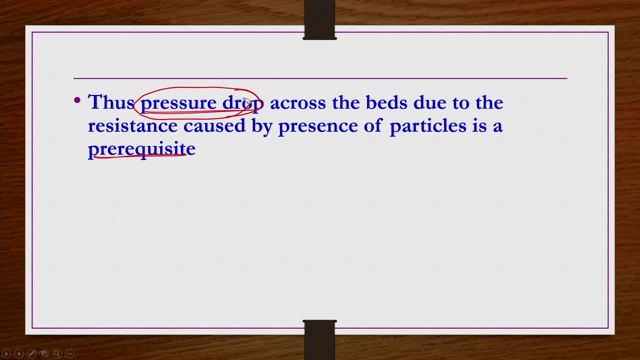 of this. you know equation, So we have to find out, you know proper way, how to find out, this pressure drop for a given system. Further packing materials in general. they can be spheres, they can be irregular crushed particles. they can be cylindrical particles, small cylindrical particles. they may be. 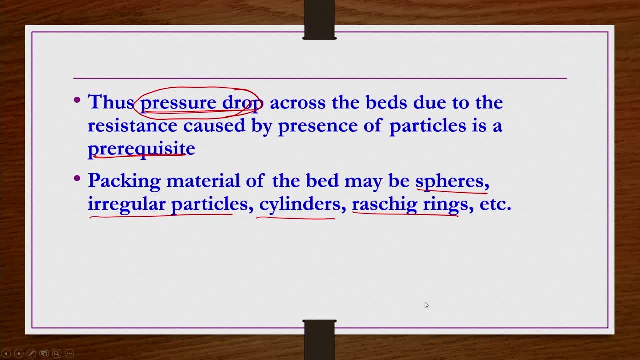 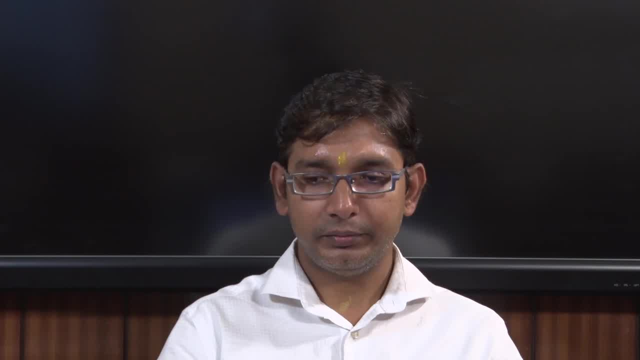 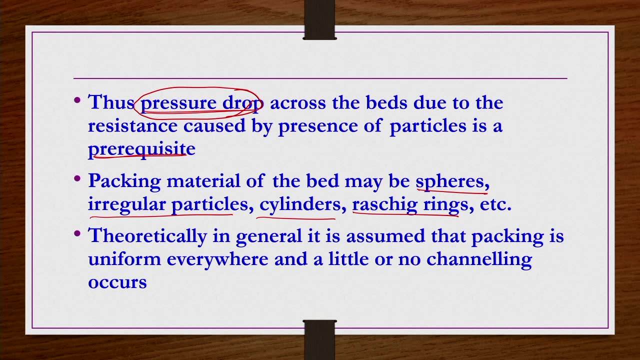 small ration, rings etc. They can be anything. usually you know spheres or cylinders or crushed glass particles etc. in general used a kind of packing material, right? So in general you know in reality when this bed is forming. if the particles are of uniform size and shape, then there is a possibility that whatever the packing is there is forming. 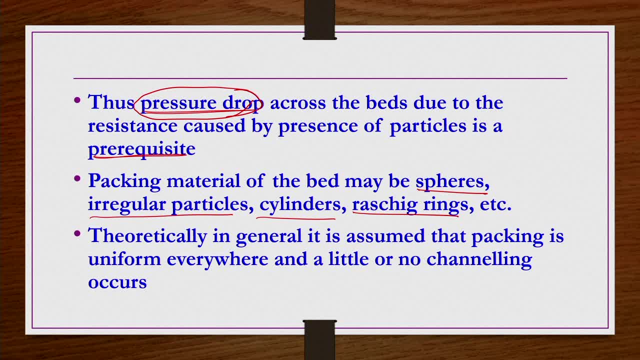 a kind of uniform packing is taking place. But if you have a different size particle though same shape- let us say you have a spherical particles shaped spherical but different size particle- 1 mm, 2 mm and then let us say 5 mm particles- if you use the packing is not going to be uniform in general. 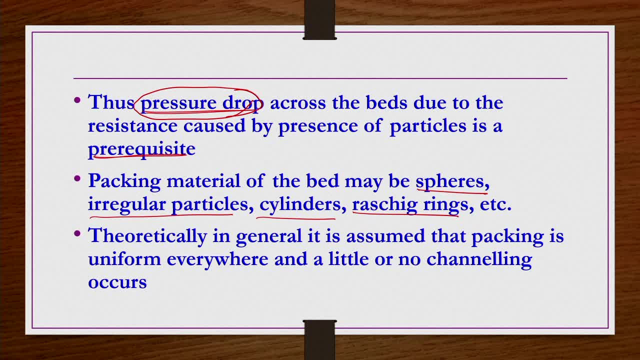 And then further, if both size and shape are not same, if you have some spherical particles, some cylindrical particles as a packing, So it is not going to be uniform everywhere Within the bed right. Further, if you have a kind of irregular particles, crushed particles, something like that as a 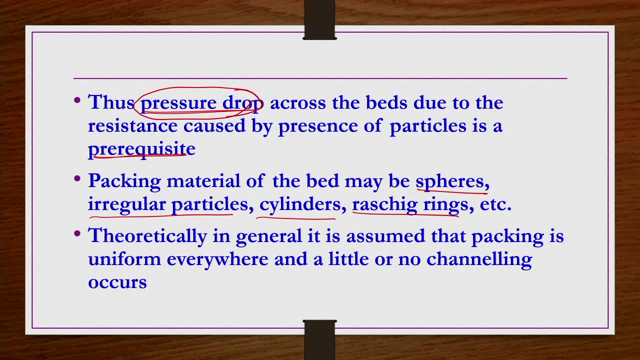 kind of packing, then the packing is going to be varying from one point to the other point, But theoretically, what we assume and whatever the analysis that we are going to do, we assume that the packing is uniform everywhere and there is no or little channeling occurs. 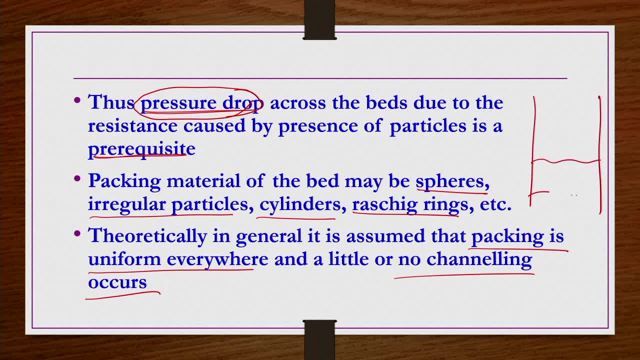 Channeling in the sense, like you know, the bed is there, let us say, this is the bed. so within this bed, somewhere, you have a kind of you know this kind of channels which is allowing the fluid element to flow through without any kind of hindrance, kind of thing. 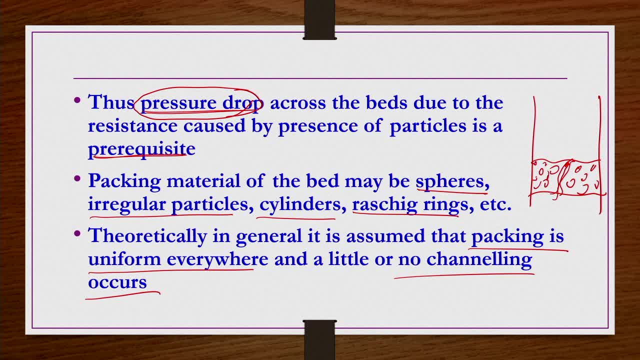 So particles are being segregated and forming a kind of channels kind of thing, right? So because of this channeling, you know the particles, you know fluid element may be offering. the fluid element may be receiving a little bit less resistance. but that is not going to be useful in many cases, especially if there is a kind of heat transfer or resistance. 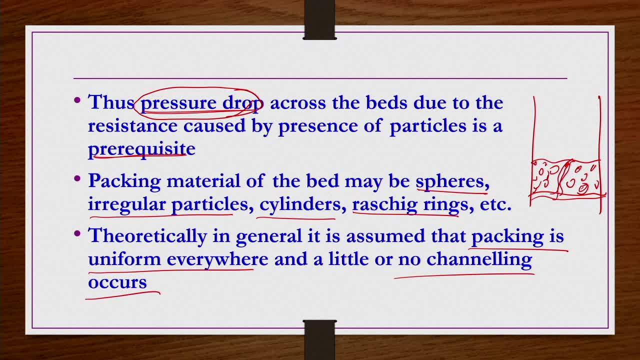 So it is not going to be useful in many cases, especially if there is a kind of heat transfer or resistance. Okay, So this channeling may be occurring in general in reality, but we assume that channeling is very less or almost there is no channeling. 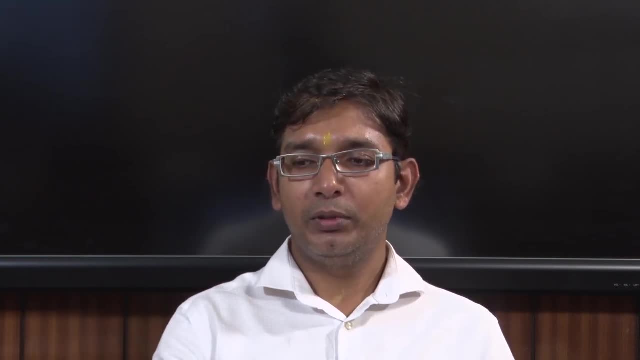 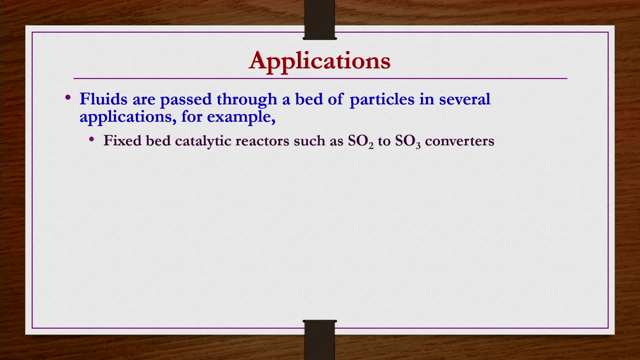 So this is what we, some basics, what we are going to do about these things. okay, about the packed bed. So then, coming to the applications. once again, fluids in general, liquids or gases, are passed through a bed of particles in several applications, For example, fixed bed catalytic reactors, such as you know, SO2 to SO3 converters. 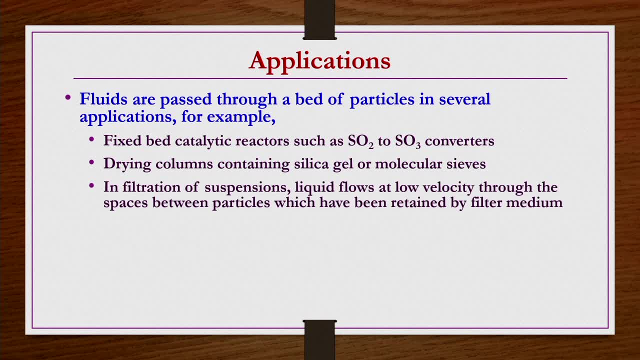 Then drying columns containing silica gel or molecular sieves. Then filtration of suspension. liquid flows at low velocity through the spaces between particles which have been retained by filter medium as explained Then sometime. deep bed filtration is also used on very large scales for water treatment. 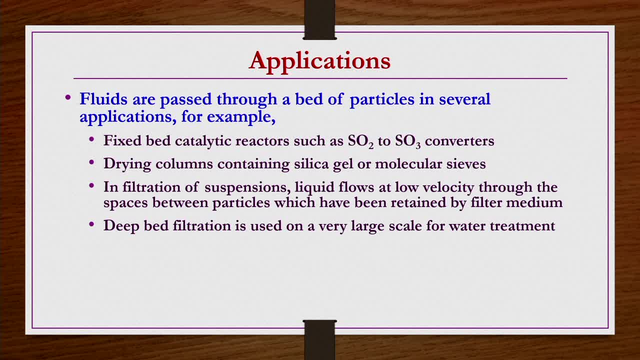 but, however, in such applications, the you know particles that are being settled. You know very few particles. okay, Pressure, drop of flow through a bed of small particles provides a method of measuring external surface area of powders such as cement or pigment. So cement or some kind of pigments, particles are very small, very, very small, you know. 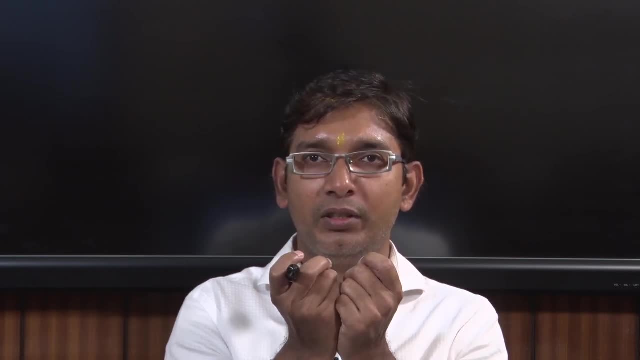 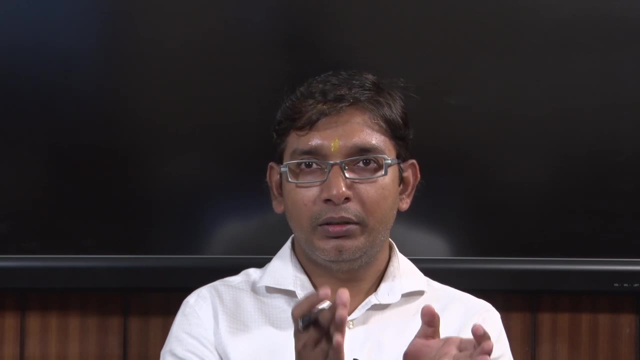 You know, measuring their surface area and then surface to volume ratio in general very difficult for a given sample right. So if you know the pressure drop, indeed we are going to obtain expression: pressure drop for the laminar flow, pressure drop for the turbulent flow. 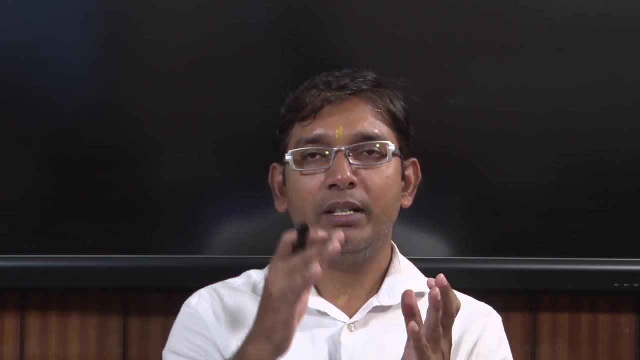 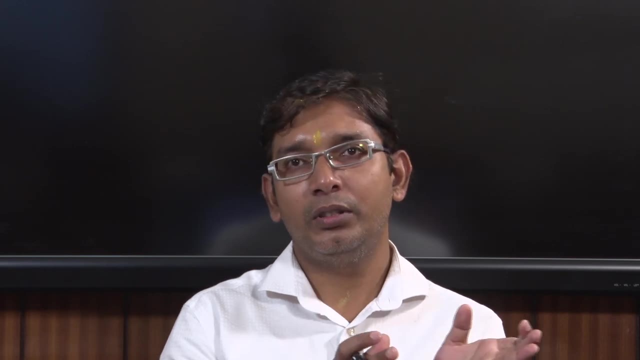 So under such conditions we have: let us say: if you know the average velocity experimentally, then you can know the Reynolds number. If you know the Reynolds number by experimentally, then you can know the pressure drop experimentally. right, You can, experimentally also you can calculate the pressure drop. 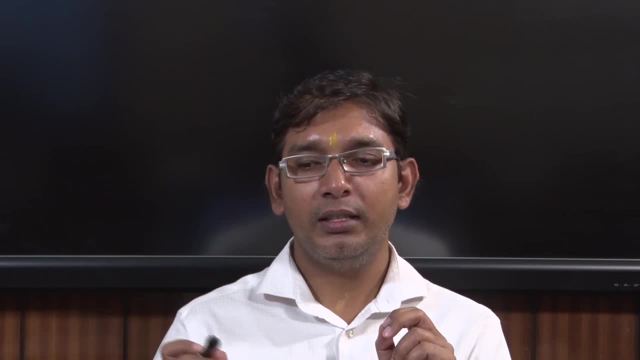 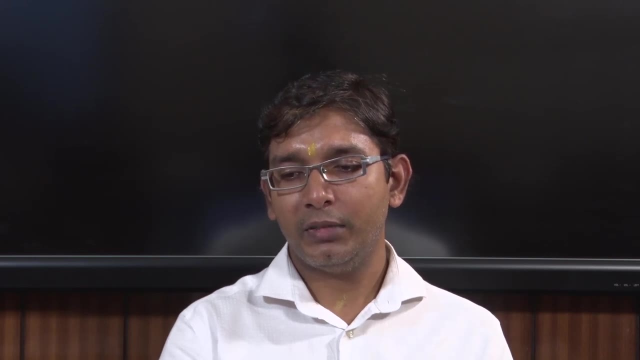 So the corresponding to that pressure drop, what is the velocity, etc. you can calculate and then you can use the equation that we are going to apply here. So then, what we understand? We find the pressure drop, We find out something like 6 by pi, s, dp. these kind of expressions are there in our equation. 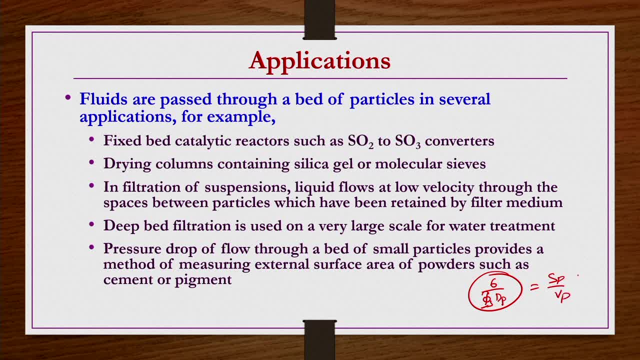 So, which is nothing but Sp by Vp. So this Sp by Vp, finding Sp by Vp, is very difficult, especially for very small particles. in general That has to be generally done by, you know, microscopics, but you cannot use microscopic analysis for large number of particles. 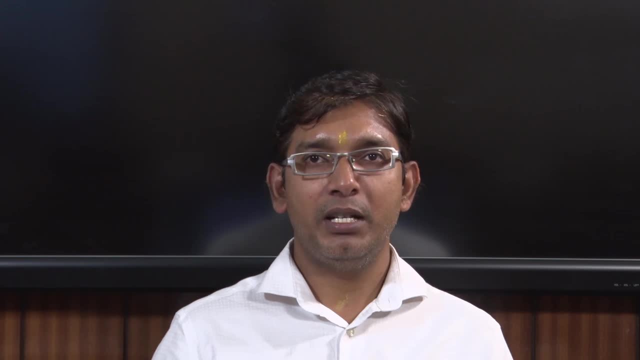 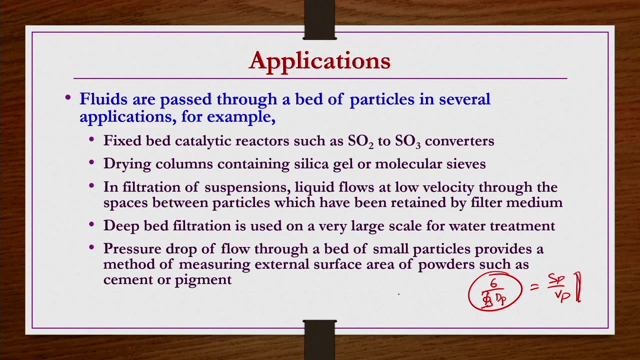 And then also microscopically, if you see, there are different dimensions, like you know, farad dimensions, There are different Stokes dimensions, etc. we have seen, Let us say, the fine particle, if you see in the microscope, if you taking having this kind of shape, let us say right. 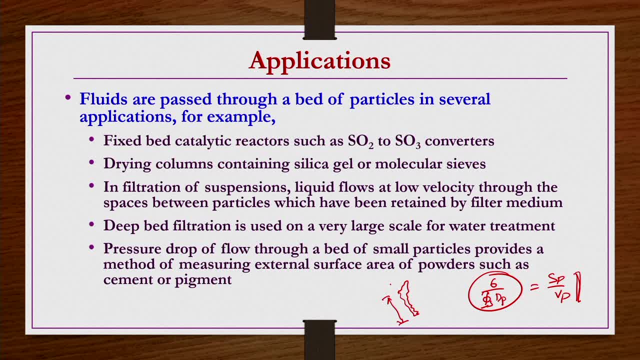 So which dimension should you take? Should you take this dimension, Should you take this dimension or should you take this cross-sectional dimension? Which one should you take? This all we have seen, like you know, in one of the previous lecture of first module. 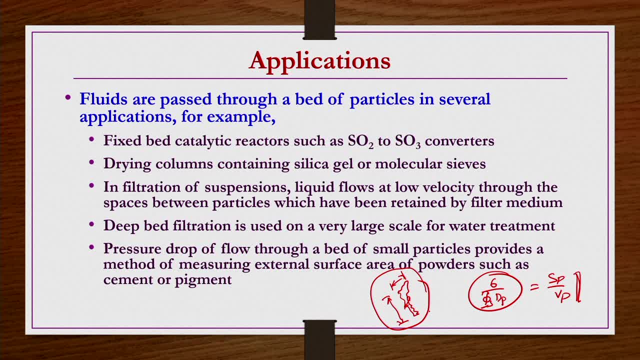 So because of these reasons, you know, finding out this Sp by Vp ratio in general very difficult. So what we are going to do, We are going to take this Sp by Vp. We are going to take this Sp by Vp. It is very difficult for the very fine and then irregular particles. 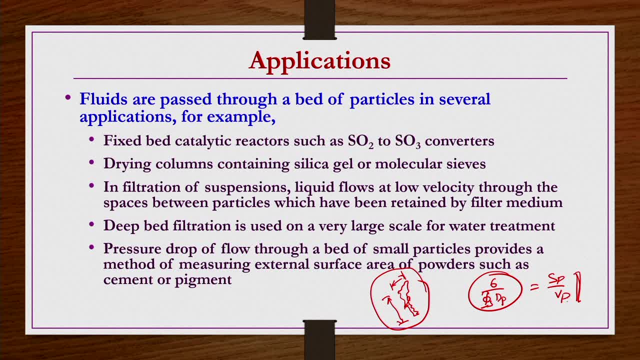 So for that you know what you can do. We can find that overall Sp by Vp from this pressure drop calculations. What we can do, We can take this particle in a kind of a column, as a kind of packing material, like this right. 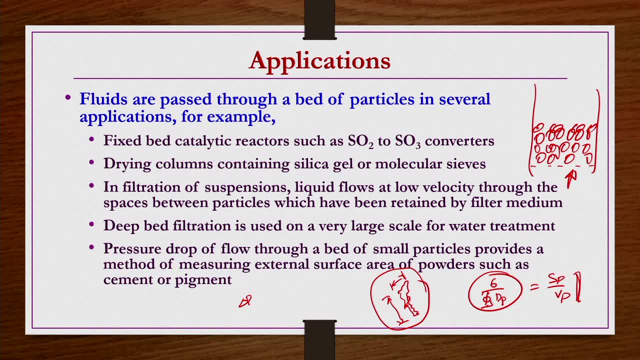 And then you allow some fluid to flow, non-reacting, non-corrosive fluid to flow through this particles. Okay, Thank you, Thank you, Thank you. So we are going to take this Sp by Vp which is forming the bed. 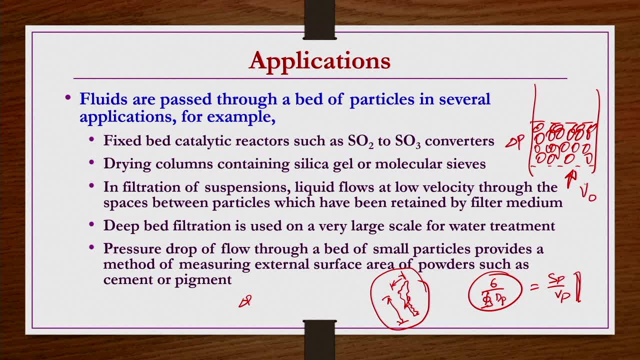 And then for this bed, for this velocity V, naught bar, you know, you calculate, you know what is the pressure drop experimentally, right? So now, theoretically, we are going to develop delta P by L or minus delta P by L, expression for packed bed, right? 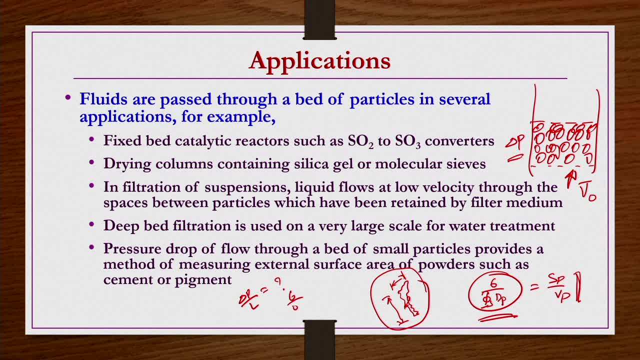 So it is having some terms, like you know: 6 by pi, s, dp, something like that we are going to derive, Okay. Okay, So now you calculate experimentally: rest. everything in the right hand side is in general known, like you know, velocity of the fluid, void, age and then density of the fluid viscosity. 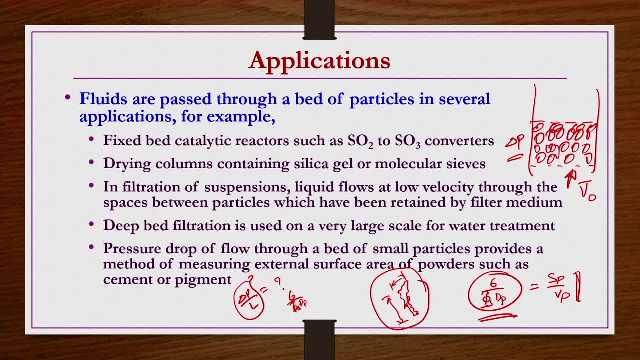 of the fluid, size of the particle used for the packing, etc. Those things are known, right? So, size of the particle, if you assume that it is not known from theoretical point of view, So then experimentally, whatever delta P that you get, that you use, and then only in the 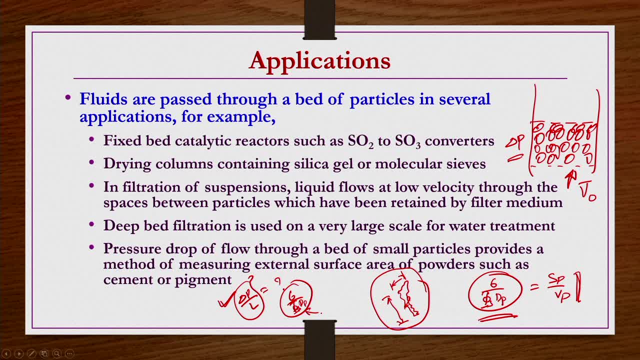 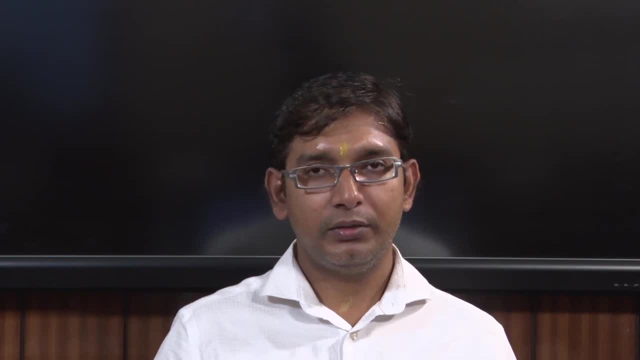 right hand side, you may not be knowing. 6 by pi s dp, So rest everything is known. so then, 6 by pi s dp, you can calculate which is nothing but sp by Vp for a given irregular particles. So this is how you know we can measure the surface, external surface area of powders. 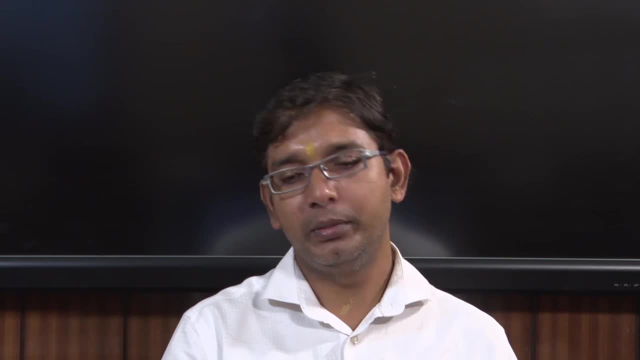 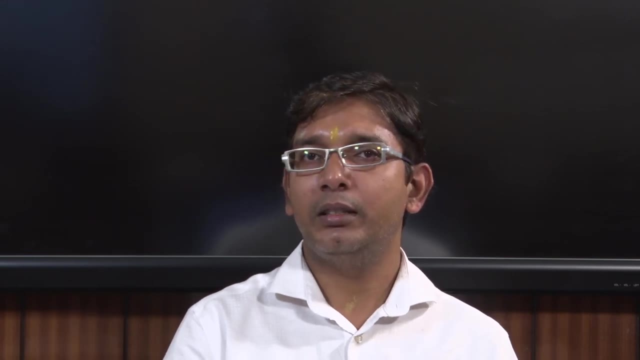 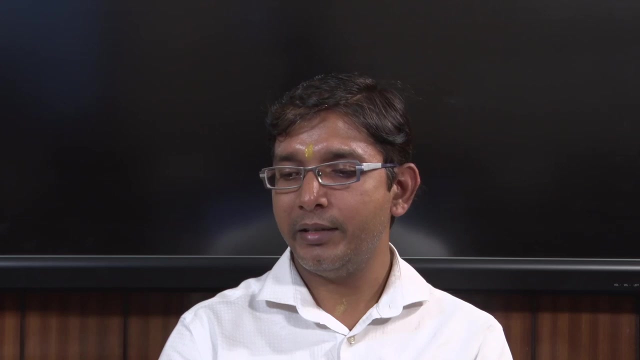 of such small size irregular particles like cement and pigment by using this flow through packed bed experiments. So that is also possible. Indeed, this we have seen as a kind of one kind of application in one of the earlier lectures. So this 6 by pi, s dp is equals to sp by vp. from where are we getting? We are getting. 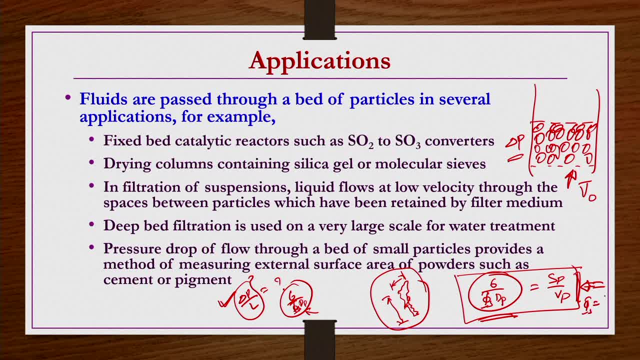 from the definition of pi s. pi s is 6 by dp divided by sp by vp. So 6 by dp is nothing but surface to volume ratio. for a spherical particle of equivalent diameter, sp is the surface area of the regular particle, vp is the volume of the regular particle. So from: 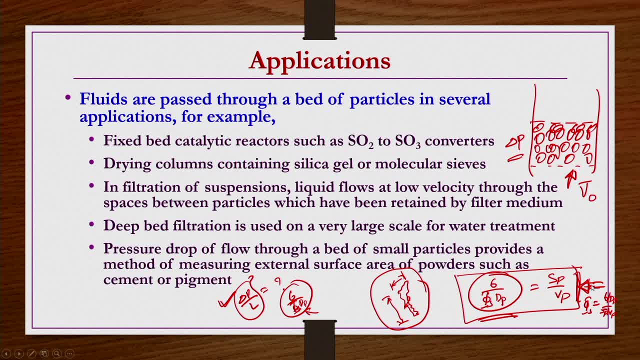 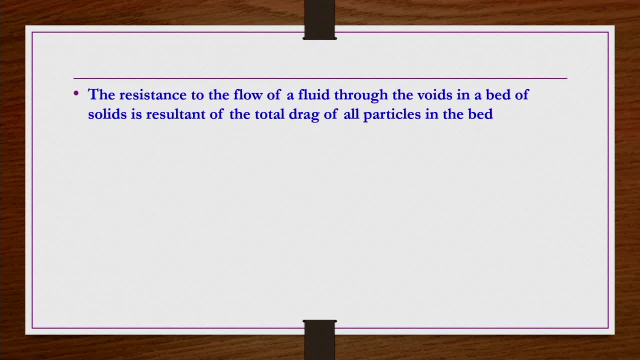 where it from that definition it is coming. this also we have seen, and then we have done several problems also on these things. So now what we understand: the resistance to the flow of fluid through the voids in a bed of solids is resultant of the total drag of all particles in the bed, or the total 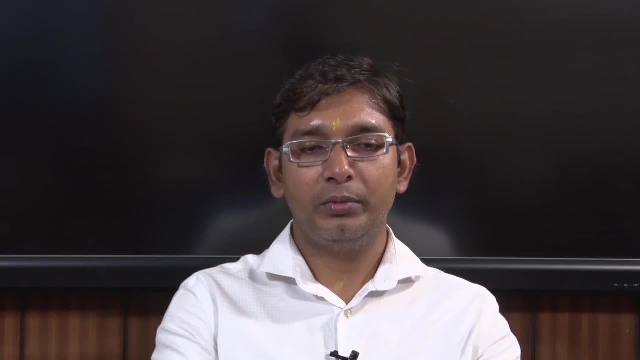 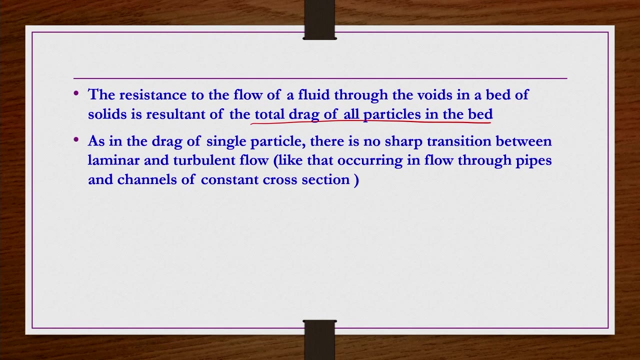 resistance offered by all the particles. So that is going to be the overall resistance to the flow of fluid. So, but you know, as in the drag of single particle, you know, there is a sharp transition between laminar and turbulent flow in general. 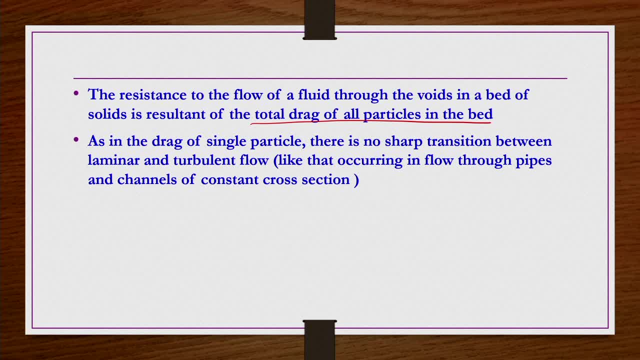 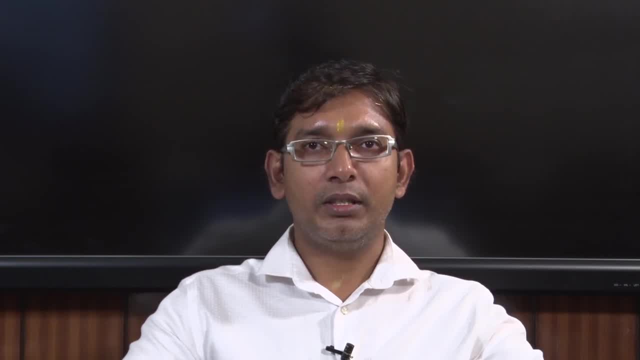 In our single particle cases we have seen, like you know, if the Reynolds number is less than 0.1 or less than 1, we say that it is a kind of Stokes regime, or if it is a kind of a case flow through pipes, then we know that you know Rep or the Re for a kind of 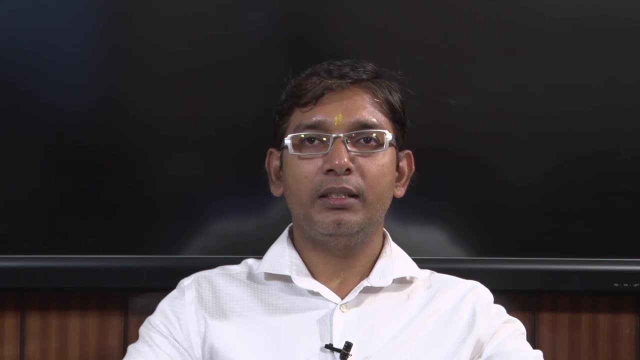 pipe flow case. if it is less than 2100, we can say that it is a kind of laminar flow. if it is more than 2100, we can say it is a kind of turbulent flow. Such kind of sharp transitions in general are not possible in the case of a flow through packed events. 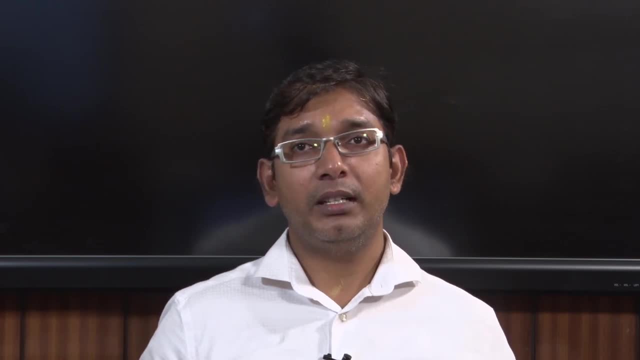 In general. indeed we know that from expriment tiene. so far it has been found that the flow through beds of particles is laminar only for small ranges. let us say up to Rep of 5 to 10 only. If it is more than 10, it is not going to be under laminar flow conditions. 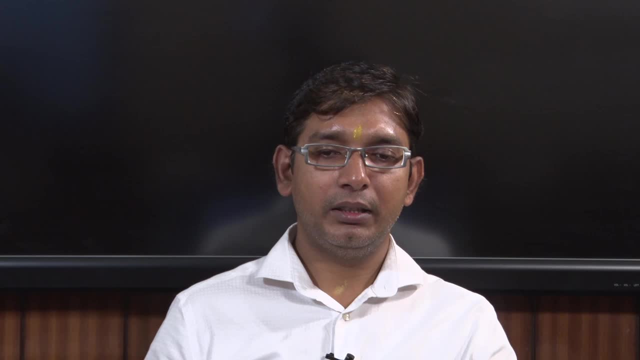 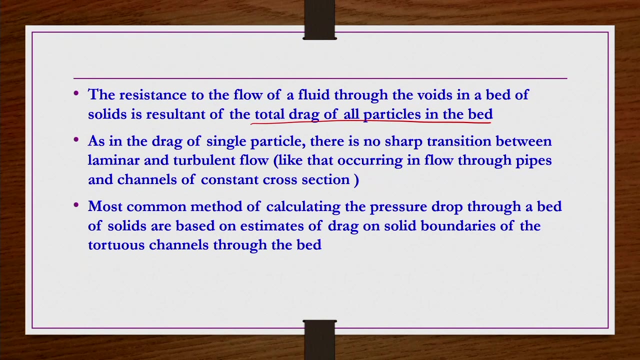 anyway right. So such kind of sharp transitions are not possible in the case of flow through packed beds. case of packed bed. Thus most common method of calculating the pressure drop through a bed of solids are based on the estimates of drag on solid boundaries of the tortuous channels. 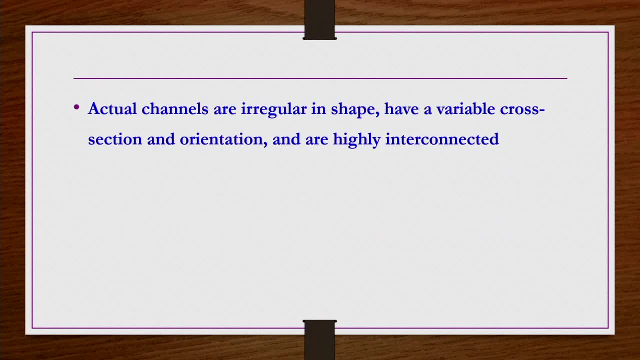 through the bed. So actual channels in general are irregular in shape- okay, We have a variable cross section and orientation and are highly interconnected. porous structure in packed bed in general like this. So these particles are in general not necessarily spherical, They can be kind of needle like they can be crushed particles. irregular shaped particles. 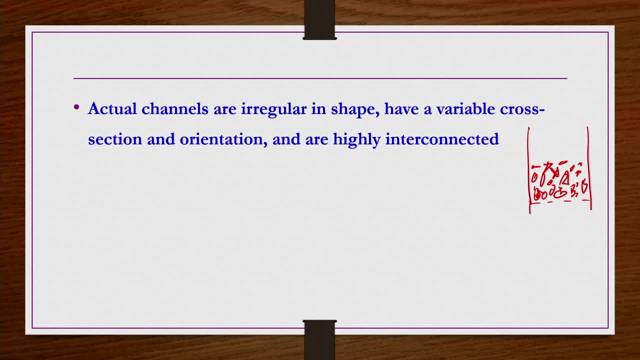 they can be like anything, right. So because of that one, actual channels in general they are irregular shaped. So this flow channel, flow channel in the sense, whatever the flow channel, is, free area, free volume area that is available between the particles right. 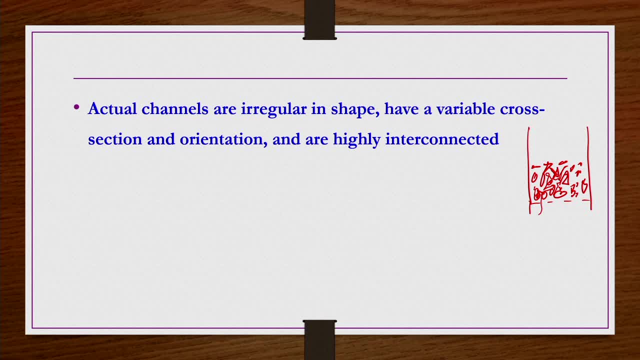 So that is very irregular, okay. And then we have a variable cross section. If it is a flow through a column, so then the cross section is a constant from the inlet to the outlet of the column through which the fluid is flowing. But if that column is packed with, 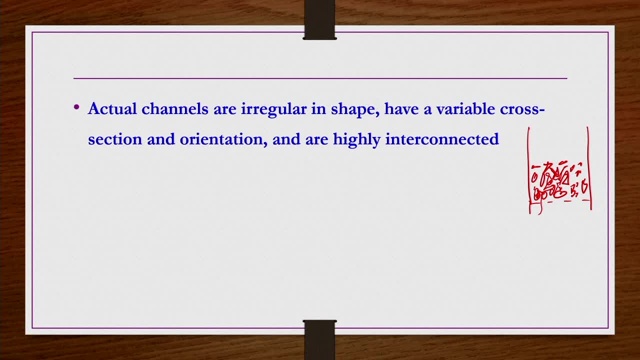 some kind of packing material. so then, what we have- We have a kind of cross section- is varying. So here the cross section is different, here the cross section is different, here the cross section is different From one location to other location. cross section in the sense, cross section of the. 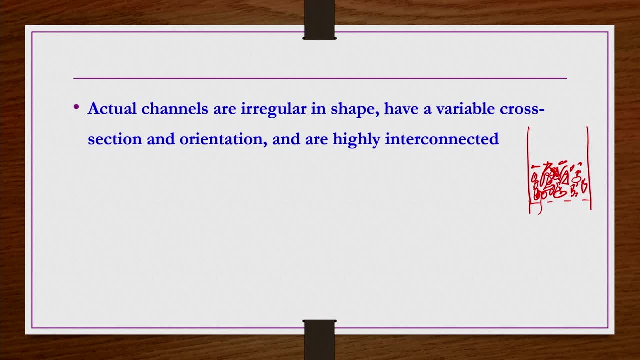 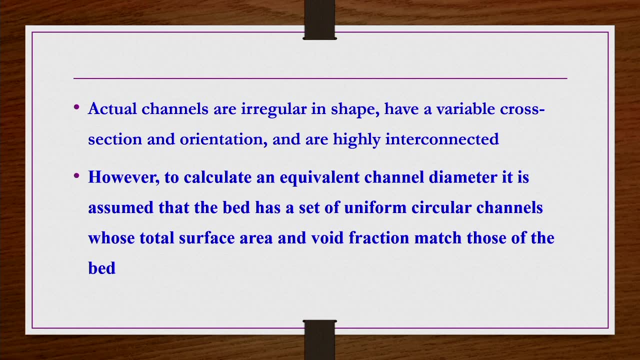 flow channel which is available for the fluid to flow, And these channels are also highly interconnected in general. okay. So, however, we have to calculate the pressure drop. So how to calculate pressure drop? Calculate an equivalent channel diameter. It is assumed that the bed has a set of uniform circular channels whose total surface area and void 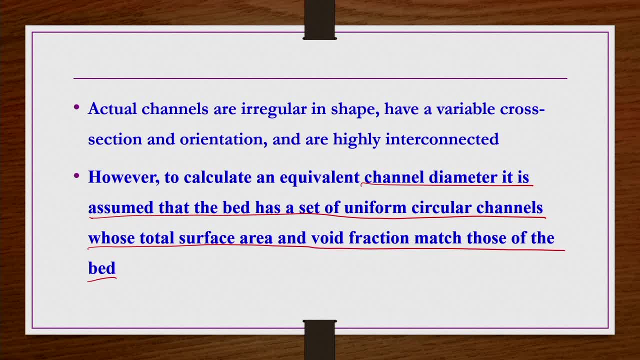 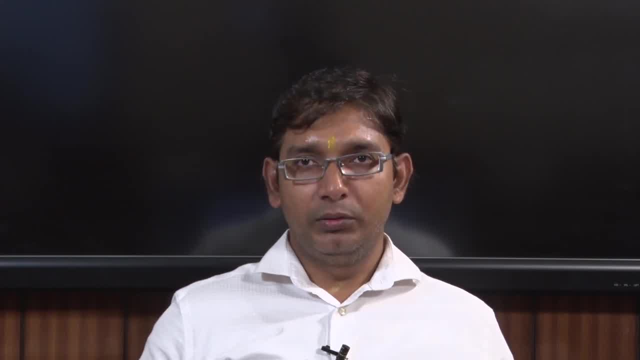 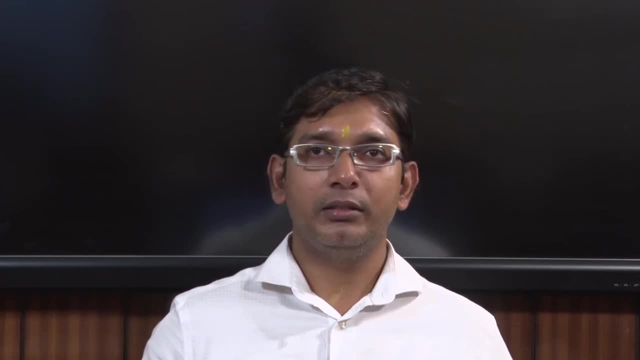 fraction match those of the bed. Okay, So now actually this: why are we doing this flow through packed beds in general, Though we have seen there are a kind of catalytic reactions, there is a kind of heat recovery kind of system. there is a kind of mass transfer in something like drying, etc. So then what? 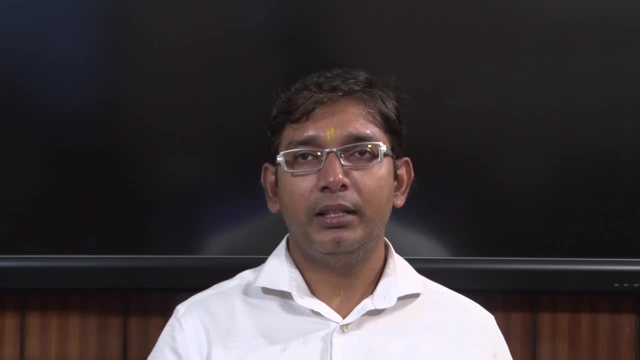 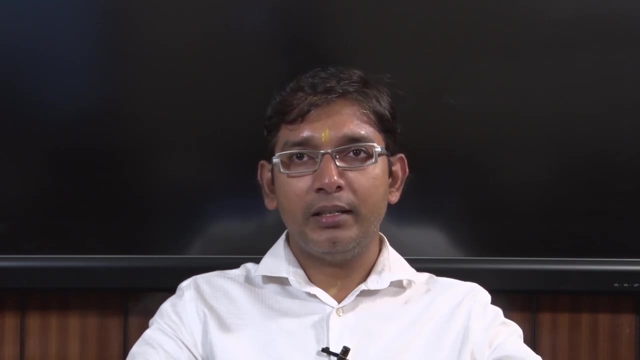 is the point. Why are we using these things in a kind of packed bed? Why not we doing in a kind of single column or individual columns, like that? That is because, you know, when we have this packing, the surface, the surface, the material, the material, the material. 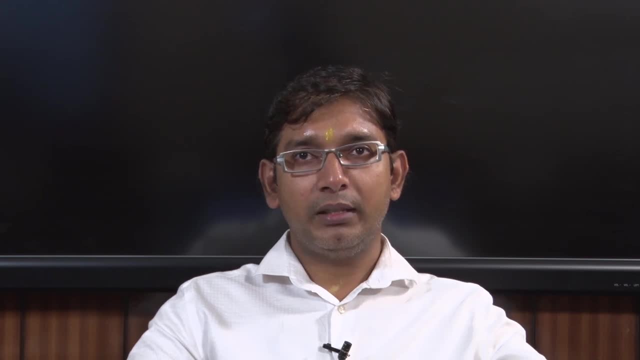 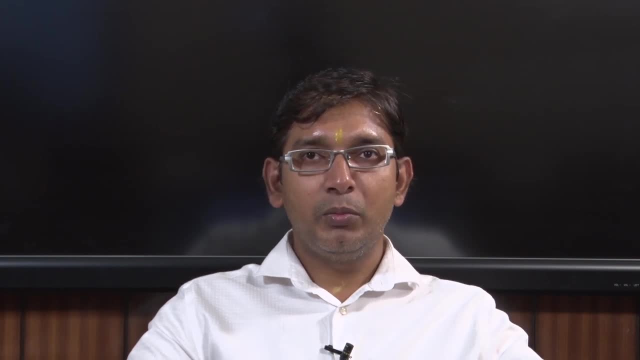 very much higher compared to the single columns. So that is the more surface area you have for this transport process to occur, or the mixing kind of operations to occur, or whatever the momentum, heat or mass transfer or reaction is taking place. that, that is degree of performance. 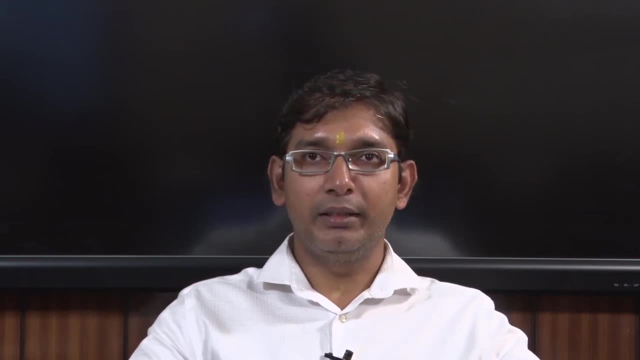 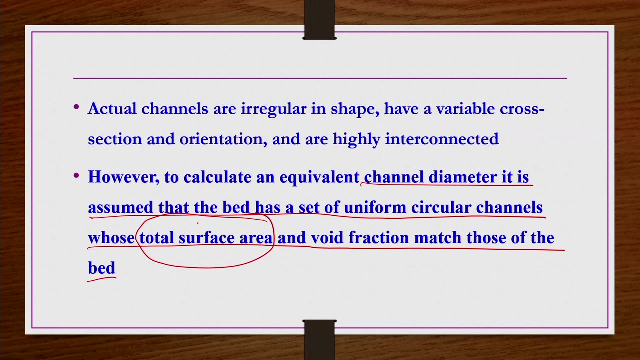 should be higher because of this higher surface area provided because of this packing. that is the reason we are doing Okay. So now what we understand? this total surface area is the one, you know, very important one, and then because of this thing, this packing, 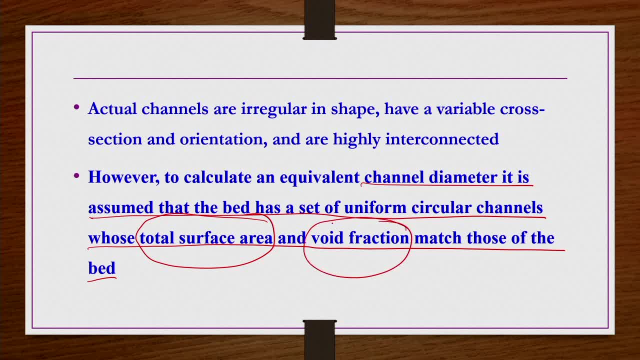 etc. what we have within the voidage or which in the column. we have a kind of void fraction. So these two are going to have a kind of important role, along with the particle diameter, along with the density, viscosity of the fluid and then height of the packing, in measuring this. 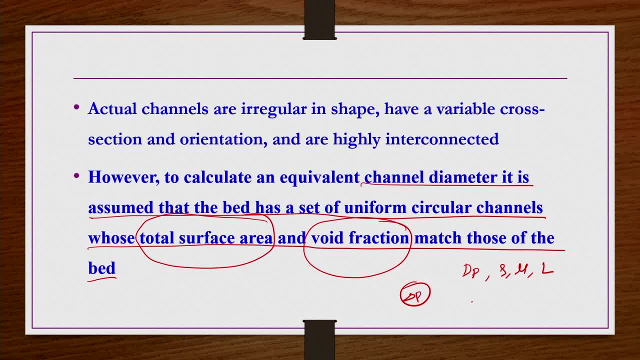 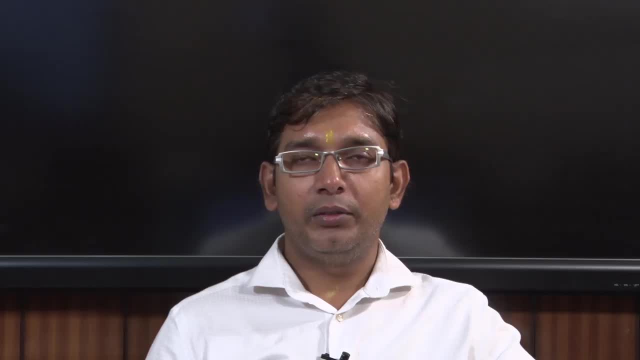 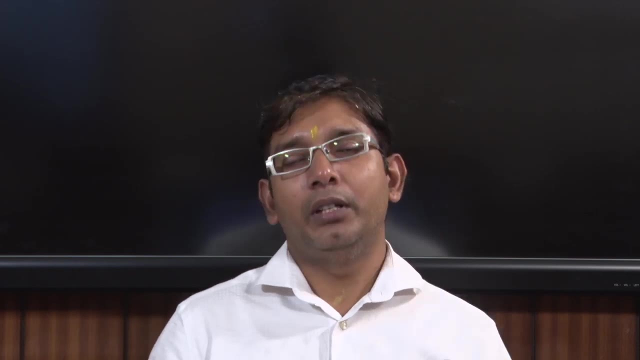 delta P. So these are the kind of things you know are playing role here. if you want to find out this dp, So, but theoretically it is very much difficult. like we know, the flow is very irregular and indeed very complex from one channel to the other channel or from. 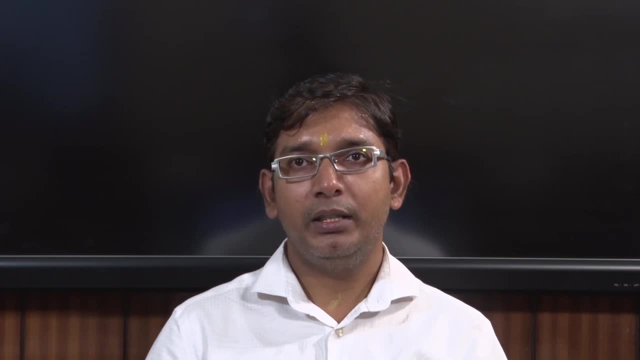 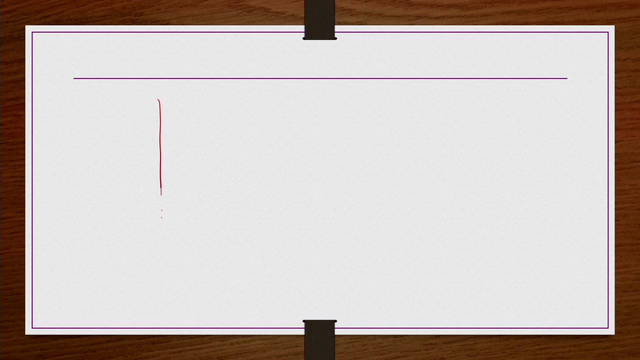 one location to the other location within the packed bed because of the irregular flow of the channels, variable cross section orientation and then highly interconnected channels etc. present in the packed beds. So then, how to do this one? So now what we do? We assume this bed, whatever is there. you. 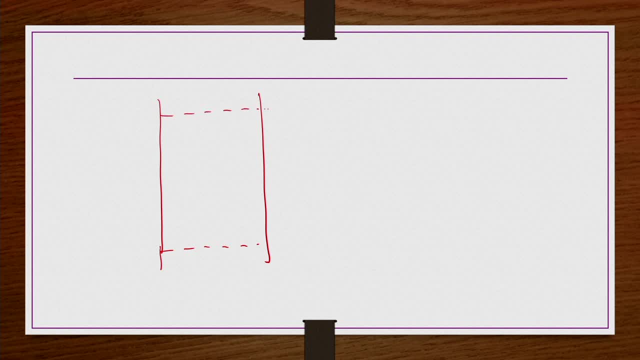 know, simplify rather than assuming simplifying. you know this is the bed packing. let us assume I am just making a kind of circles kind of thing, So do not do that, Okay. Okay, Take it granted for a kind of only spherical particles The analysis that we are going. 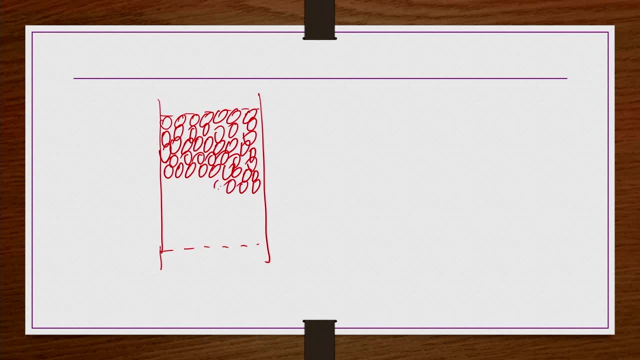 to do. that is going to be valid for all the particles, all types of all shapes: irregular, irregular, irregular, small, big particles, all of them. it is valid, actually. Okay, So now what we do? We have to equally represent this packed bed in a kind of, you know, workable. 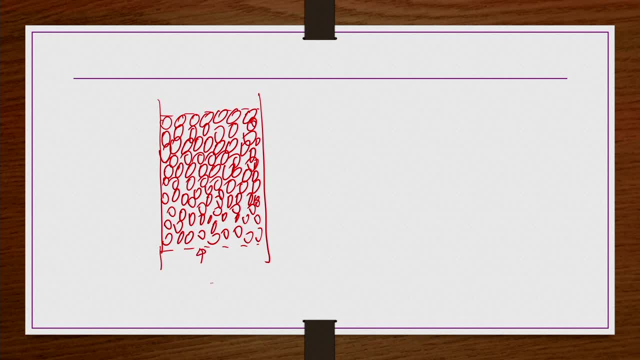 geometry, kind of things. Here, what we have, We have this, You know, epsilon, and then this channel dimension, that is, you know, variable cross section, etc. Right, So that these things are there. Right, So we have to worry about the void fraction. 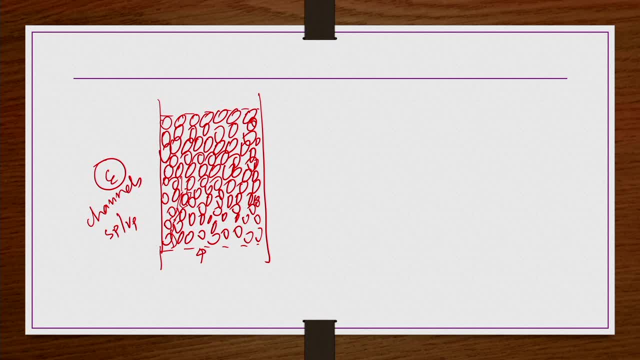 of that? is free space available for the fluid to flow? What is the free space available? That is, the interstitial spaces between the particles, That we have one parameter, and then the surface area, the other one we have to worry about, because these two are the additional. 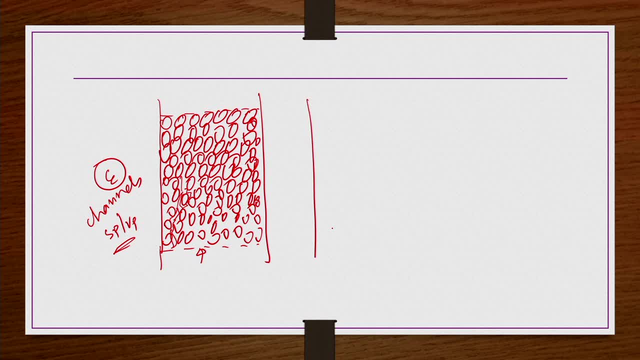 thing compared to a kind of a single column. If you have taken a kind of single column, this is packed bed, now single column, or flow through pipe, kind of things. So if you take these two cases here now, what is the difference? Only this packing is there, and because of 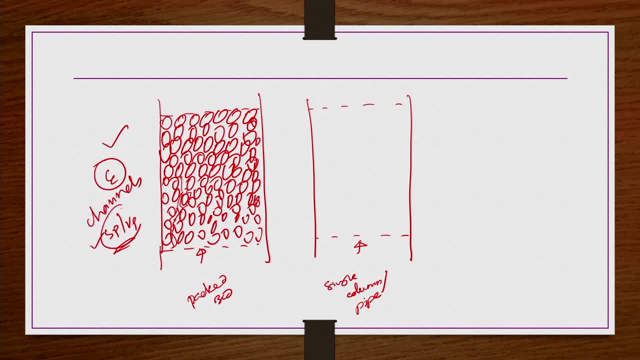 the packing, this epsilon, and then sp by vp, are the kind of things which are making a difference, newly being added up. So what we do, This system we have kind of, we will try to generalize or simplify so that we can easily do a kind of analysis and develop a kind of expression as we develop for this. 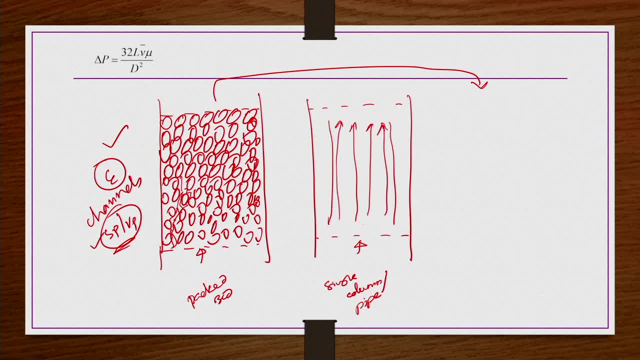 case, like you know, delta p by L is equals to 30.. Okay, 32 mu v by d square. like this is Hagen Poiseuille's equation that you know for a laminar flow through pipe. the pressure drop is this one. One can derive this one in fluid mechanics. 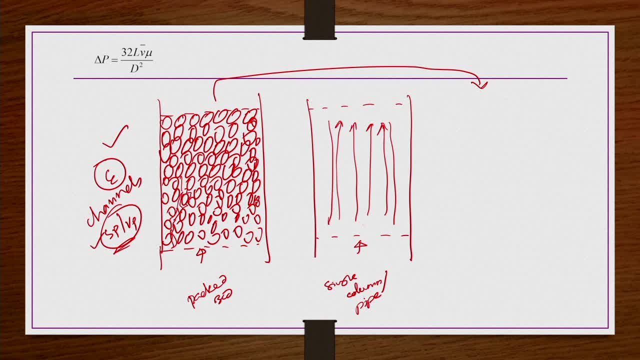 course, right. So this is the one you know. we have, like you know, for now, this column. when we are adding some packed material or material for packing, then these two things are additionally coming. So this system, we are generalizing it. How we are generalizing now or simplifying like this, We are taking a few number of 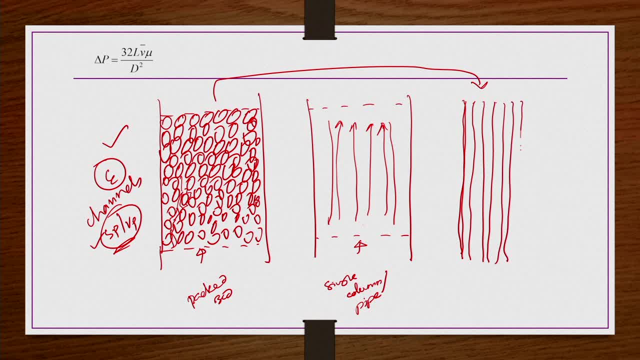 capillaries. okay, right, we have these capillaries like this through which the flow is taking place, like this: okay, The diameter of these capillaries we take like this: okay, Here we take, let us say, D capillary. The height of the capillaries is same as the height of the. 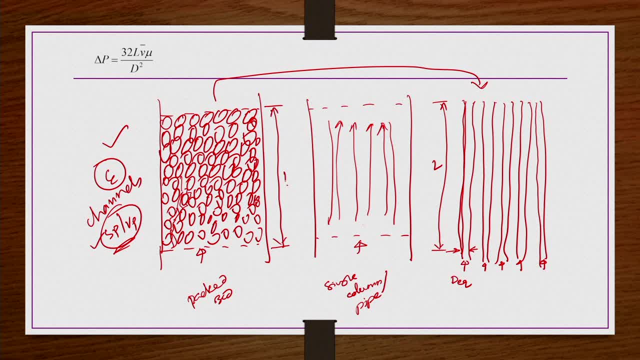 packing here. So now these N number of capillaries. so what we are saying, they are N number of capillaries. So these capillaries, what we are saying, we are bunching together, we are adding together, like we are forming, like you know, we take N number. let us say this: 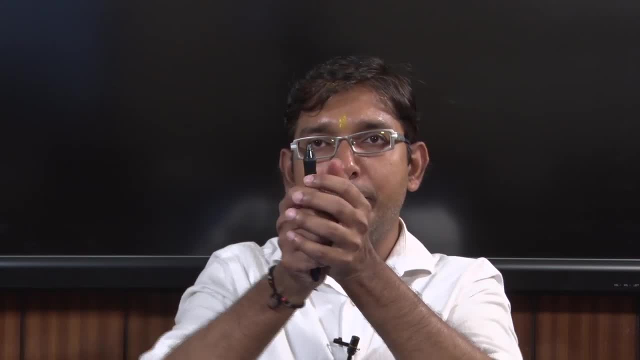 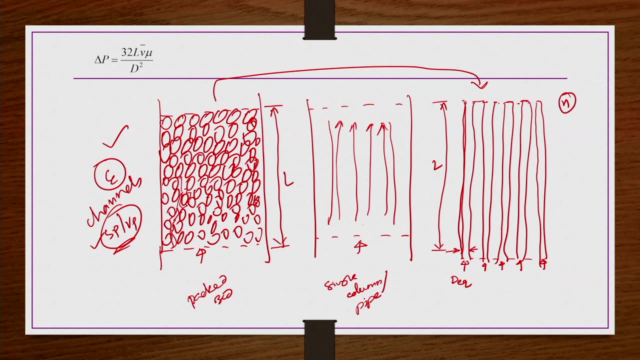 is one capillary like N number of capillaries are there. we are making a kind of bunch, kind of thing. So bunch of capillaries, so how many capillaries? we do not know. let us say N. So what we are. 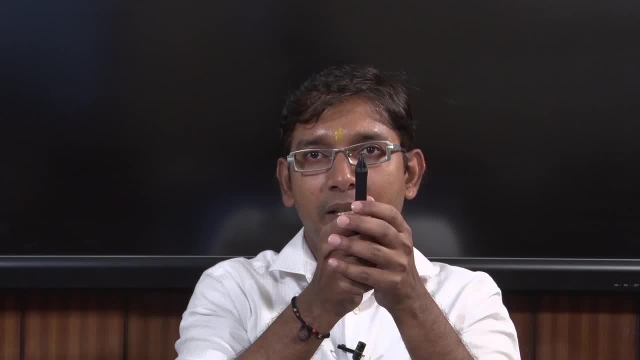 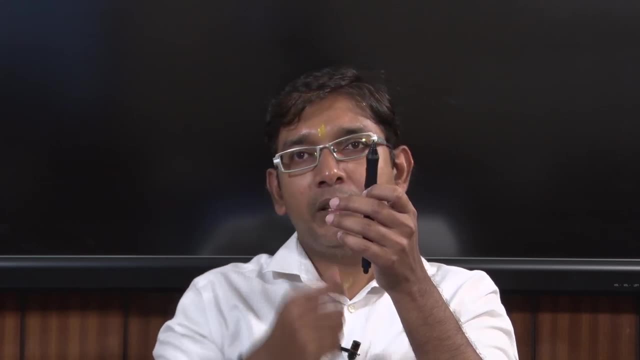 assuming that this capillaries, when you are taking N number of capillaries, whatever the void space is provided, that is the area, internal volume of the capillary through which flow it is taking place For all the capillaries. if we are together, then find out the fraction. 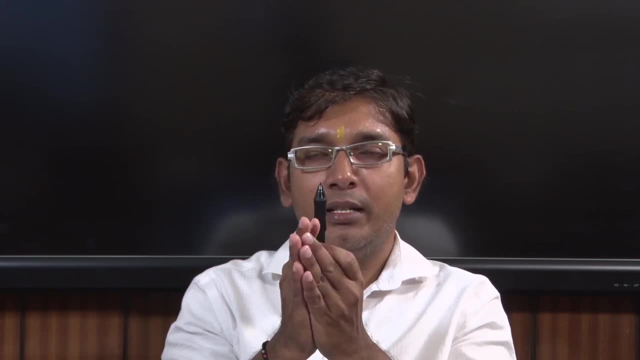 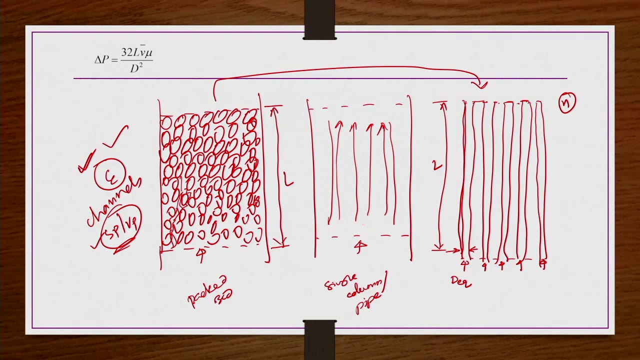 so, then, that you know space, or the space, or the void space available for this N number of capillaries is same as the void space here in the packed bed. That is how we are going to do. So: we are replacing, we are getting N number of capillaries. 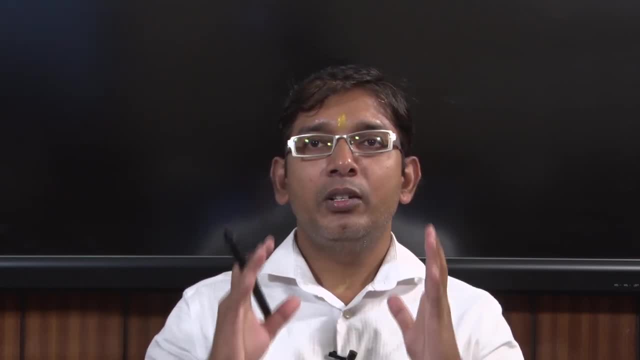 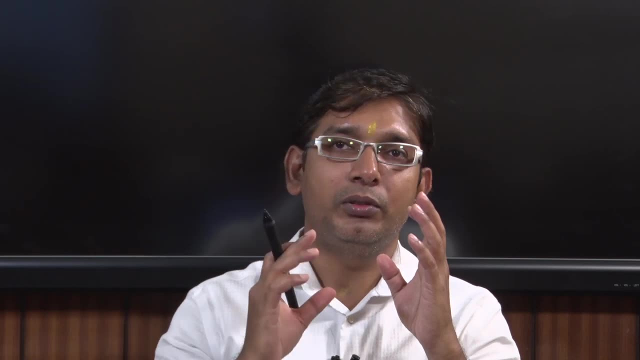 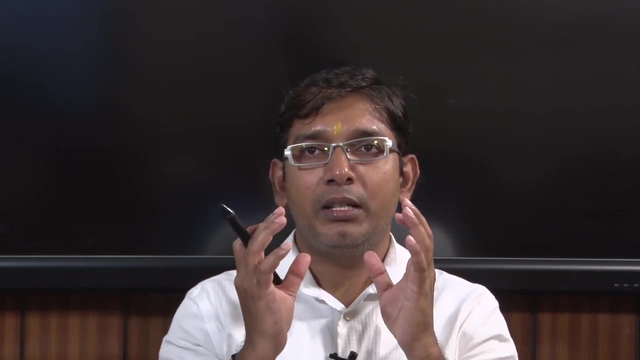 having same height as the packed bed height, right? So those N number of capillaries are forming a kind bunch of capillaries and then allowing the fluid to flow through. So then, whatever the void space that is available in this bunch of capillaries, that is equal to the void space. 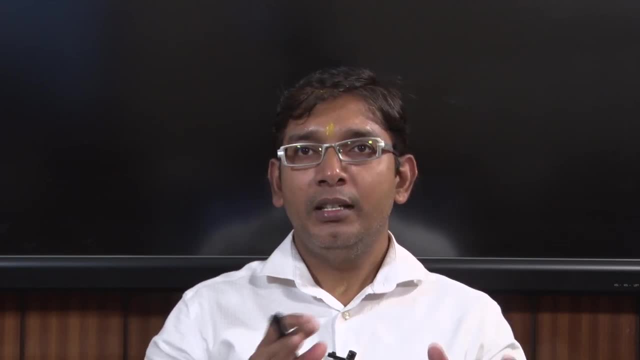 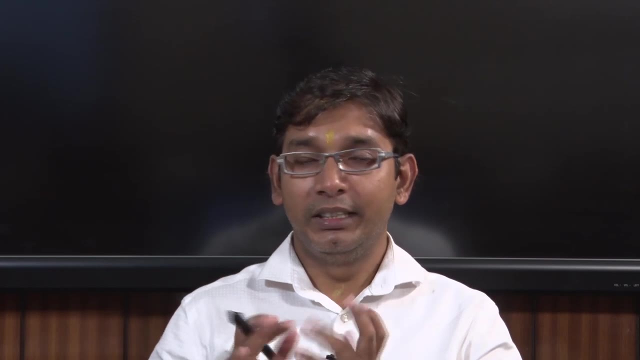 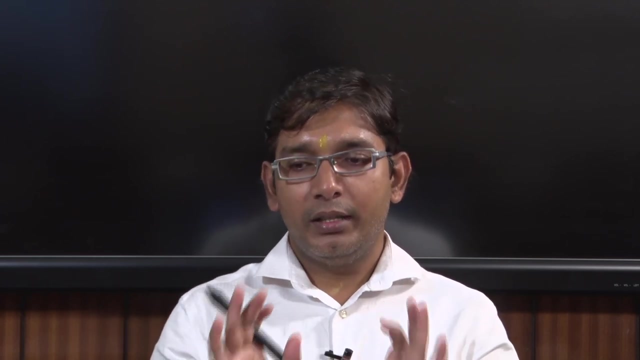 of packed bed, that epsilon that we have taken, such that n number should be decided. Should it be 10, 100, 1000? that we do not know, indeed, we do not want to know at all. So, but theoretically, this is what the one representation that we are doing, that is one. 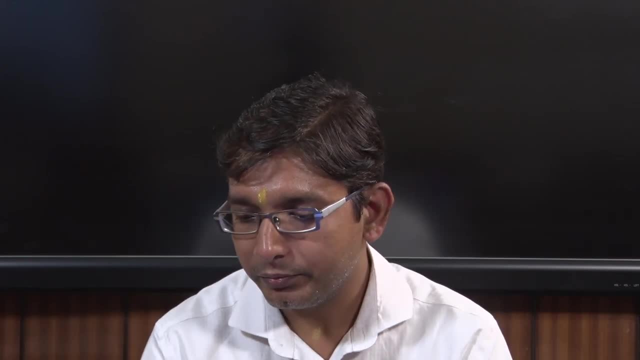 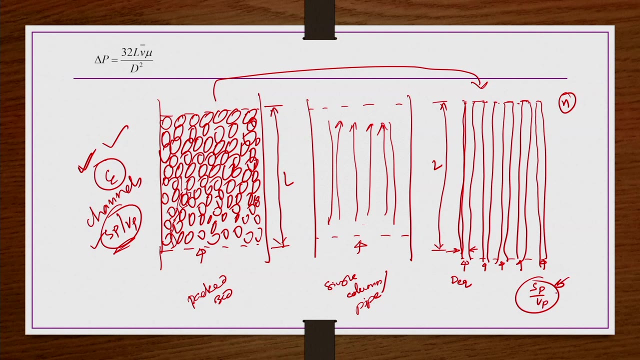 and then next one is the surface to volume ratio. Whatever the surface to volume ratio here in this n number of capillaries are there, that is same as the surface to volume ratio for the packed bed. So the n number should be decided such that for the bunch of capillaries 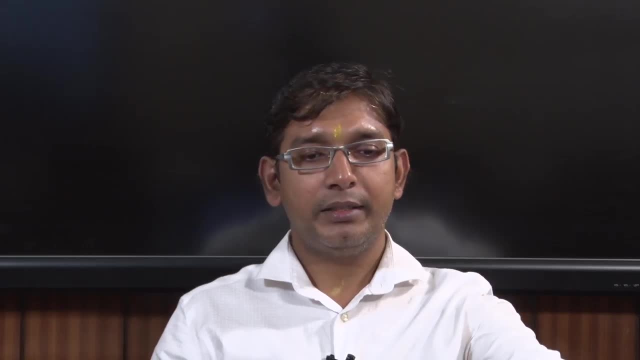 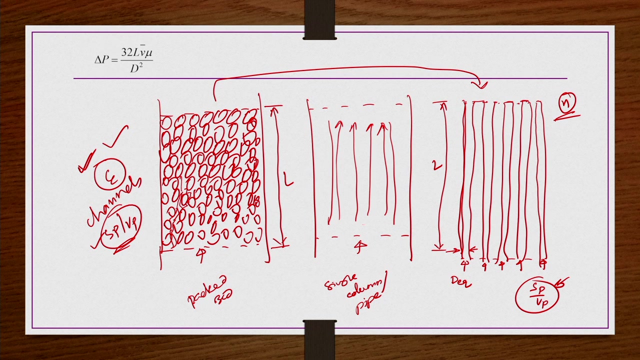 whatever the epsilon and sp by vp are there, So they are same in the case of packed bed, or they should be equally equivalent to the whatever we have, the packed bed case. So this n one has to find out. In reality. we may be thinking, but we do not need to find out. Let us assume this is n. So this we. 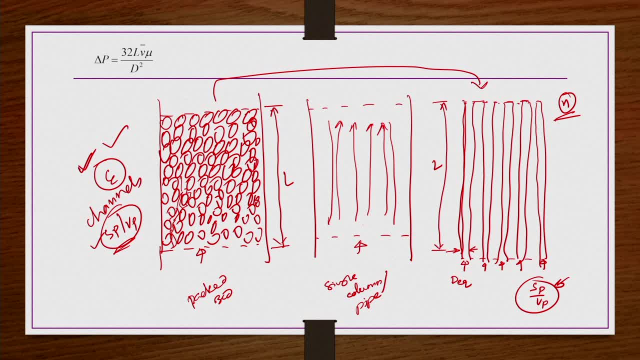 are doing. Now, here, this representation, this d equivalent is there. The diameter of the capillary is d equivalent. that is, the flow channel dimension, or the dimension which is providing The space that is through which the fluid is flowing in the capillary. Now, this d equivalent. 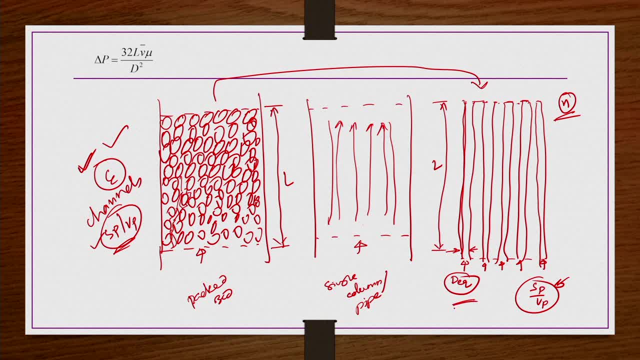 we are going to find out, as function of this epsilon packing, particle diameter etc. for a given real system. That is what we are going to do. And then here, whatever the d in Hagen-Pazels equation is, d is there, we replace d by d equivalent, and then v we replace by the superficial velocity. 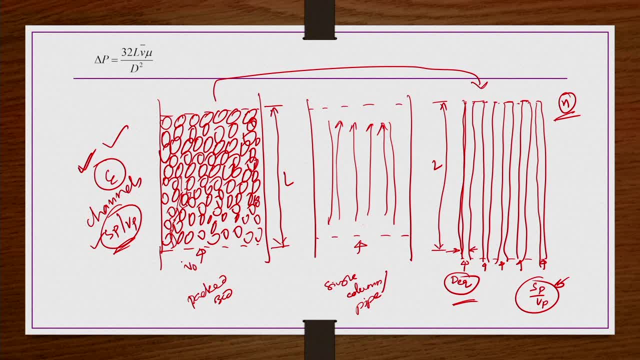 Okay, V bar. So V bar is a kind of a superficial velocity of the packed bed. superficial velocity in the sense, like you know, empty tower velocity. like you know, this column is there, this is the same column here, this second one, this column, packed bed column is there, whatever. 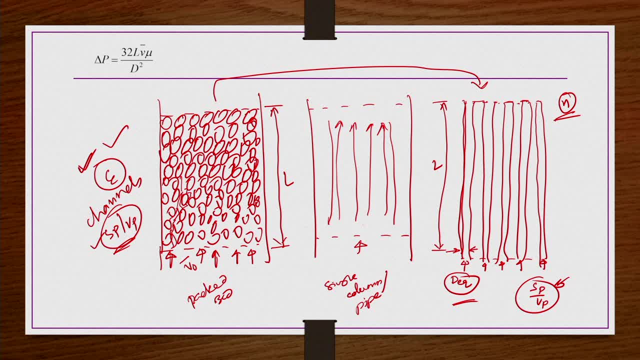 the dimensions are of this packed bed column and then dimensions of the empty column are same, Then whatever the velocity is there through the empty column under this same pressure drop as in packed bed. that is known as the superficial velocity, or simply superficial velocity is a kind of empty tower velocity when there is no packing right. 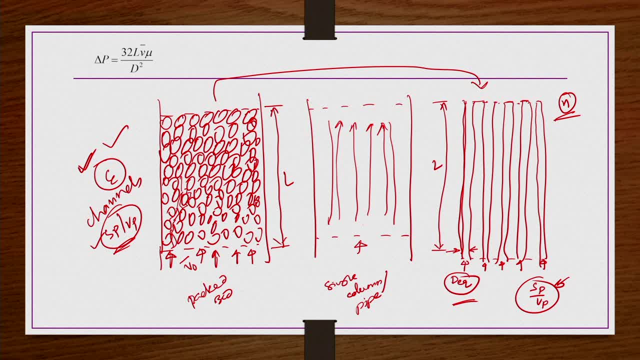 But here this V should not be, you know, kind of V naught bar, because V naught bar is a kind of velocity that is passing through as a superficial velocity, But the true velocity here you know, in the, The packed bed, the average velocity of the fluid element when it is passing through from 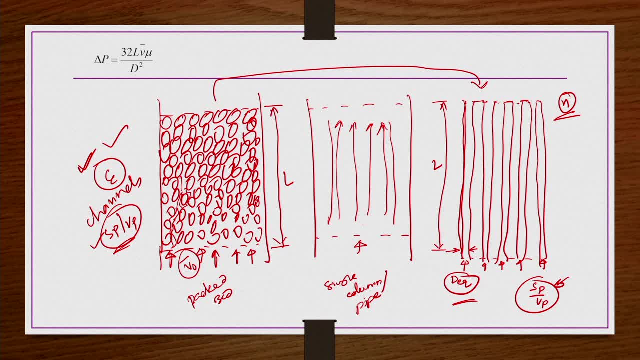 inlet to the outlet. it may be having some average velocity. that average velocity, V average, should be taken here. right. But we understand this: V average is nothing but V naught bar by epsilon here. So those things we substitute here and then simplify this. 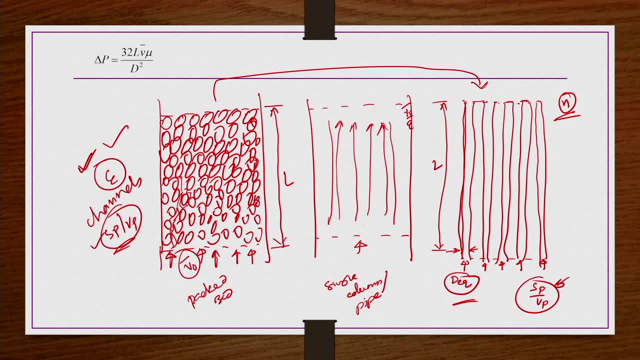 equation so that we get the pressure drop equation for this n number of you know capillaries, which is same as pressure drop for this packed bed. Why it is same for this packed bed? Because this bunch of n number of capillary, whatever the characteristics are there, that is their epsilon and their Sp by Vp. they are same. 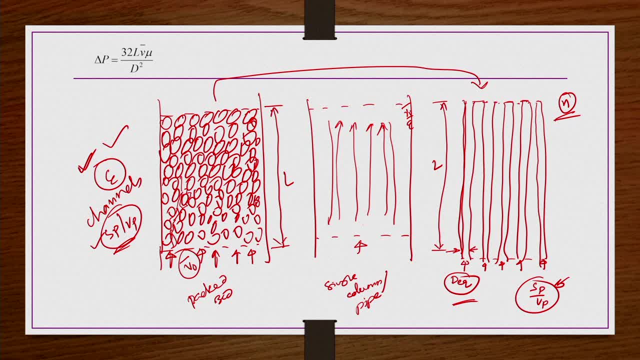 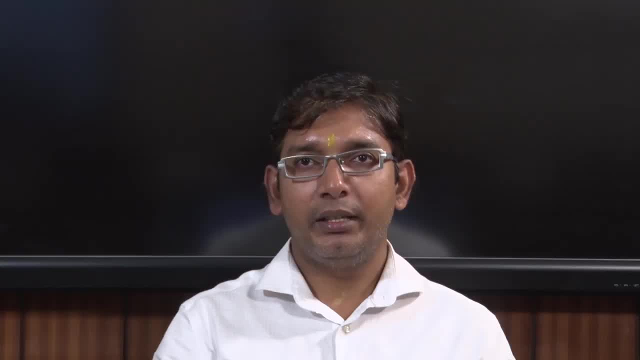 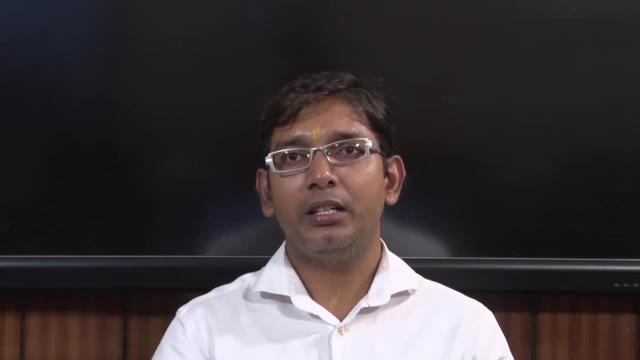 as this packed beds. That is the reason they will be same right. So since these capillaries also kind of circular tubes, something very fine, small diameter tubes kind of thing, So here also Eigen, Poiseuille equations are valid. Indeed, for those capillaries, only this Eigen. 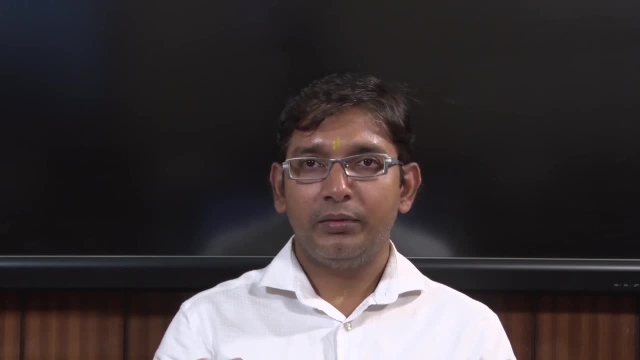 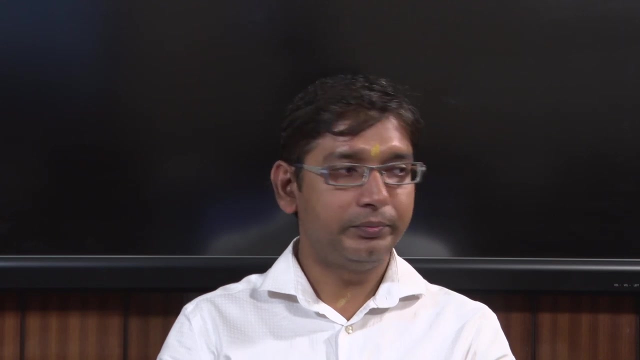 Poiseuille equation is more reliable. 1- Because of you know, laminar flow conditions can be established in capillaries much easily, right? So this is what we are going to do now for you know, developing this expression for the pressure drop. 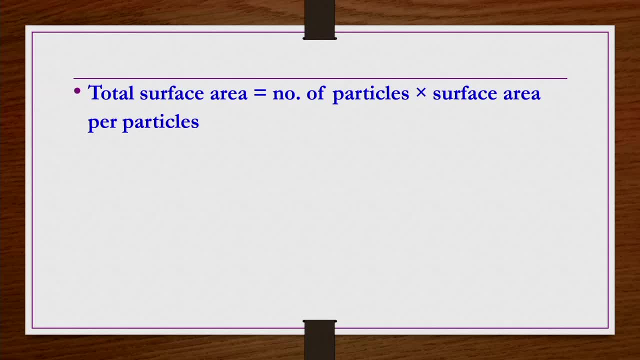 So total surface area of the bed should be surface area per particle multiplied by total number of particles. that we should do Then it is made convenient to base the calculation on the volume fraction of particles in the bed and the surface volume ratio for the particles. 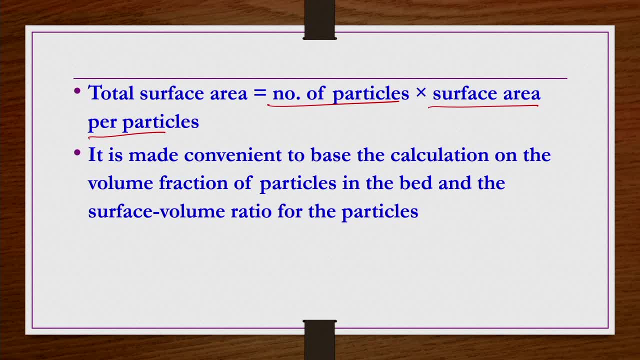 why? because if you take surface volume ratio particles, then you can also bring in the information of sphericity. Sphericity In equations. that means you can also use those equation for regular particles. okay, So then: 1 The surface to volume ratio. we know it as 6 by dp. That is nothing but surface area. 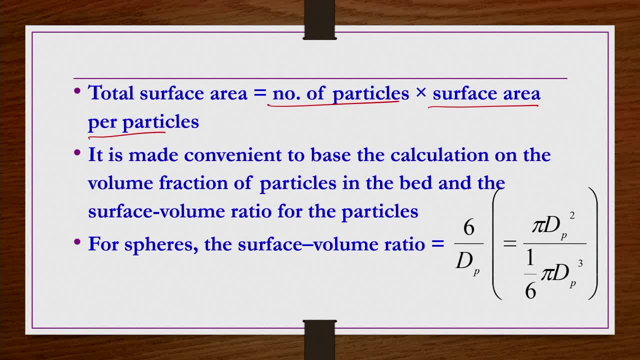 of this bed. So I have already discussed previously as the things related to the separation motion particle, that is pi Dp square divided by the volume of the spherical particles, pi Dp cube by 6, Dp is the diameter of that particle. let us say, okay, 6 by Dp. so that is from. 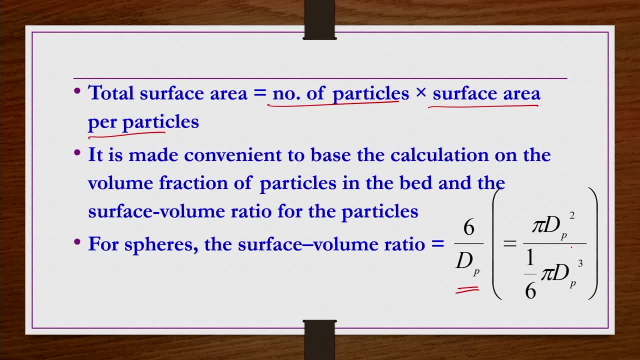 where it is coming. 6 by Dp, that is pi Dp square. that is surface area of spherical particle divided by the pi Dp cube by 6, that is the volume of the spherical particle. then you get surface to volume ratio for spherical particle as 6 by Dp. this is for the sphere. 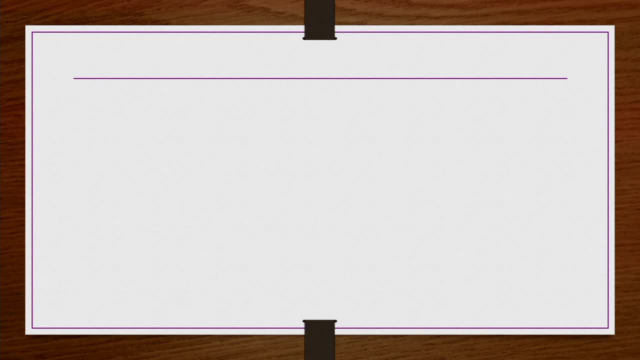 But we wanted to bring in the non-sphericity or irregular particle nature also into the consideration. so for other shapes or irregular particles, it should also include the sphericity, which is defined as surface to volume ratio, of sphere divided by the surface to volume. 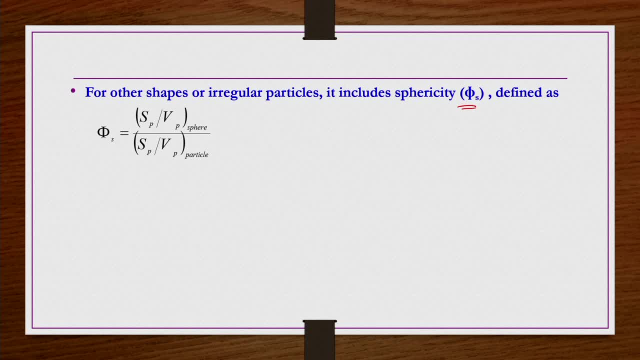 ratio of the particles, right? So then from here that we have already seen that pi S is equals to Sp by Vp, for sphere is nothing but 6 by Dp. And then for the irregular particles, surface to volume ratio, we do not know. so let us. 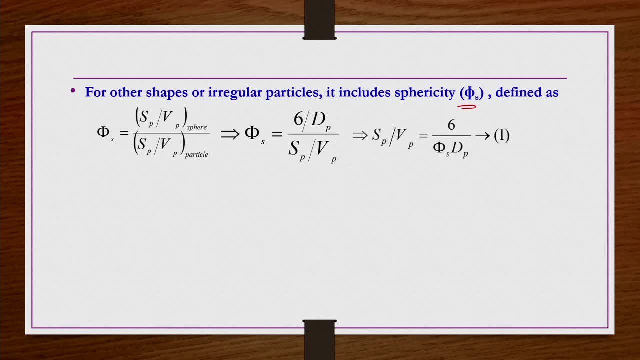 keep them as Sp by Vp. that means Sp by Vp is equals to 6 by pi S Dp. that means from somehow from your calculations that you are going to do or somehow from your results. if you can get the pi S by Dp information for unknown irregular particles, then you can indirectly 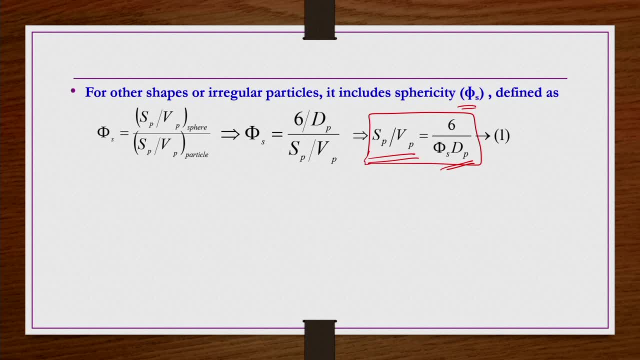 know this. So that is the Sp by Vp ratio or that 6 by pi S Dp. if you do, you will get Sp by Vp. That is not the primary object for the time being. I am giving as a kind of information because we have seen it is a kind of a application for finding out the surface to volume ratio. 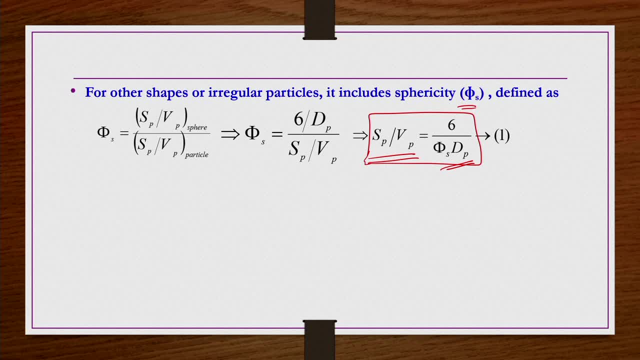 of irregular material, irregular, very fine materials. Then particle volume fraction in the bed is 1 minus epsilon. where is the epsilon? is porosity of void space, or the volume fraction of the empty space, or the volume fraction of the liquid in between the bed? 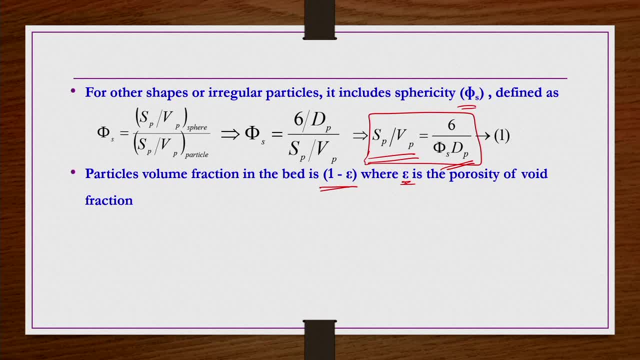 So, whatever the empty space between the particle, is that only that much space liquid can occupy. that is porosity of the void fraction. If particles are porous, then pores are generally too small to permit any significant flow through these particles. Actually, you know, when we are taking the particles, we are this analysis, we are assuming the particles. 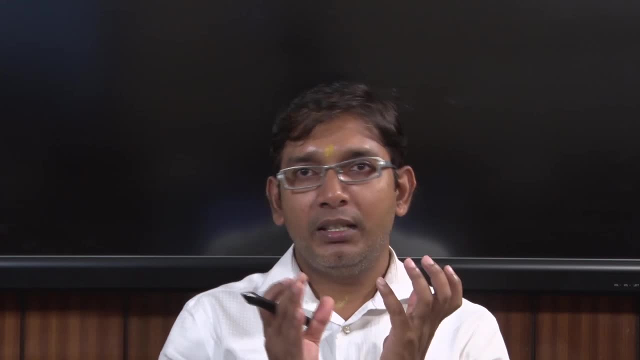 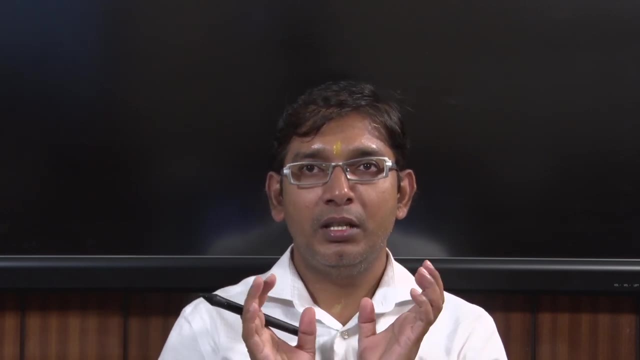 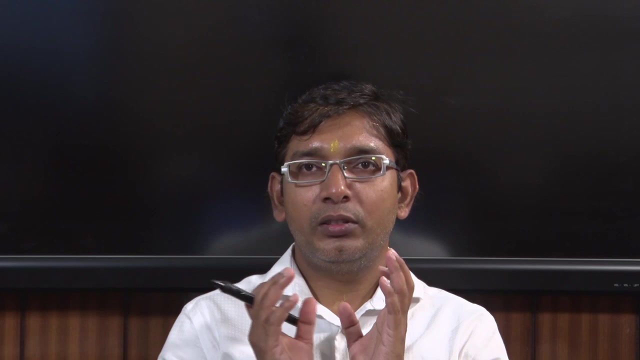 which are used for packing, Irrespective of their size and shape. we are assuming they are non-porous. The analysis that we are doing that is non-porous but however, if you, even if you have some kind of porous particle, their porous structure are too small in general to permit any significant. 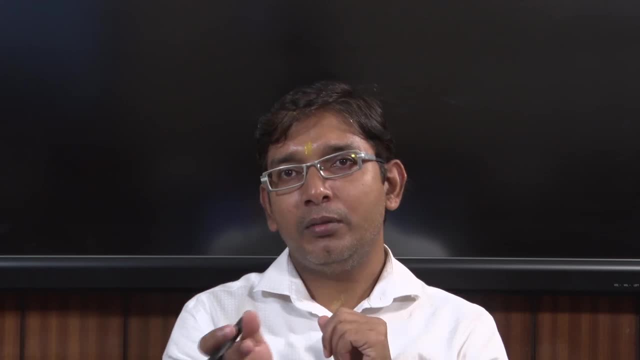 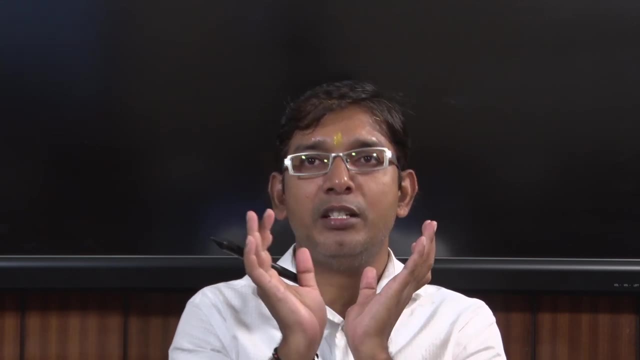 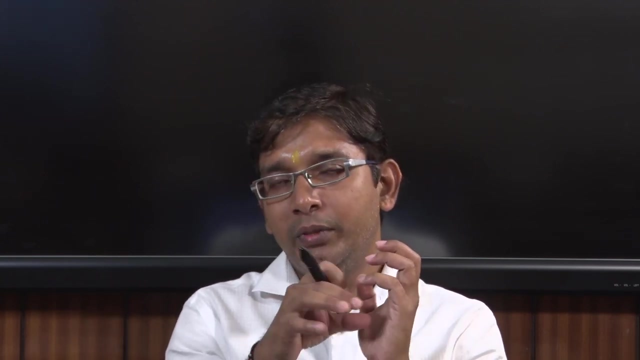 flow through this internal pores also. The porosity, whatever we are talking about, that is only for the external porosity only, or the interstitial space between the particle only. Okay, Not for the porous structure of the internal porous structure of the particle. So we are assuming indirectly that the particles are non-porous. 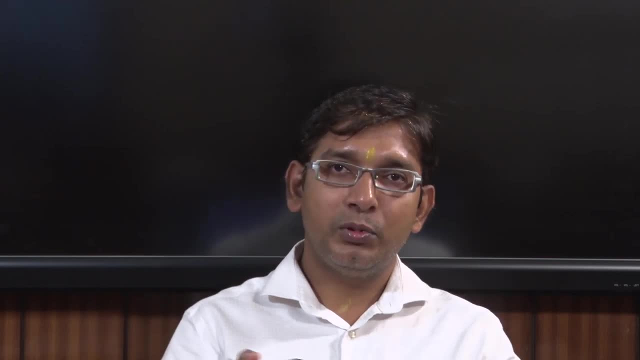 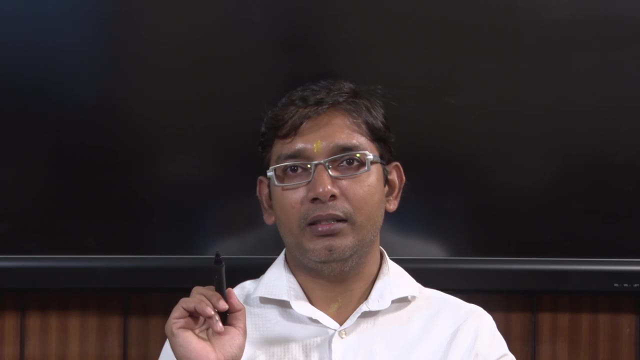 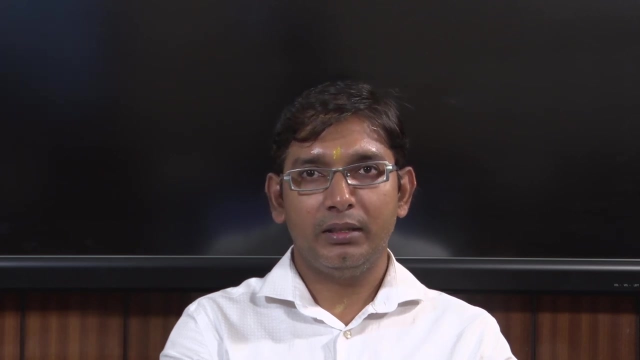 Even if they are porous, the flow that is going to take place through this internal porous is going to be much more smaller than the flow that is taking place through the interstitial spaces or external porous structure right. So that is the reason one can safely ignore the internal pore structure of the particles. 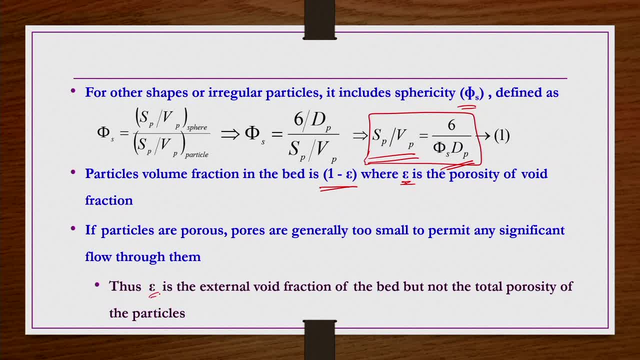 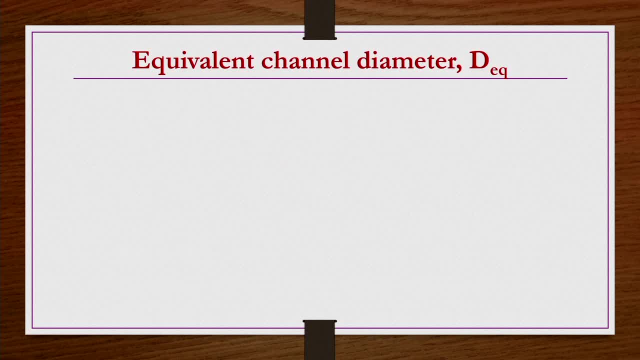 in this packed beds. So thus epsilon is the external void fraction of the bed, but not the total porosity of the particles. Now we find out equivalent diameter of the capillary channels, n, number of capillary channels that we have taken. So the diameter is d-equivalent. this d-equivalent we are going to find out as function of epsilon. 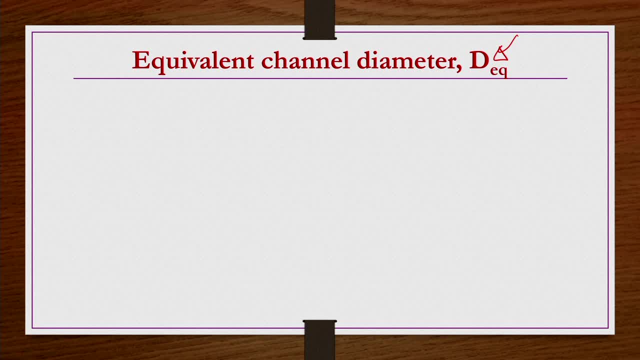 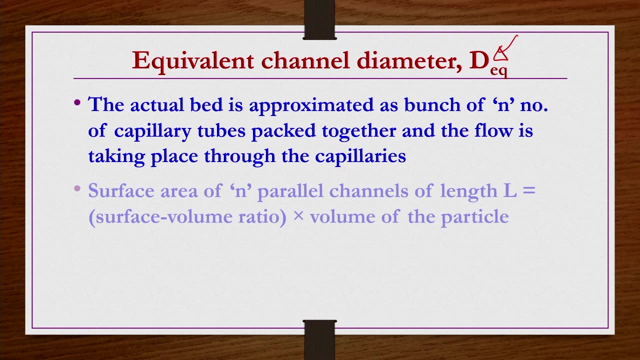 or the size of the packing material, etc. Okay, So, So the actual bed is approximated as bunch of n number of capillary tubes packed together and the flow is taking place through the capillaries. So that is what we assumed, as I explained before. 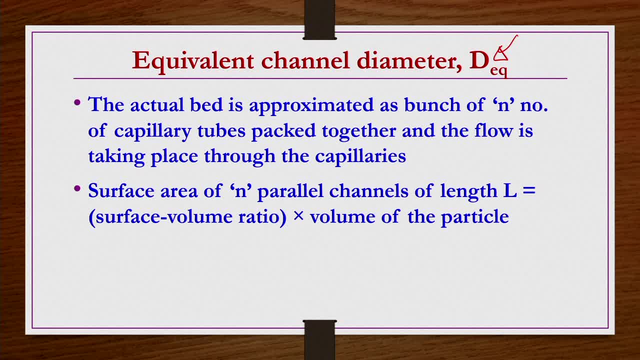 So the surface area of n parallel channels of length l should be the surface to volume ratio of particles multiplied by volume of the particle. So in real packing conditions, whatever the surface to volume ratio, is there that if you multiply by the volume of the particles, 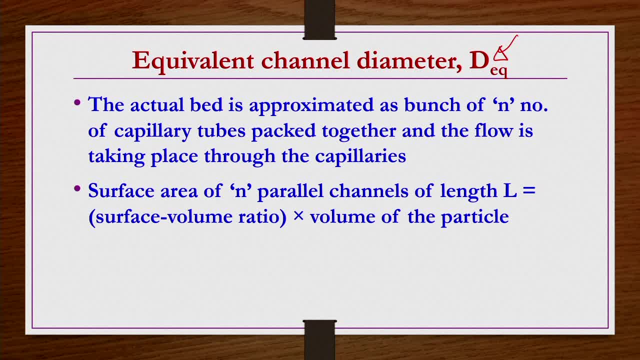 Okay. So then that that would be giving the total surface area of the packed packed structure or packed bed right, That should be equal to the surface area of one channel of length l multiplied by the total number of such channels. okay, So that means if you have n number of channels or capillaries, okay, the surface area of 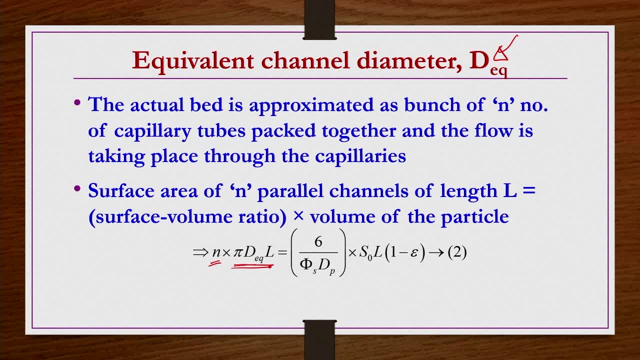 each capillaries. So that is pi d equivalent l, or pi d l, because they are cylindrical capillaries. okay, So the capillaries are, you know each of them are having you know surface area pi d equivalent multiplied by l right. 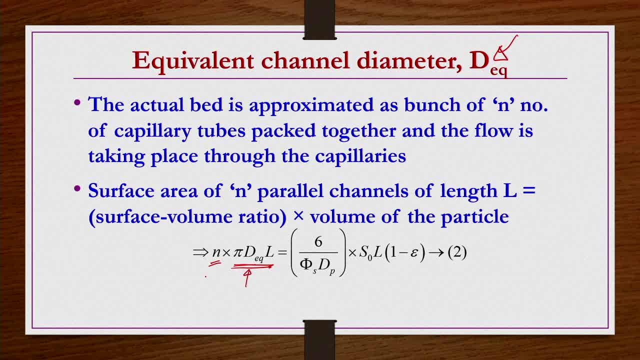 And that should be multiplied by n, because n number of capillaries are there. So this is going to be total surface area for n number of capillaries of length. l okay, So Now coming to the particle, real packed bed. 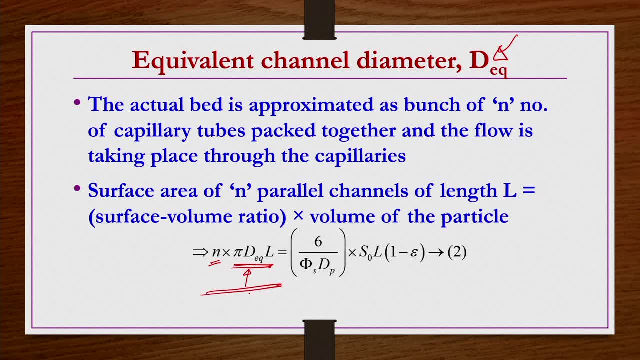 So this is left hand side. it is about the capillaries, which is equivalent to of our packed bed. We simplified it, okay. So now about the packed bed. 6 by pi S dp is what It is: the surface to volume ratio of the particles, irrespective of the size and shape. 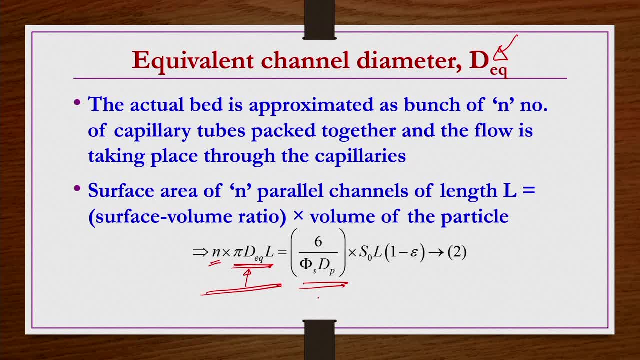 It is true for all size, all shape, regular, regular particles. okay, This one multiplied by the volume of the particles. So, Okay, So, volume of the particles, how do you find? Let us say, this is the packing here. 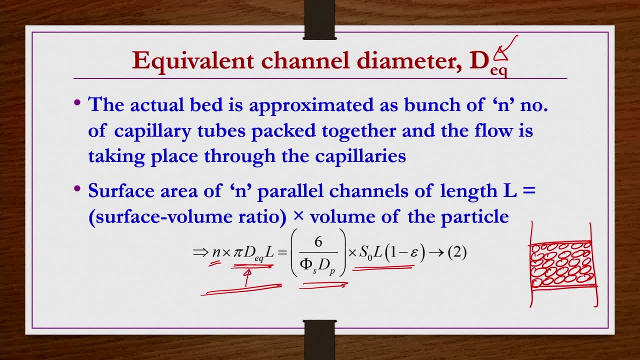 So these are packed between two perforated plates like this. So the cross section area of this- you know, column, whatever is there- that is S naught, okay. Cross section area of the bed is S naught And then height of the bed is L Okay. 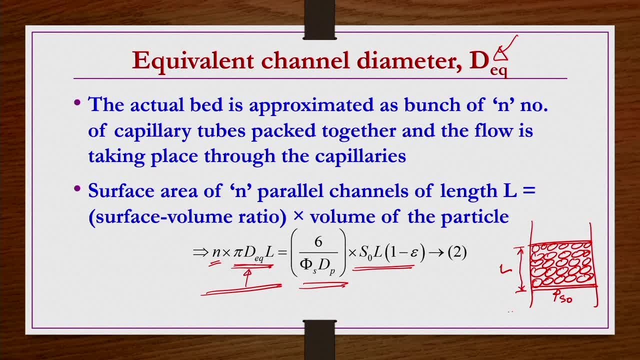 Okay, So volume of the bed is going to be S naught. and then if you want to know the volume of the particles out of this volume, 1 minus epsilon volume fraction is occupied by the particles. Remaining is occupied by the liquid or void space. okay, 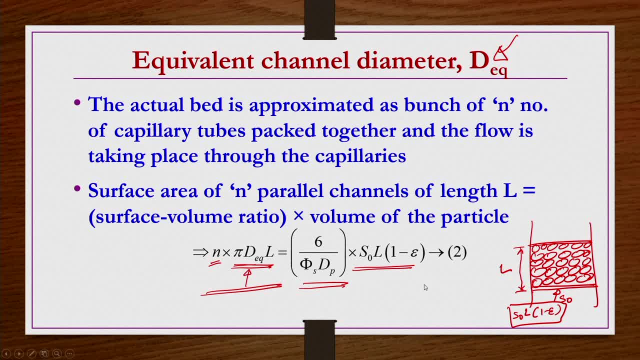 So S naught into 1 minus epsilon is going to be volume of the, all the particles that are present in the packed beds. So surface to volume ratio: 6 by pi, S, dp, multiplied by S naught into 1 minus epsilon. Okay, 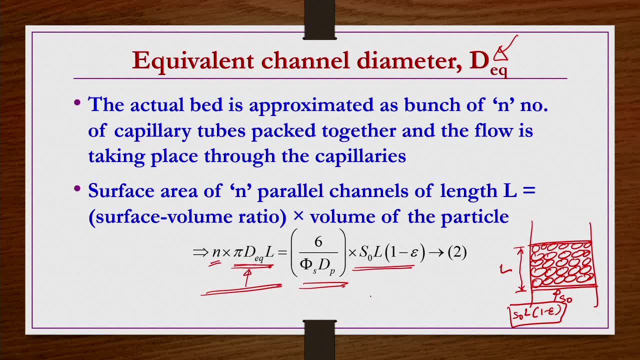 Okay, L 1 minus epsilon. if you do, you will get a kind of a true surface area of the packed bed, that packed bed, whatever the packed bed that we have taken, that is true surface area of the entire bed is this one: that is, 6 by pi S dp multiplied by S naught: L 1 minus epsilon. 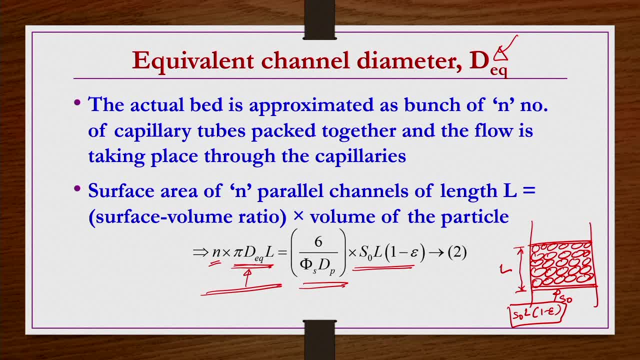 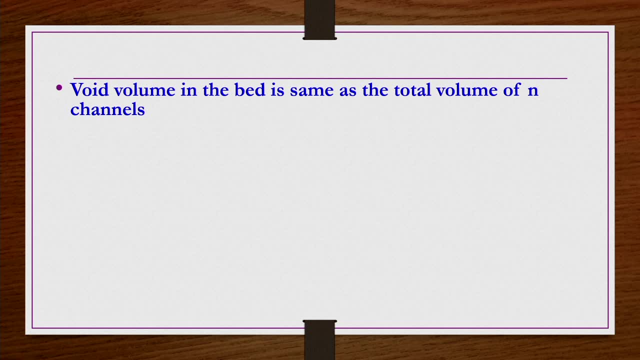 So that should be equal to the total surface area of n number of capillaries, that is, n by d equivalent L. So here S naught is the cross section area of the bed. Now void volume in the bed is same as the total volume of n channels. total, there are n number of channels. 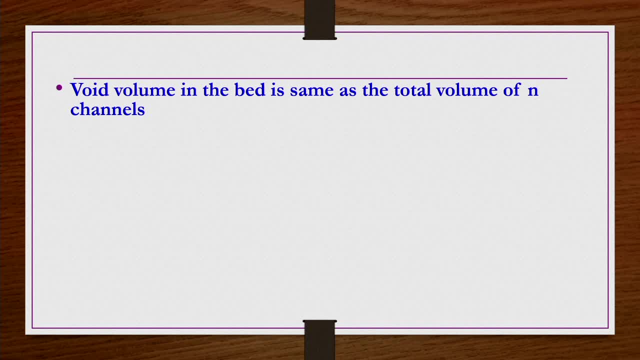 are there? whatever the volume of each channel? is there that if you multiplied by total n number, that should be equal to the existing void volume within the bed, because 2 are equivalent? So then when you do this one, so similarly, as I mentioned that S naught is the cross. 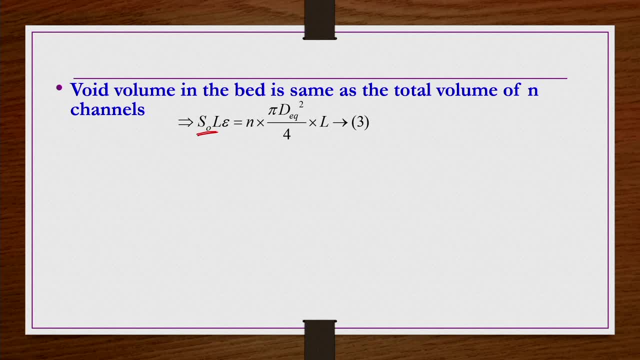 section area of the bed. L is the height of the bed or the height of the packing that we have done. So S naught, multiplied by L is going to be volume of the bed, the entire volume of the bed, which is consisting of both solids and, you know, void space or the liquids. 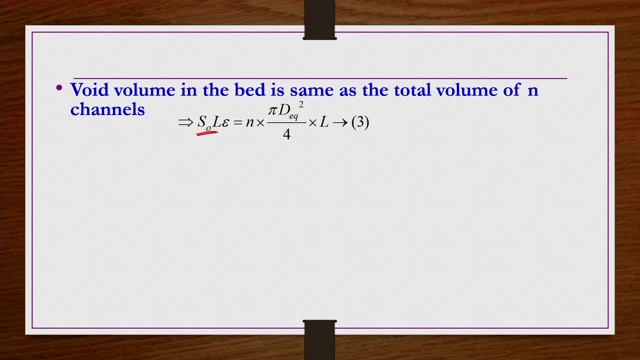 So out of this total S naught L volume, only epsilon fraction is in the bed. So this is, you know, void volume. 1 minus epsilon fraction is solid volume. So here we wanted to know the void volume in the bed, So that S naught L multiplied by epsilon will give you the 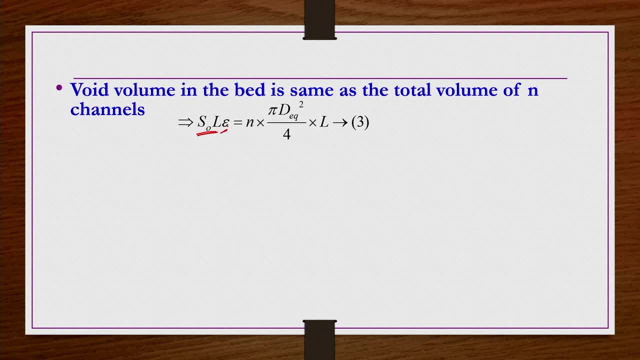 void volume in the bed, So that void volume should be equal to the void volume provided by n number of, or bunch of, n number of capillaries or channels. So there, capillaries, you know, we have this. each capillary of size, you know. 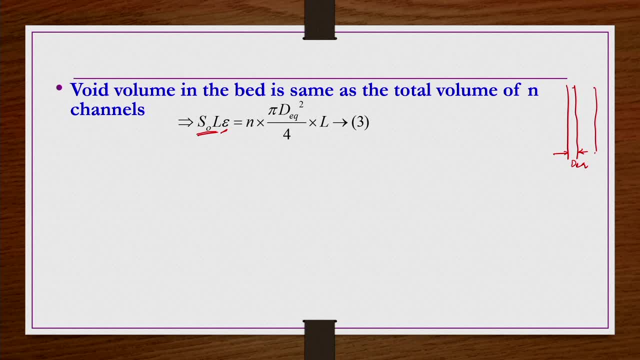 This is d equivalent diameter and then height same as the height of the bed. So cross section of this capillaries is pi d equivalent square by 4 multiplied by L. if you do that is the volume of this capillary that is available for the flow. So the fluid is flowing through. 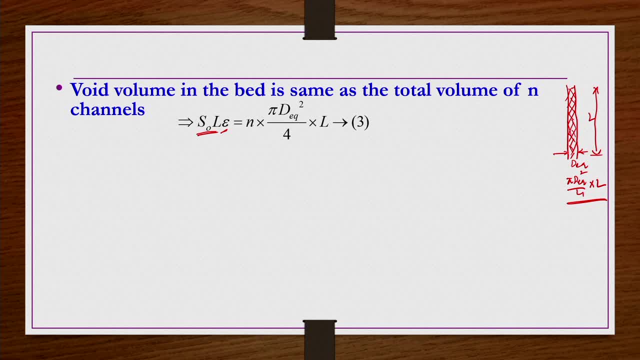 So this volume of the capillary is now pi d equivalent square by 4 multiplied by L. This is one single channel, So there are n number of such channels. there are n number of such channels, so that you know that, whatever the total volume provided by this n number of. 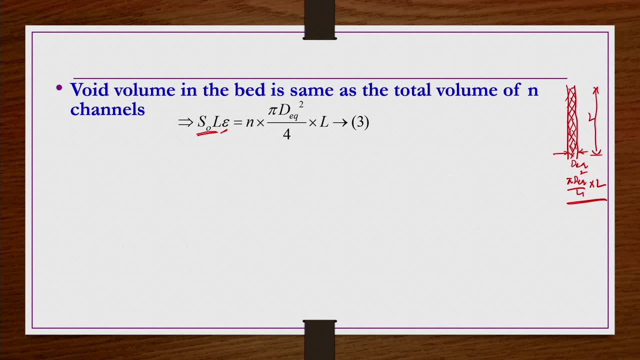 channel is same as the void volume of the real packet bits. So S naught, L epsilon is equals to n pi D equivalent, square by 4 multiplied by L. So now what we do? We take 4 to the left hand side and then 1 D equivalent. also we take to the left hand side. So S naught. 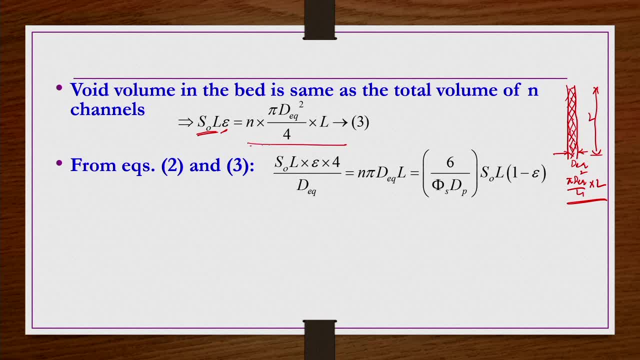 L epsilon 4 by D equivalent. So from here, 4 we have taken left hand side and 1 D equivalent, also we have taken left hand side. So the remaining things are n pi D equivalent L. So this n pi D equivalent L from just previous equation number 2, what we have found, We 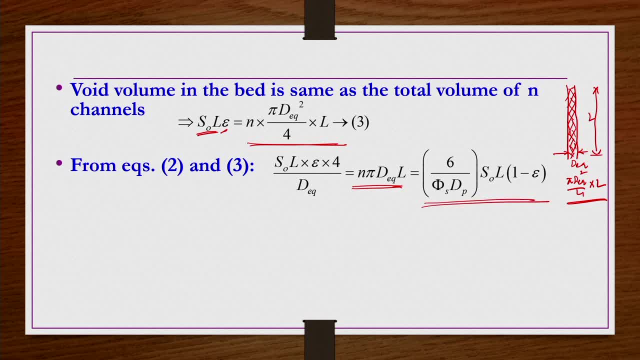 found it as 6 by pi, S, dp, S, naught L, 1 minus epsilon. This is coming From equation number 2.. So now this part. if you equate to this part, then you can find it out: an expression for D equivalent. So that is what our target here, So that we 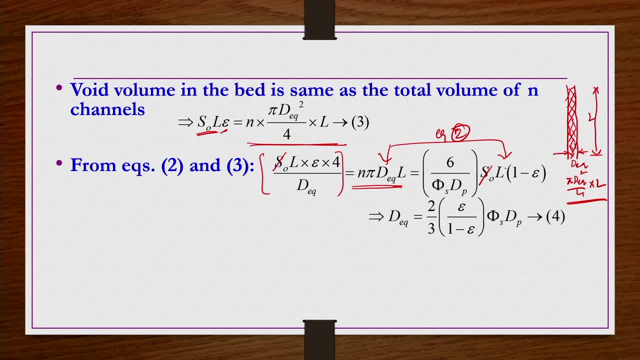 do now. This S naught you cancel out, here S naught. cancel out L and L also you can cancel out. So this is equal to 2, 3ja if you do it. So D equivalent you take to the other side. So 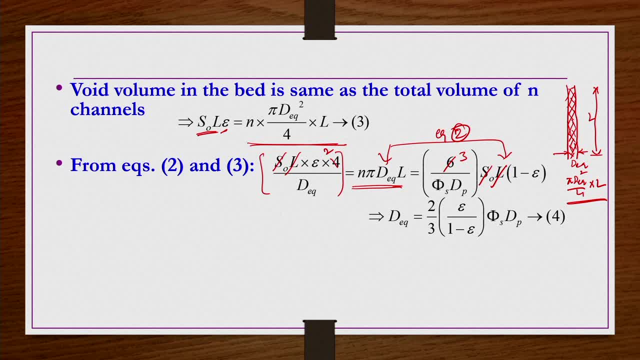 here in the left hand side you have a 2 epsilon as it is, And then from this side, if you bring that pi, S, dp to the other side, so that will be multiplied, and then 1 minus epsilon if you bring it to the other side, that will be divided, So D equivalent what we get here. 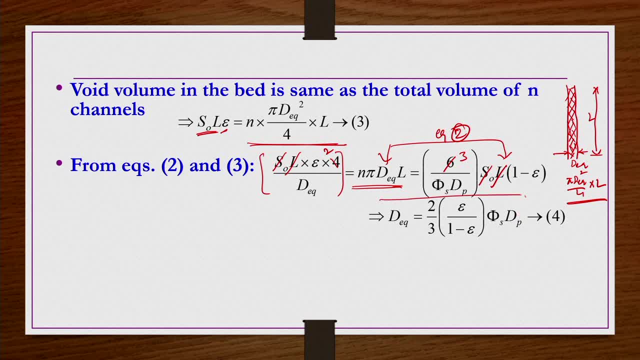 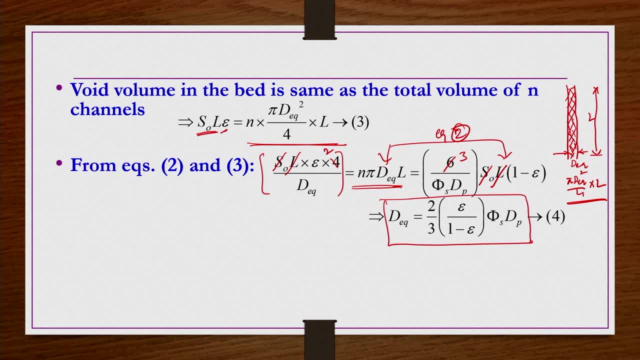 equal to 2 by 3.. So this is equal to 2 by 3, epsilon by 1 minus epsilon, pi, S, dp. dp is volume equivalent diameter of the irregular particle that has been used for the packing of the column D equivalent is the diameter of capillary, and there are n such number of. 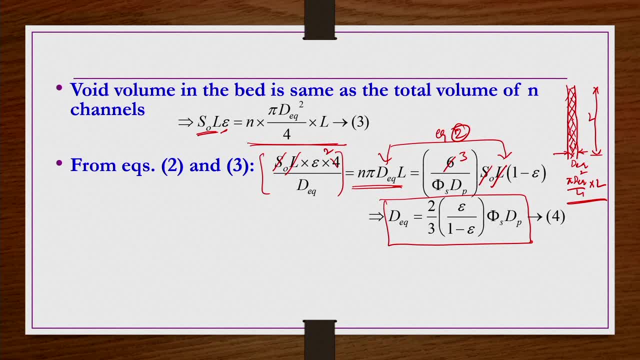 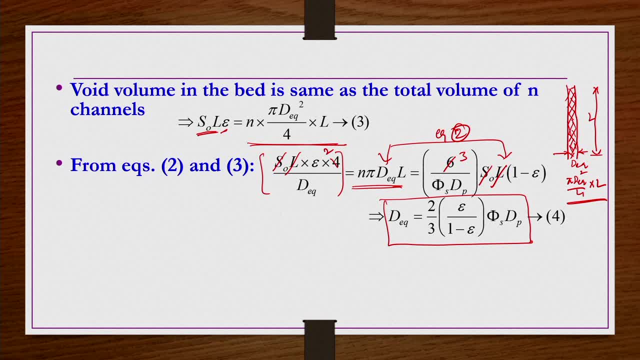 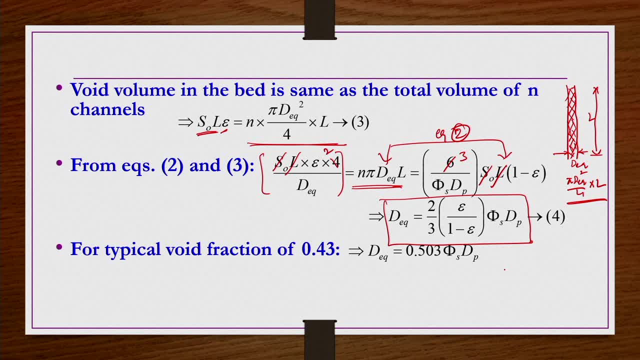 dp. So let us say: if it is a spherical particle, let us say they packing has been done with a spherical particle, So that means there is a vacuum inside. let us say: if there is particle of diameter dp, then d equivalent is equals to 0.503 dp because pi s is equals. 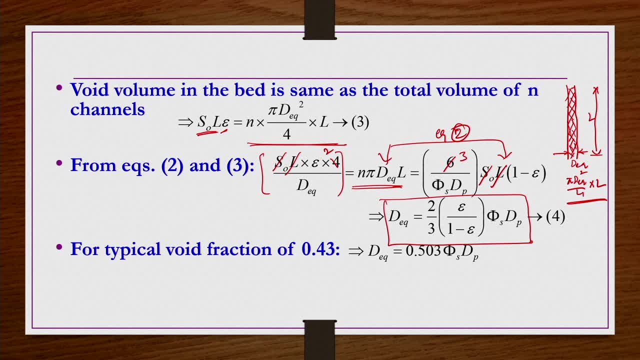 to 1 for spherical particle. So what does it mean? If the packing is done using a spherical particle, then equivalent diameter of which is required for the capillary, so that n number of such capillaries can form a kind of you know bed, having a kind of equal characteristics. 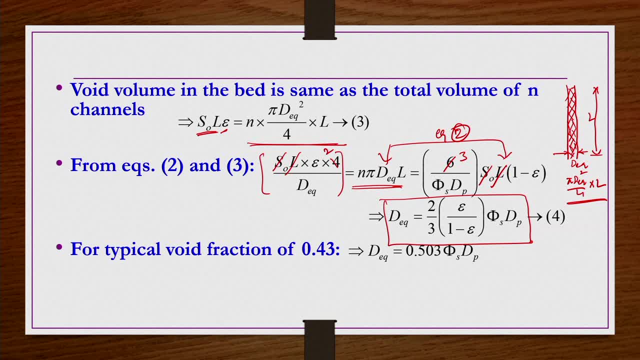 as a kind of a true bed that we have taken. So what does it mean? So that equivalent diameter is half of the diameter of the sphere? If the voidage is 0.43 and the packing is done by the spherical particle, then equivalent diameter is half of the diameter of the spherical. 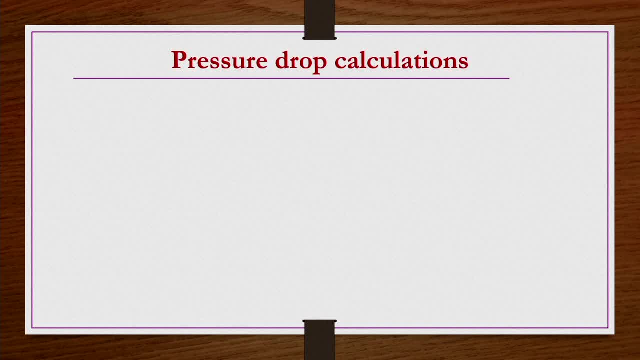 particle. Now what we have to do? We have to find out the pressure drop calculations. So delta p depends on the average velocity in the channels v bar, which is not known. Superficial velocity is known. How much you know empty tower velocity? you are providing that you. 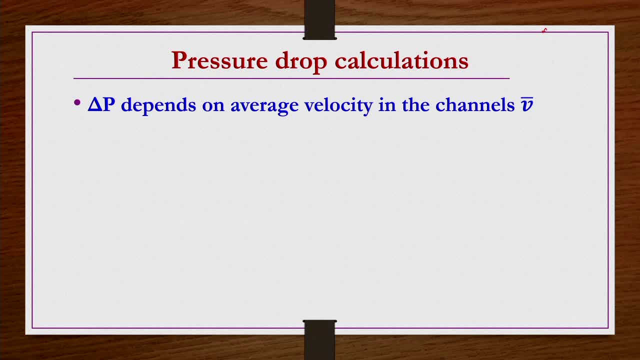 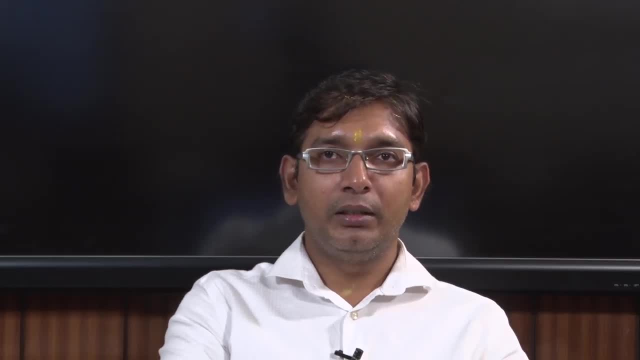 can know, because average velocity is going to change from packing to the packing or from packing is a kind of irregular packing and then size and shape are different from you know. shape of the particle is also irregular and then size is also be going to be different from one particle to other particle. 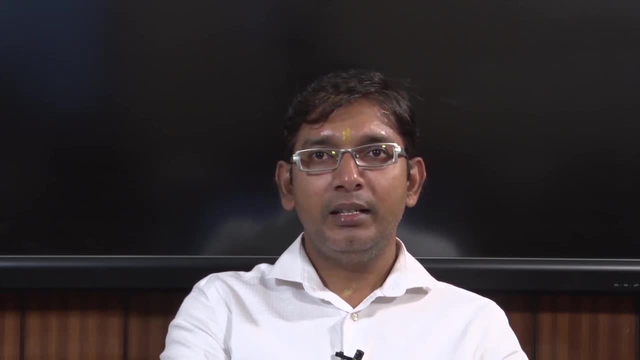 Then nor all theicha Fields are not going to be regular, Then definitely the velocity is not going to be the average velocity is not going to be same from one experiments to the other experiments. That we cannot know Or you know. you can know from the experiments any way by doing experimentally. but however, 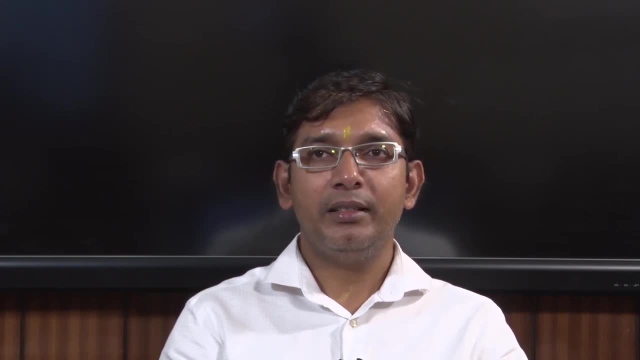 in applications without. this is simplification, theoretical analysis. why are we doing? because without doing experiments a priori, we can calculate how much pressure drop is required. They started to Dogman systems. Havel Works are not going to不同: the same siguients. 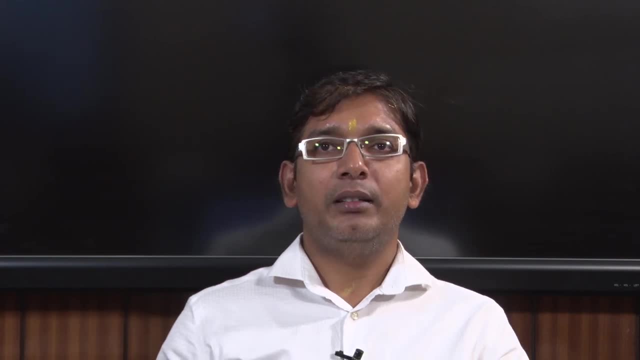 And so testament are going to be 0, since Because, without doing it, fragment is depak président Go to Ls. we calculate how much pressure drop consciously. he is required this software difference for a packed bed of certain height and certain porosity, etc. for that purpose we are doing. 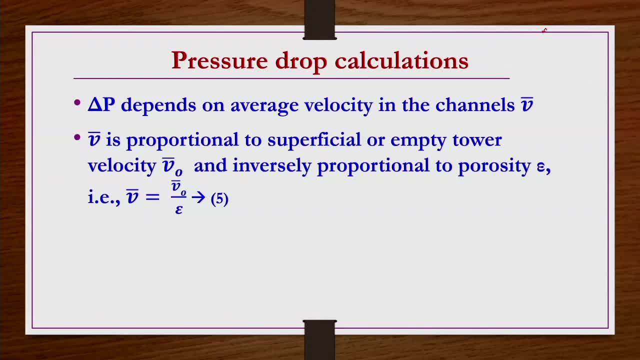 it okay. So then this V bar is proportional to superficial velocity or empty tower velocity- V, not bar- and inversely proportional to the porosity, so that V bar is equals to V, not bar by epsilon. So in this equation in place of V we replace V by V bar, that is V, not bar by epsilon. and 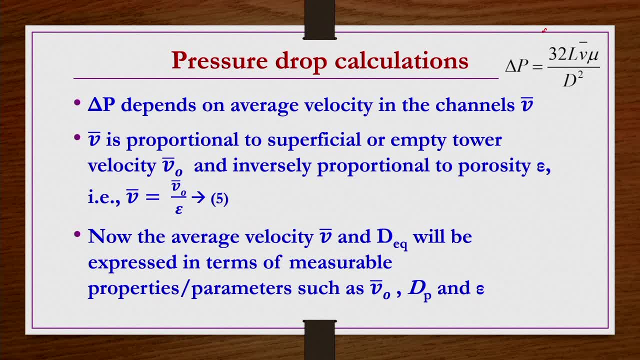 then D we replace by D equivalent. simply do that. So now the average velocity, V bar and D equivalent will be expressed in terms of the measurable properties or parameters such as V bar, Dp, epsilon, etc. and those things will be used in this equation. 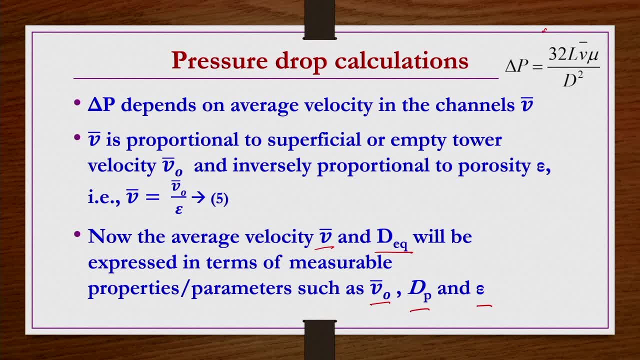 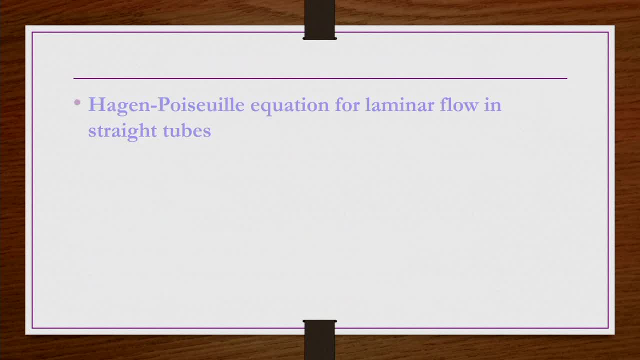 So indeed, D equivalent. we have already represented in terms of this Dp, epsilon and then Vr. just now we have seen it is V, not bar by epsilon. This information we are going to use in this Eigenpolitik Eigenpoise equation for laminar flow in straight tubes without any packing in straight tubes. 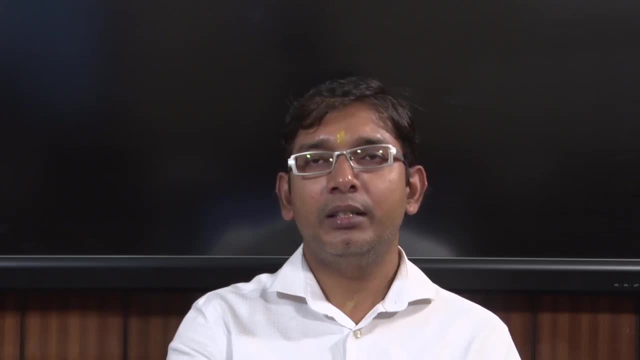 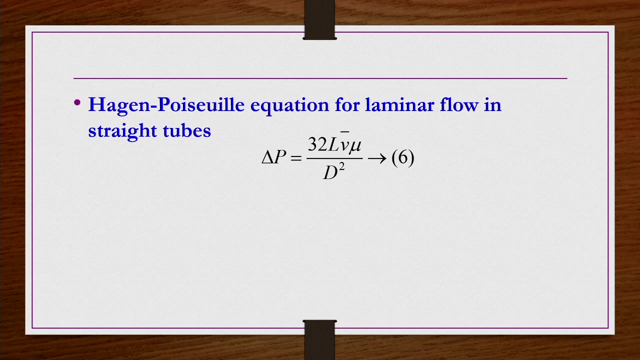 without any packing. if the fluid is Newtonian and then fluid is flowing under laminar flow conditions, then pressure drop is 32 L V bar mu. by this we already know here. So then what we do here- We substitute V bar is equals to V, not bar. by epsilon D. we replace by D equivalent and. 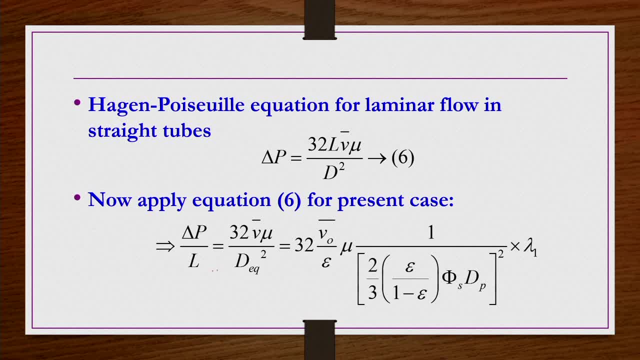 simplify. So then when we do it, 30. Delta P by L is equals to 32 V bar. mu by D equivalent square 32 V bar is nothing but V, not bar by epsilon mu. and then 1 by D equivalent is 2 by 3 epsilon by 1 minus epsilon pi s. 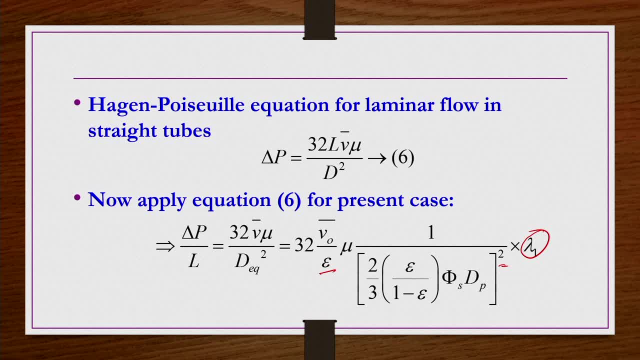 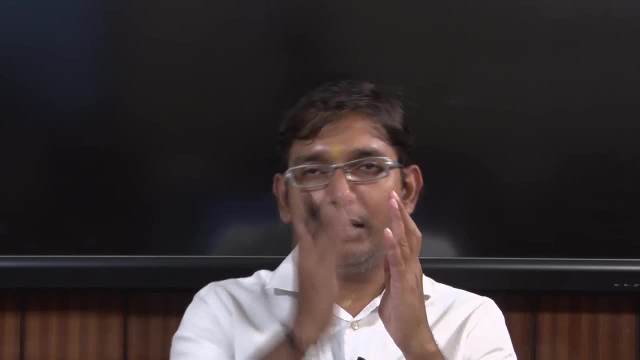 Dp whole square, and this multiplied by a factor lambda, 1.. Why it is Because in straight pipes, straight tubes, etc. like capillaries, if there is a laminar flow, when there is no obstacle, So there is fluid- elements are traveling the same distance as the height of the pipe or 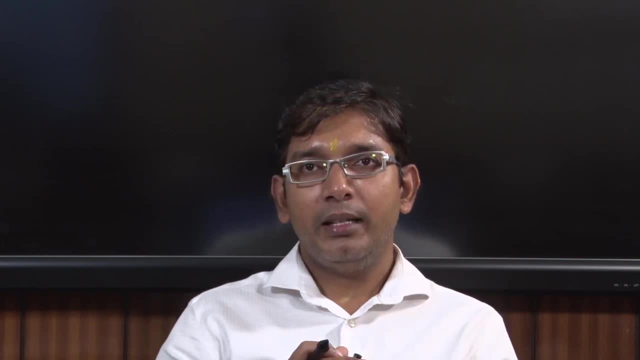 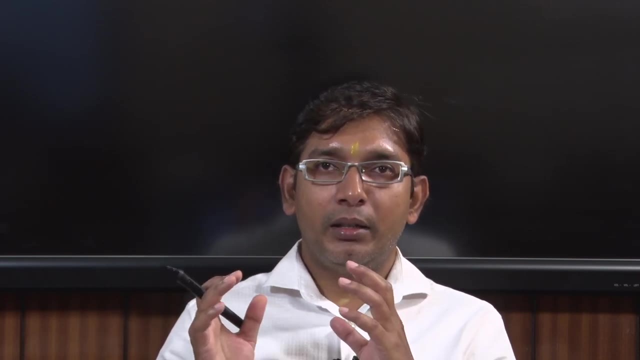 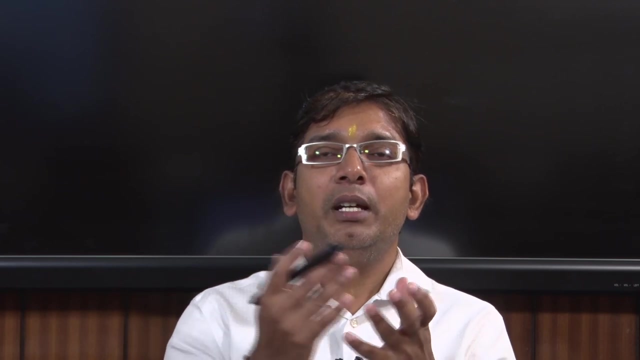 the length of that pipe that you have used, But in the packing, the fluid element. if you are packing that column with some kind of packing material, some particles etc. then what happen? this fluid element is traveling more than the height of the packing because of the tortuous path. 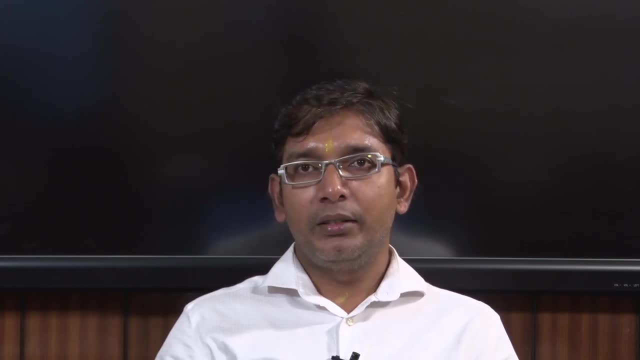 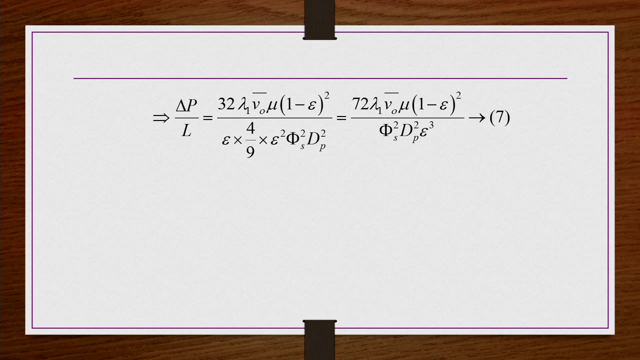 So, in order to bring in those information, We are taking this fraction, lambda 1.. Let us not worry about what is this lambda 1 value as of now. Now this equation, you rearrange and simplify it. So then what we have, delta P by L is equals to 72 lambda V, not bar mu 1 minus epsilon. 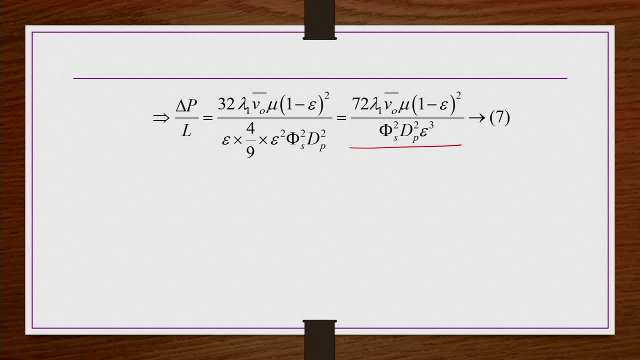 whole square by pi s square, Dp square, epsilon cube. This is what we are having it. So now here V bar is. superficial velocity is known How much velocity superficial velocity you want to provide, that you know. And then viscosity of the fluid, you know the void space of a bed, characteristic that in 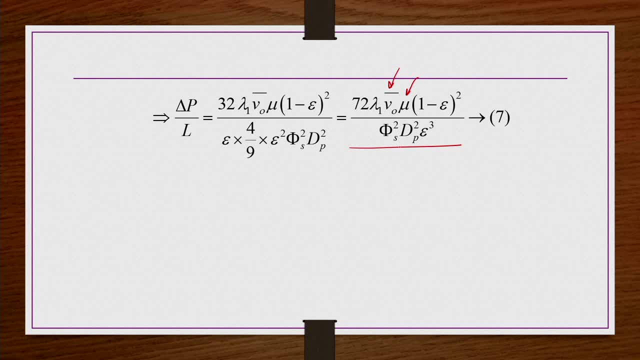 general. you know Dp and the volume sphere, volume equivalent diameter of irregular particle. you know sphericity of the particle. also, you know, or you can know, the way that we calculation that we have done in module 1.. Right, So then everything is known. 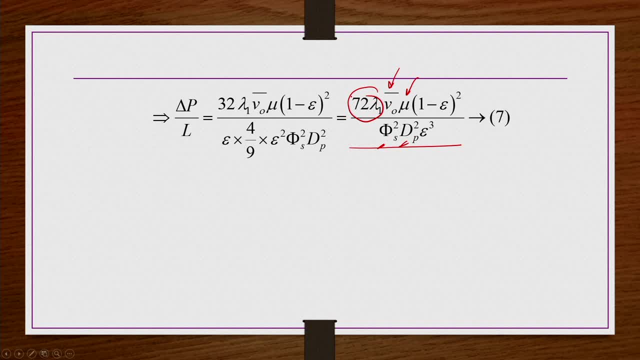 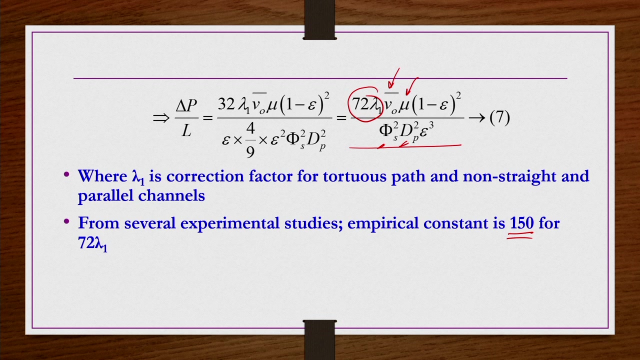 Here, except this one, lambda 1, right, But this lambda 1 is a correction factor for tortuous path and non-straight parallel, non-parallel channels, in general irregular channel. that is what I already mentioned. right, But from experimental studies, empirical constant is found as 150 in place of 72, lambda 1.. 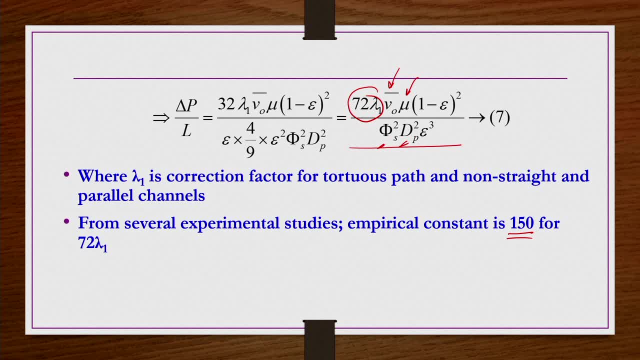 So like you do the experiments right And then try to maintain the laminar flow conditions, Then if you represent your results, delta P, by L as function of these parameters, like this, you will get 150 V naught bar mu 1 minus epsilon, whole square by pi s square, Dp square. 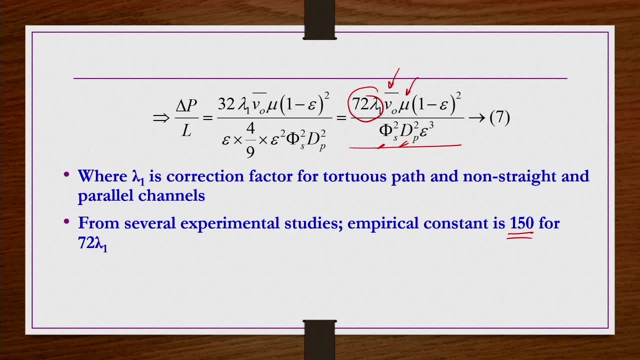 epsilon cube or you know, theoretically, whatever the values that you get here other than these things, if you calculate So that constant is coming out to be close to 150.. Right, Okay, Okay. So this delta, P by L are the pressure drop, okay? 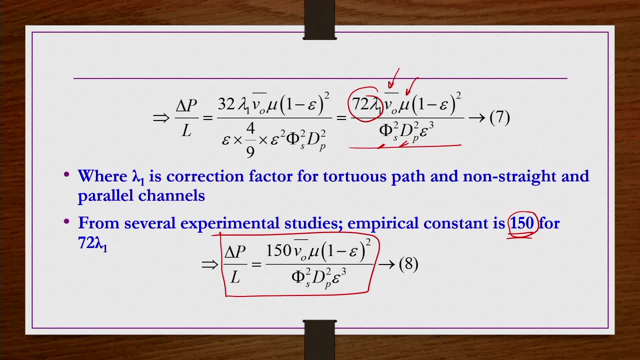 Pressure drop for a fluid flowing through packed bed of packing height, lambda bed. having the void space epsilon, then packing has been done with some kind of irregular particles. If the flow is laminar flow, then pressure drop. you can calculate using this expression without doing anything. 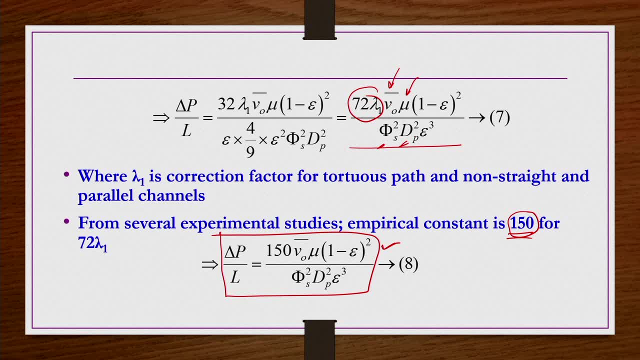 Okay, Because this has been found consistent with the experimental study. If you replace that 72 lambda 1 as a kind of 150, okay. This equation is known as the Kozeny Carman equation and valid for Re up to 1 only small. 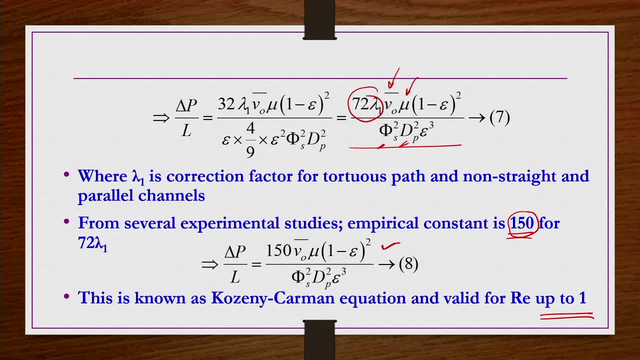 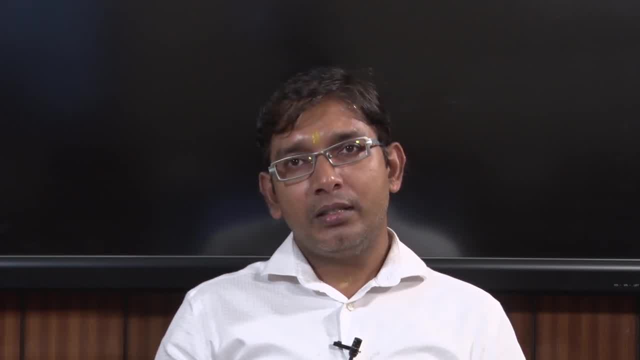 Reynolds number only. it is valid, As I already mentioned, in the straight pipes without any packing kind of thing. we have seen That laminar flow conditions are existing up to Reynolds number of 2100, something like that. But if the same channel or the tube, if you have some kind of packing in between to have 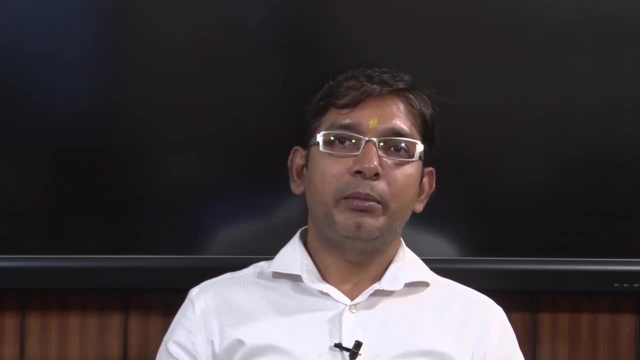 a kind of packed bed. so then the flow is not going to be laminar beyond Reynolds number of 1.. However, some people take approximation of Reynolds number up to 5 to 10 is also laminar, but in reality this equation is valid only up to Reynolds number of 1.. 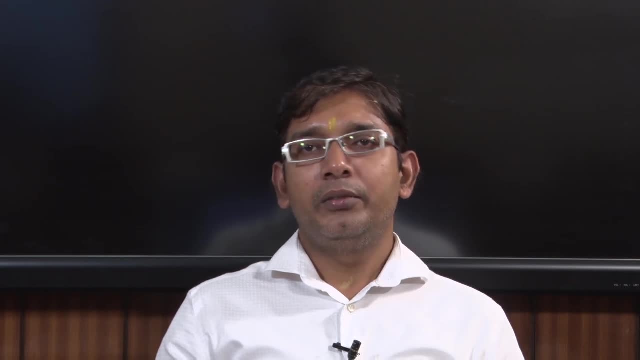 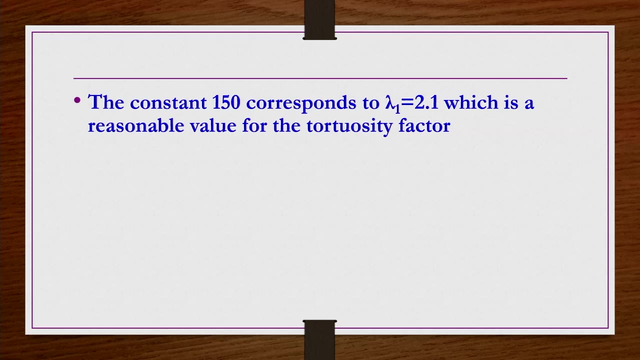 Okay, Okay. So this is for the laminar flow conditions. Same thing we do for a kind of turbulent conditions also. But before going to do this one, the constant 150, if you equate to the 72 lambda 1, then 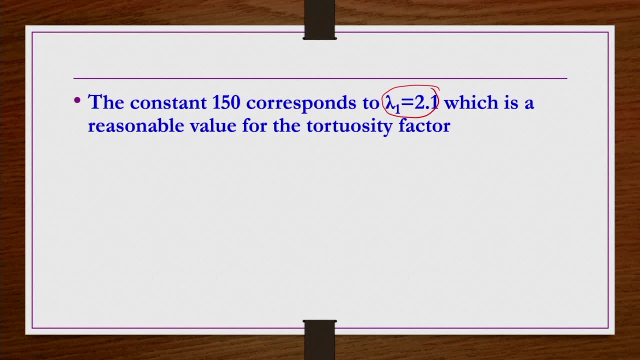 what you get. Lambda 1 is approximately 2.1.. It is fluid element is, on average, travelling twice the or 2.1 times the length of the packing or the height of the packing. Okay, So that is a reasonable value for the tortuosity factor in general for tortuosity factor. 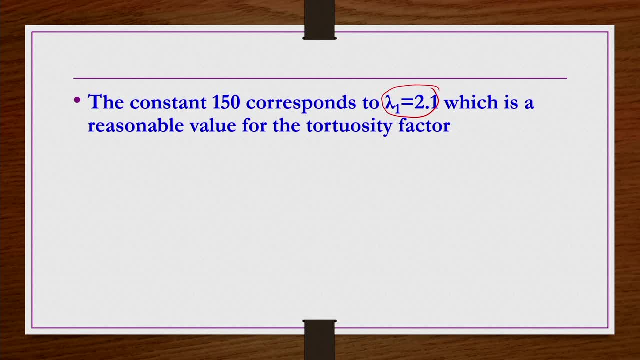 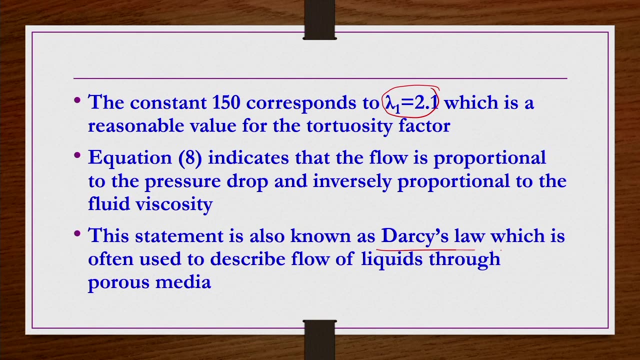 So that is not a kind of a very blind value kind of thing. So that is acceptable one. So equation A: it indicates that the flow is proportional to the pressure drop and inversely proportional to the fluid viscosity. So this statement is also known as the Darcy law, which is often used to describe the flow. 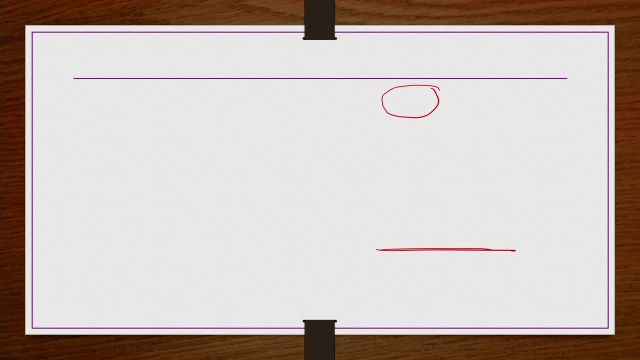 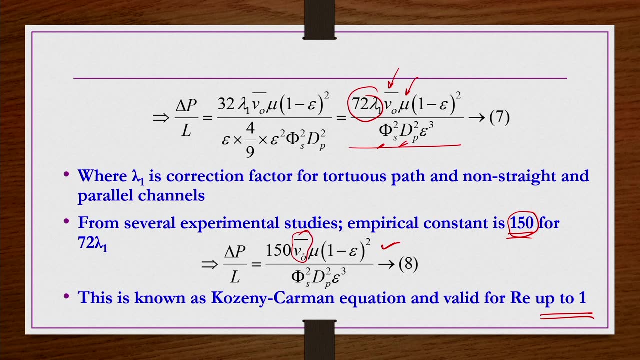 of liquids through porous media. So here we can see, Okay, You can see this, V naught bar the flow velocity. flow, whatever is there. flow velocity is there that is proportional to the pressure drop and then inversely proportional to the viscosity. 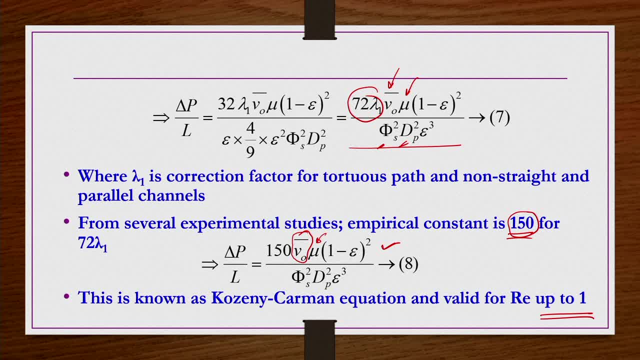 which is consistent as a kind of a Darcy's law which is used for a flow through porous media. And then other thing I was mentioning, like you know, for a given packed system, if you calculate delta P by L experimentally, let us say if you use a regular small particle, 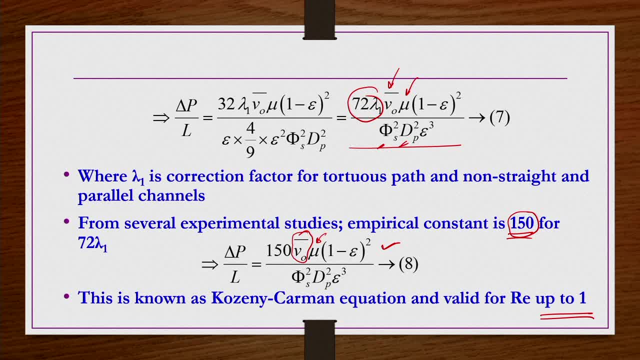 the excrement, pigment particles etc. for which you do not, you find very difficult to measure Sp by Vp ratio. you make a packed bed with those particle and then experimentally you find out what is this pressure drop Right? So then from here you can back calculate what is Pi s dp, so that from here you can 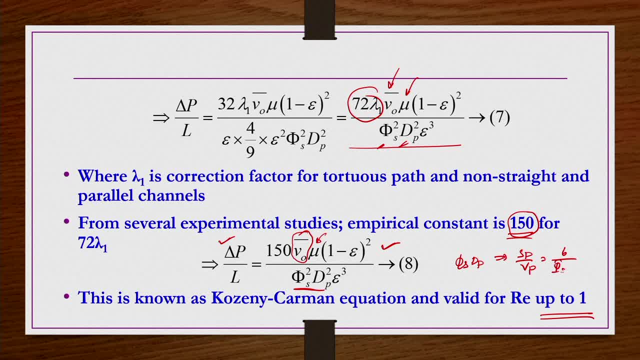 find out, Sp by Vp is equals to 6 by Pi s dp. Okay, So this is the other advantage of this equation, Only thing that you know for the particles for which you wanted to find out Sp by Vp ratio, which is not possible or very difficult to find out using the other conventional ways. 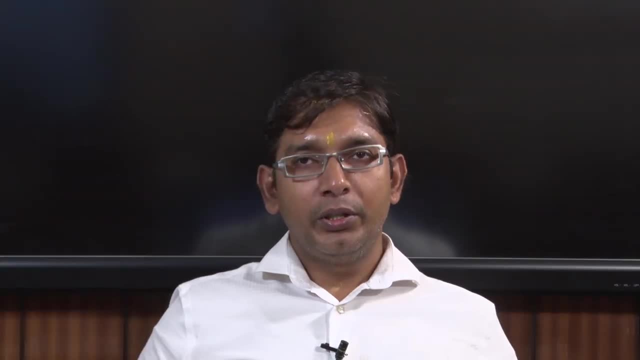 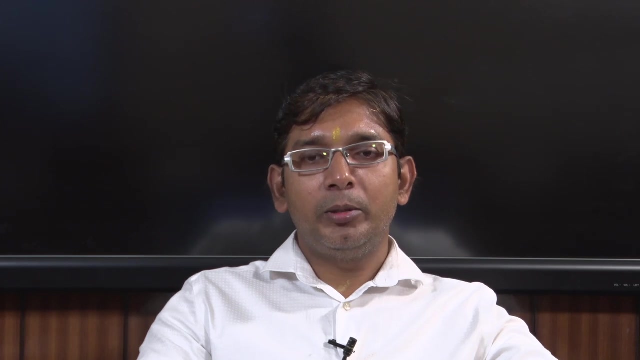 because of inherent difficulties. then you use those irregular particles, small particles, as a kind of packing material and form a packed bed and do the experiments, find out delta, P or pressure drop experimentally. Okay, So that pressure drop you can use here in this equation and then back calculate what. 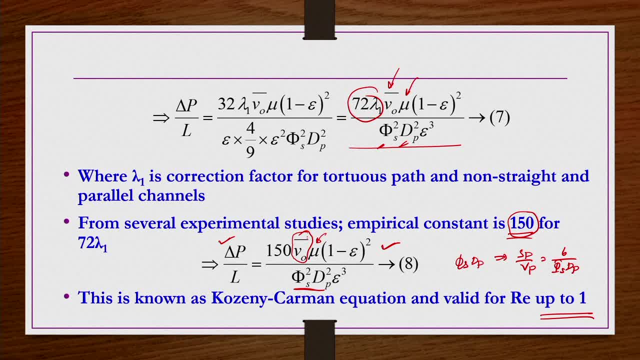 is Pi s dp, because remaining things are known experimentally. how much superficial velocity you have, given that you know, viscosity of the fluid, you know, and then void space of the bed in general, you know, or in general it is around 0.4 to 0.45.. 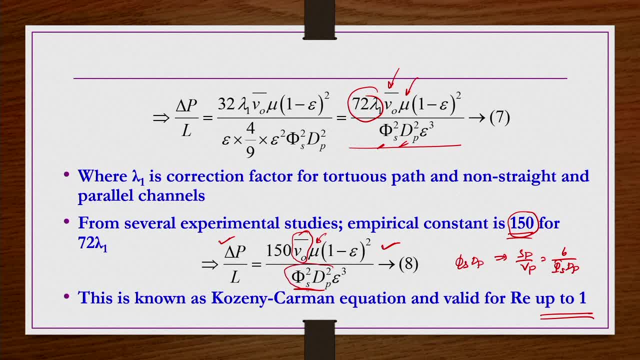 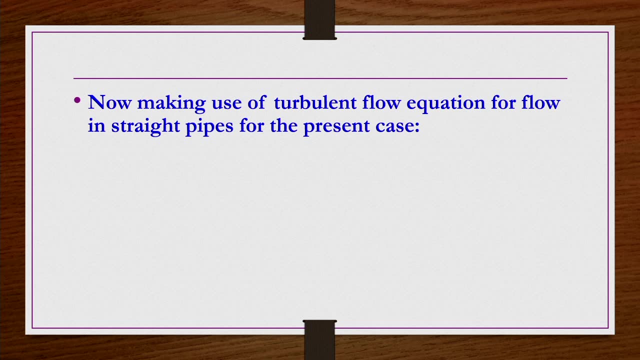 So you can calculate Pi s dp from here, because rest everything is known once Pi s dp is known. So Pi s dp, you will get surface to volume ratio for those particles. Okay, So now making use of turbulent flow equation for flow in straight pipes. for the present, 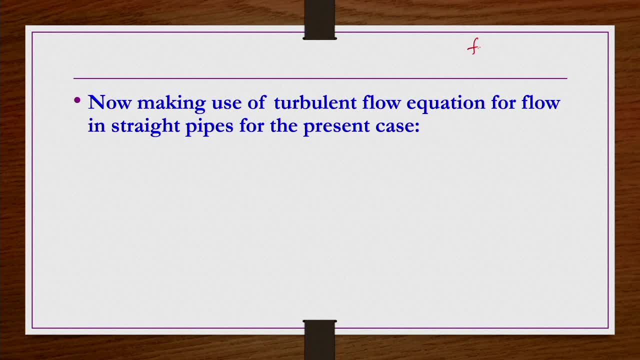 case. So what we do? We have this friction factor expression F is equals to tau w by Rho V square for flow through pipe. So this one we can write it as a kind of tau w. we can write minus delta P by L. So 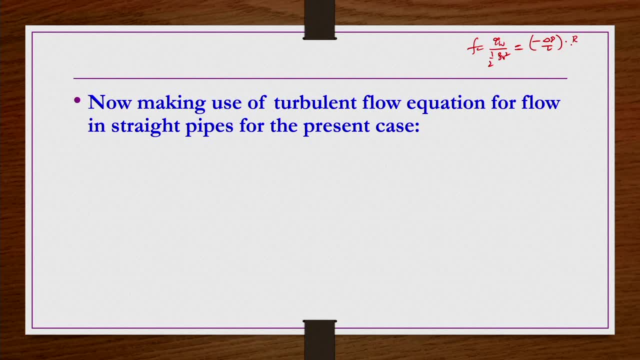 this is the expression. Okay, So R by 2, R is the size of the that pipe of rho V square. you can do it. So that means there is a relation between F and minus delta P by L. So that relation. 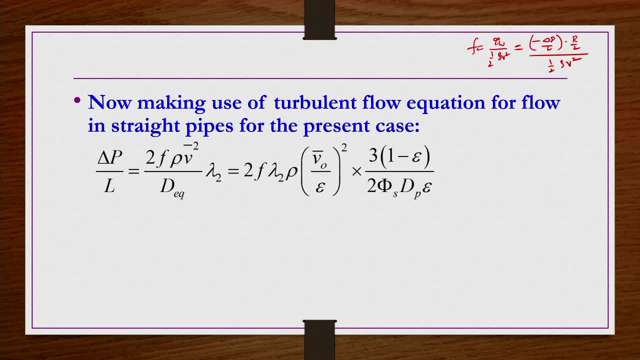 if you write it, rewrite it here in this form: delta P by L is equals to 2F rho V square d equivalent divided by d equivalent here. So this R, we can write it as d by 4.5.. Okay, So d by 4 or d equivalent by 4.. 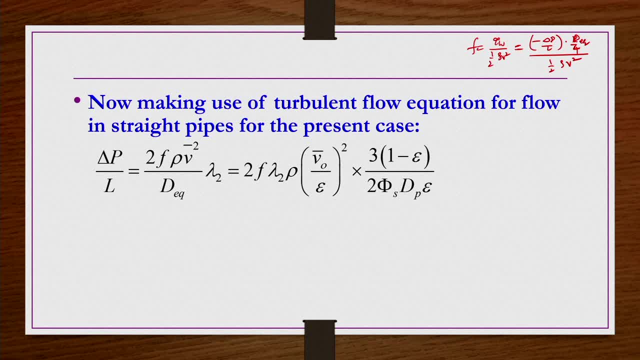 Then we have this equation: Right: 2 ones are 2, fours are 2 ones are 2, twos are 4.. So then we have: 2F is equals to minus delta P by L d equivalent divided by rho V square. 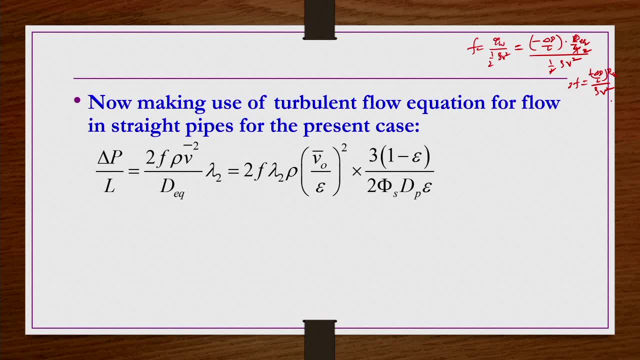 or minus delta. P by L is equals to 2F rho V, square by d equivalent. Okay, So this is the expression, the tautuosity factor for a, you know, irregular packing that we are having in the bed Right. 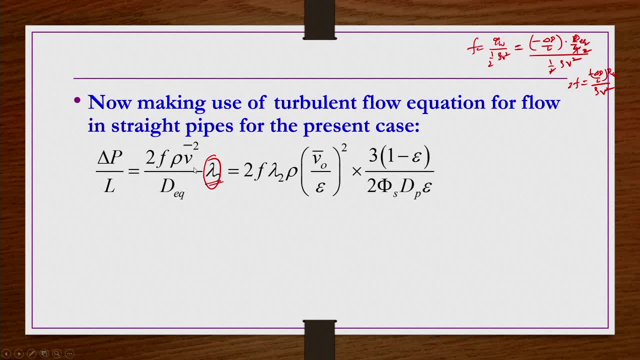 So we are not writing lambda 1, we are writing lambda 2.. Why? Because lambda 1 is valid for a kind of a laminar flow conditions. So if the flow velocity is changing, the fluid element that is traveling or the tautuous. 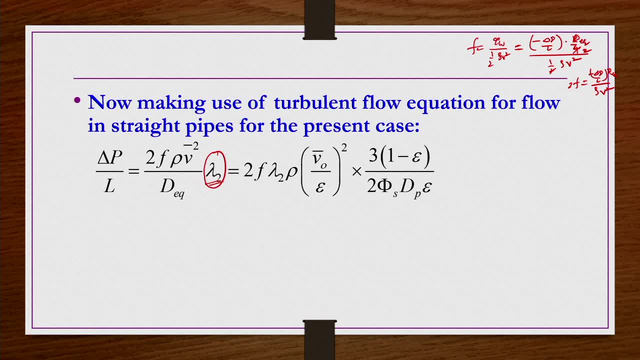 path of that you know, for a given fluid element may be different. Okay, So let us take a lambda 2.. So if you rearrange this equation like this, you have 2 f lambda 2 rho in place of v bar. 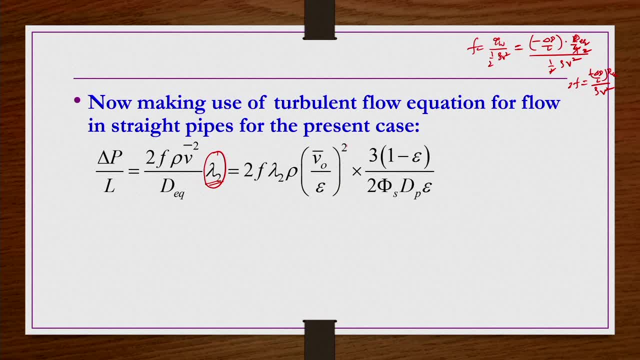 we can write v bar, v naught bar, divided by epsilon, so whole square, and then in place of D equivalent you can write 2 by 3 pi, s, dp, epsilon by 1 minus epsilon, so that you put it here, substitute here and then simplify it, so you will get delta: P is equals to 3. 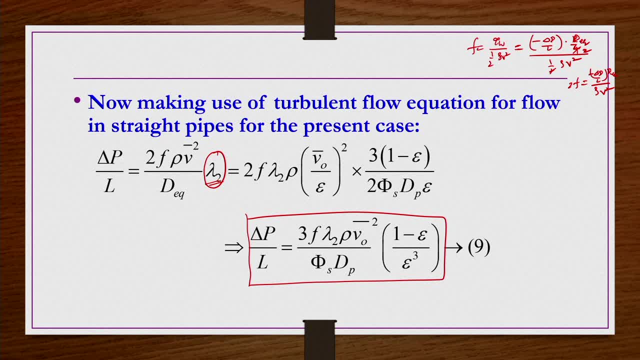 f. lambda 2: rho v naught square divided by pi s dp multiplied by 1 minus epsilon, epsilon cube: okay, So lambda 2 is a tortuous, is a correction factor for the tortuosity or tortuous path that is existing in the packed bed. 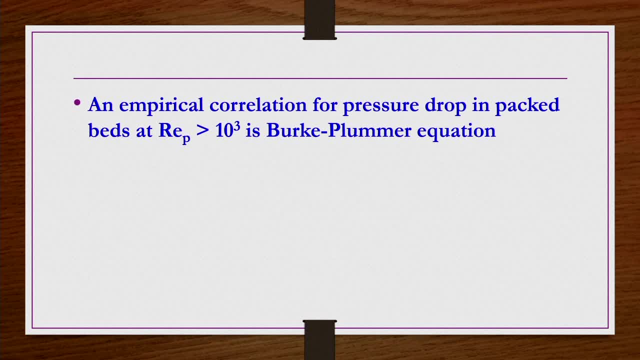 Now an empirical correlation for pressure drop in packed beds at Rep greater than 10 power 3 is known as the Burke-Plummer equation and it is given as This thing. this is empirical correlation developed by Burke-Plummer, so according: 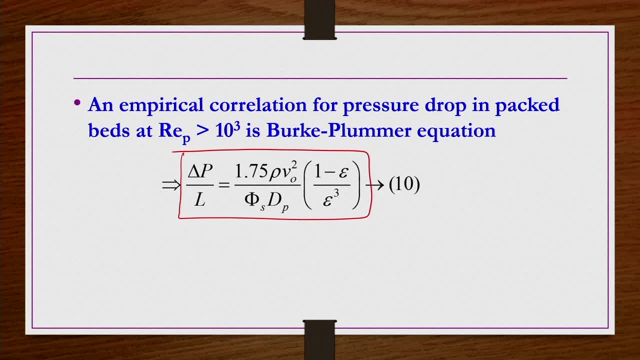 to them for the flow through packed beds. when Reynolds number is greater than 10, power 3, delta P by L is equals to 1.75 rho v naught square, or rho v naught bar square, divided by pi. s dp multiplied by 1 minus epsilon divided by epsilon cube. 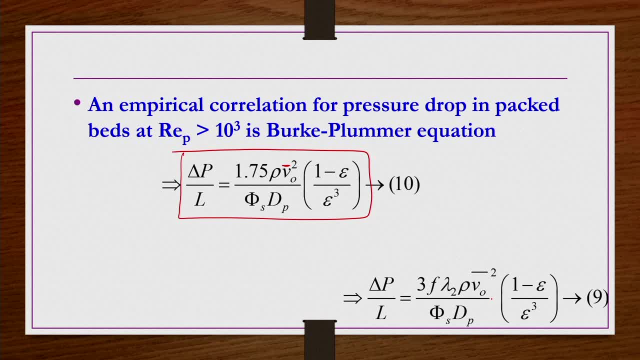 Now this. Now this equation number 10, if you compare with our equation number 9, just, we derived theoretically. this is empirical correlation. Equation number 10 is empirical correlation developed by these people, Burke and Plummer. okay, 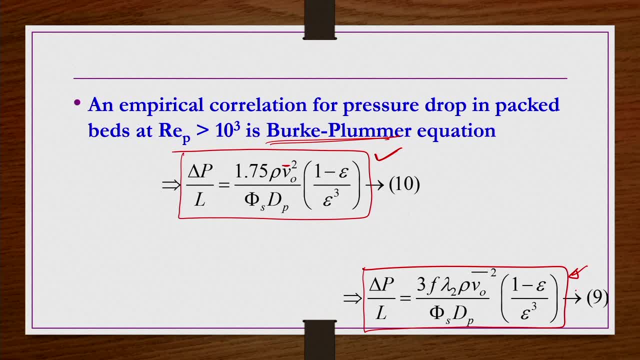 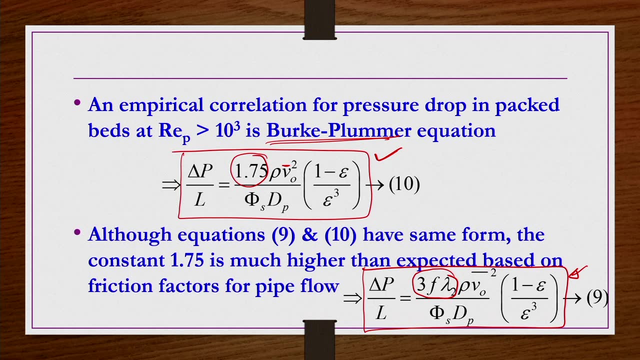 And then this is the theoretical equation that we just developed, based on the theoretical information that is available. So what we understand here, this 3 f lambda 2 is equal to 1.75 and rest everything is same, right. So, although equations 9 and 10 have same form, the constant 1.75 is much higher than 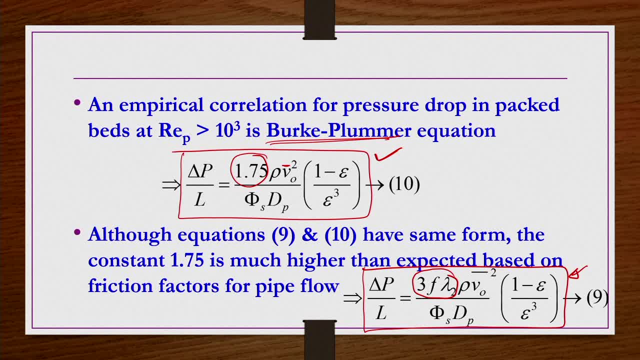 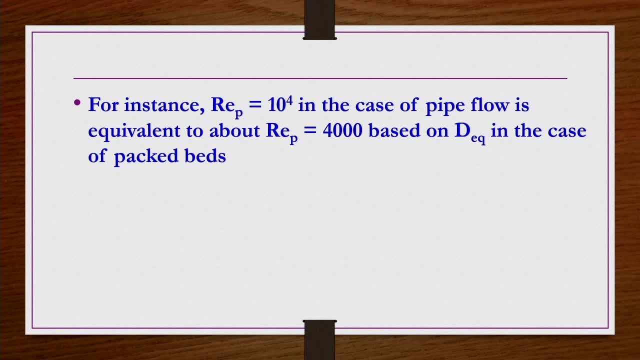 expected value based on friction factors. pipe flow: for the pipe flow cases. So whatever the Reynolds number of you know, 4000 is there in general for packed bed, which is equivalent to Reynolds number of 10 power 4 in the case of pipe flow without any packing. 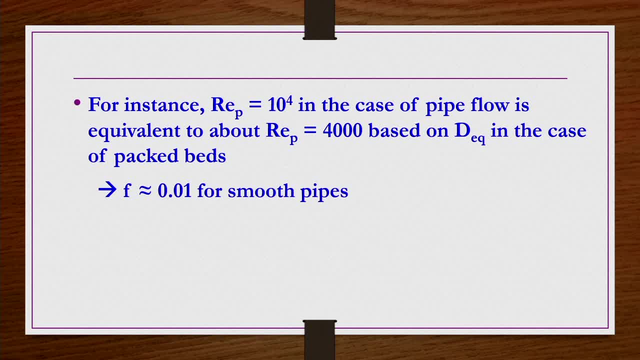 right. Under such conditions f is approximately 0.01 for smooth pipes. okay, This is fanning friction factor versus Rdp for pipe flows charts are available. from those charts we can find it out that at this Reynolds number, Rdp of 10 power 4 for pipe. 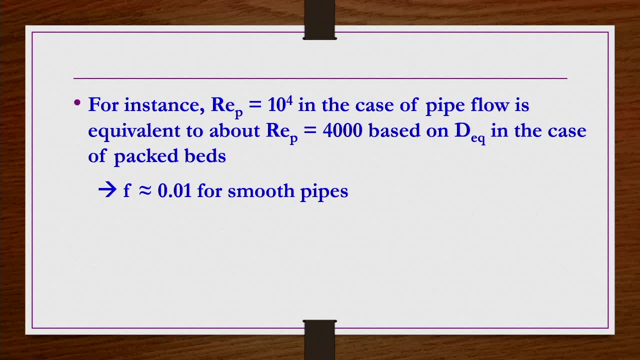 flow. at that Reynolds number, friction factor is approximately 0.01 for smooth pipe In the pipe flow where there is no packing, if Rdp is order of 10, power 4, so that is equivalent to Rdp of 4000 in the case of packed bed in general okay. 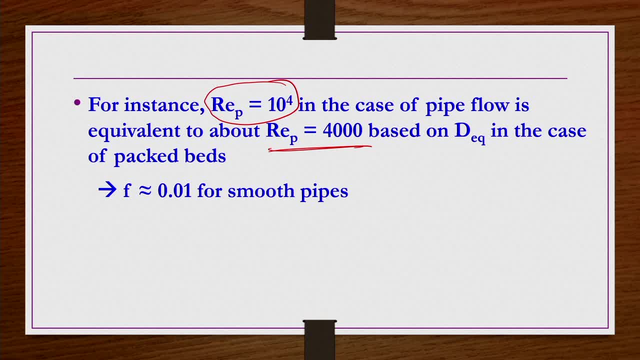 So that is more than order of 10, power 3.. So if you use this one, this expression, in place of 3 years, So if 3f, lambda 2 is equals to 1.75,, you will get lambda 2 is equals to 58, so so, 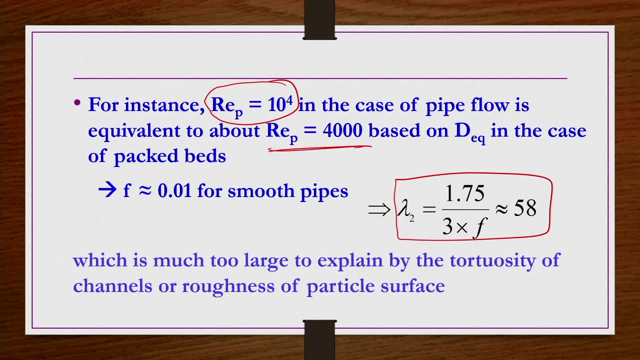 much high value, which seems to be unrealistic in general right, Which is much too large to explain why the tortuosity of channels or roughness of particle surface is you know so large values, like you know 58, something like this. however, you 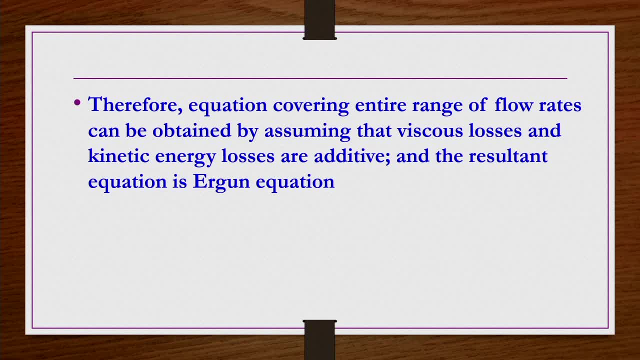 know we can use them, you know, With a constant 1.75, rather using, you know, 3f, lambda 2.. So covering entire range of flow rates. you know one can obtain the pressure drop, you know, by assuming that the viscous losses and kinetic energy losses are additive. then we 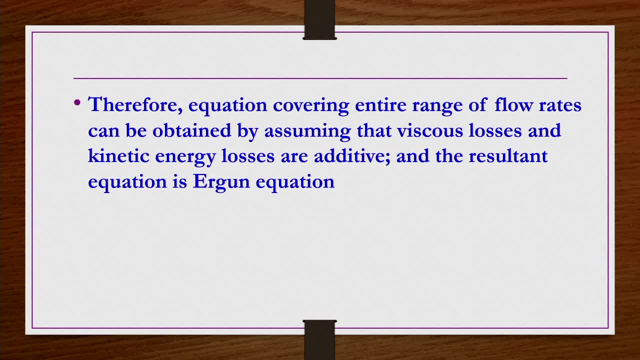 can have a kind of Ergin equation or the first equation, whatever that you know, Kozeny Karman equation that is, delta P by L is equals to 150 by L. Okay, Okay, Okay, So you can see that expression. So that is, you know, considering only viscous effect, small Reynolds number, in the sense. 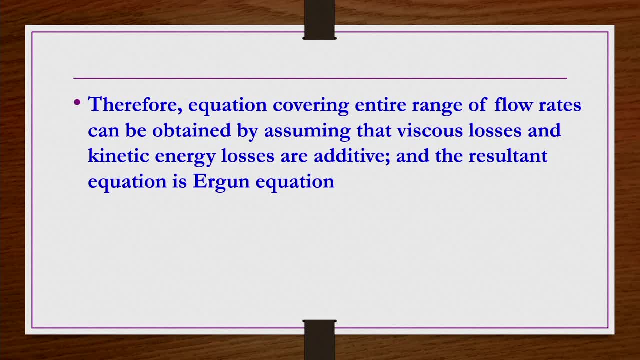 only considering the viscous effects. okay, it is not considering the kinetic energy losses. So, whereas the Burke-Plummer equation that we have, minus delta P by L, is equals to 1.75 and something that expression that is only valid for only large Reynolds number. 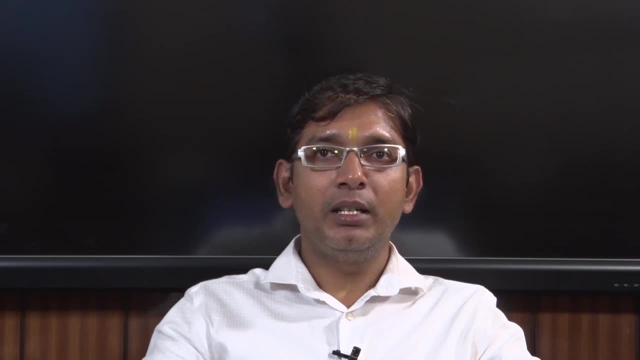 If the Reynolds number is order of 10, power 3 or even more, that means only convection forces only dominates, inertial forces only dominate. So that means you know they are due to the. whatever the losses are there because of the kinetic energy losses are there. 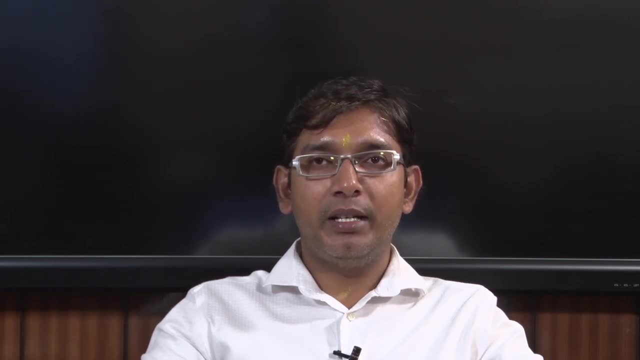 And then these two are the either extremes. one extreme is the viscous losses or for the small Reynolds number cases. another extreme is for the large Reynolds numbers or for the kinetic losses, okay, or due to the kinetic losses. So if you assume that these are, you know, kind of additive kind of thing for the intermittent, 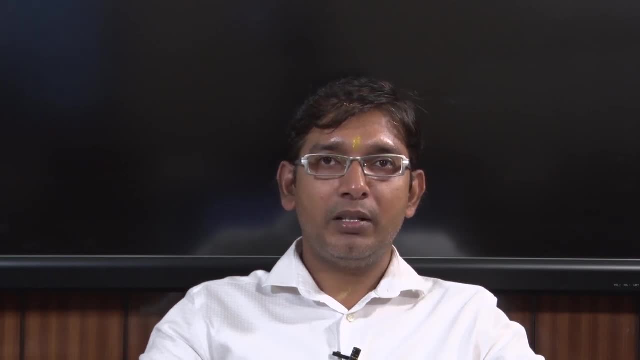 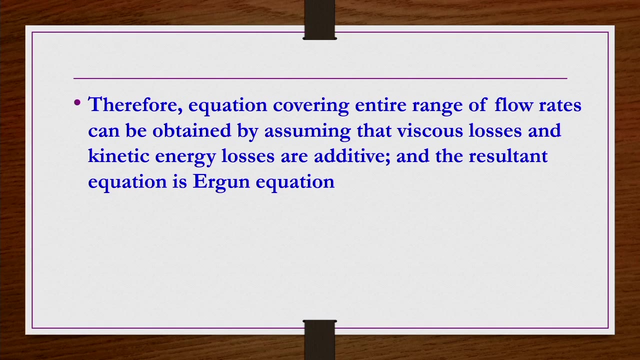 okay, So intermediate range. then you will get you know pressure drop equation for the entire range of Reynolds number, starting from small Reynolds number to the large Reynolds number. okay, That equation when you add together is known as the Ergun equation, and then that we can. 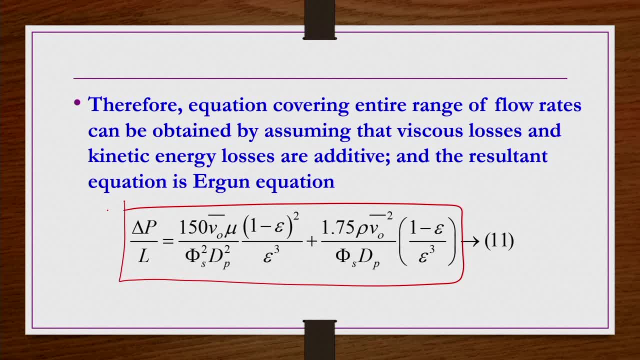 write it as: delta P by L is equals to 150 V naught bar mu by pi s square. dp square multiplied by 1 minus epsilon square, by epsilon cube plus 1.75 rho V naught bar square. Now we can see the viscous losses are having some kind of 1 minus epsilon whole square. 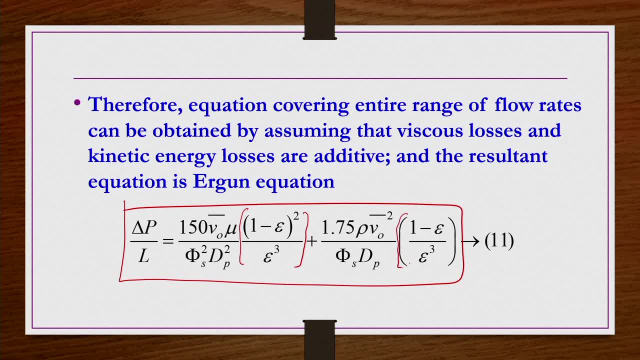 by epsilon cube terms, and then, on the kinetic losses, the second term is having 1 minus epsilon by epsilon cube terms. okay, So one should be clear, careful about them, and then indeed we can find out the reason why it is So. this is the Ergun equation. 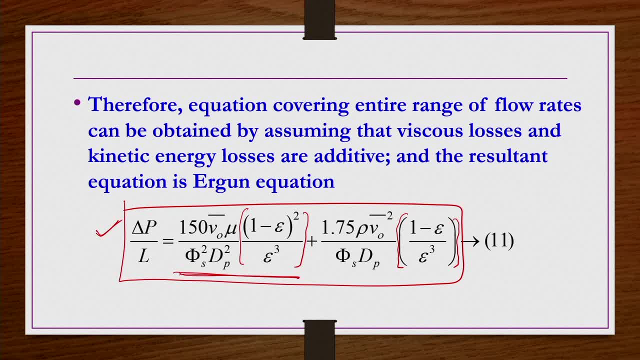 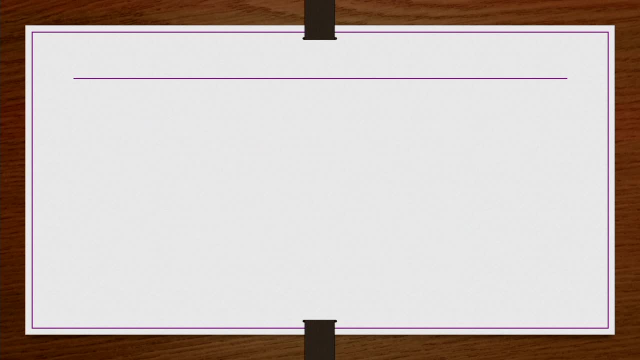 This first part is, you know, Kozeny-Carman equation. The second part is the Burke-Plummer equation. If you add them together we get Ergun equation which is valued for all Reynolds number, small to large Reynolds number, including the intermediate range of Reynolds numbers. 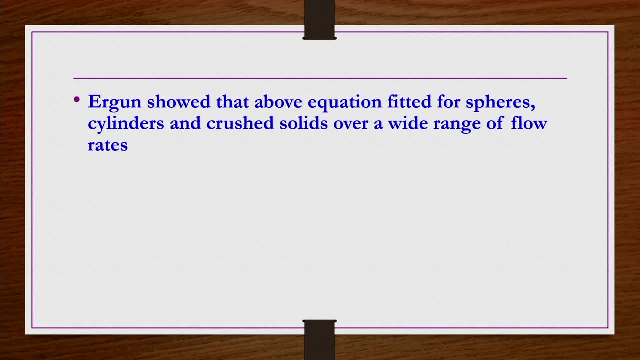 So Ergun showed that above equation fitted for spheres, cylinders and crushed solids over a wide range of flow rates. He has done several experiments for different types of packing material, So Ergun showed that above equation fitted for spheres, cylinders and crushed solids. 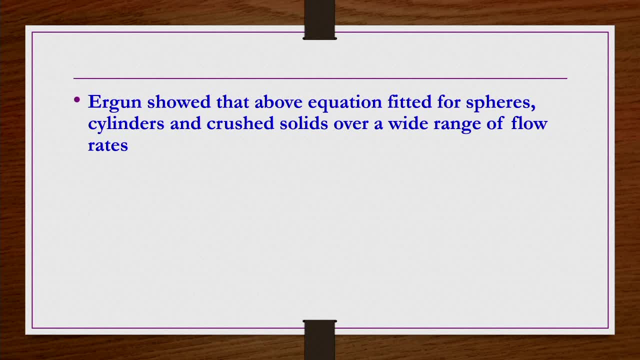 over a wide range of flow rates. He got hisущ chiral for each material, packing material, and by varying large range of flow rates. and then you find out, whatever the Ergun equation, the previous equation we have seen, that is, you know, valid for, you know, wide range of flow rates and in different types of packing. 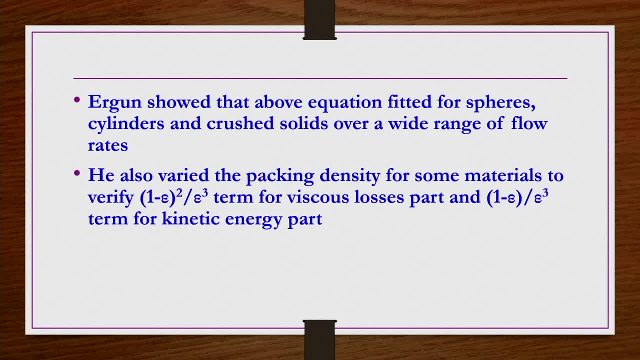 material. He also varied the packing density for some materials. to verify why 1 minus epsilon square by epsilon cube, term for viscous loss's part, that is, first part in the right hand side. And then why 1 minus epsilon by epsilon cube part for the kinetic losses. 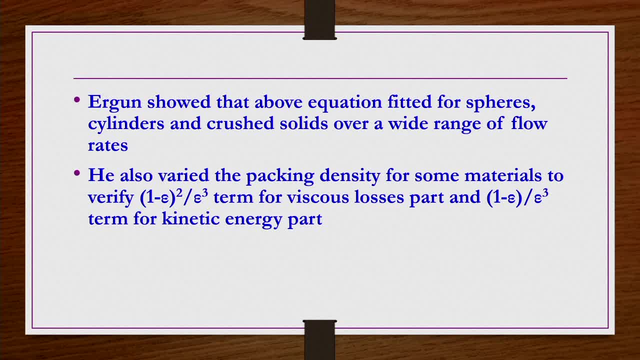 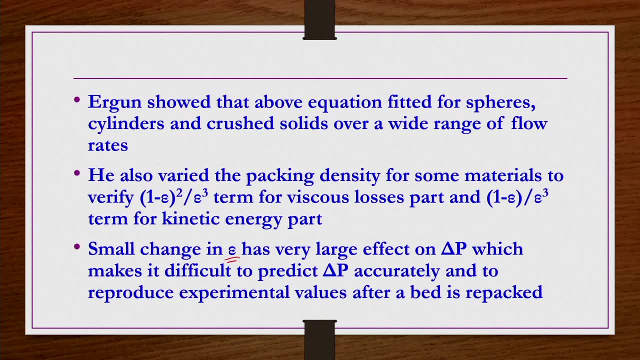 So that is Mr Ganesh's experiment, Thank you. kinetic energy part- that is second part that also he found. And then he found that small changes in epsilon has a very large effect on delta p, which makes it difficult to predict delta p accurately and to reproduce experimental values. after a bed is repacked: 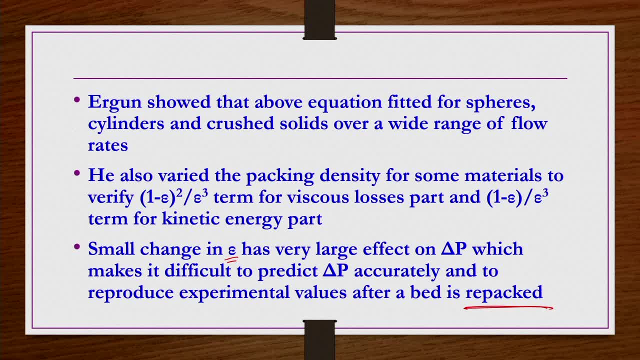 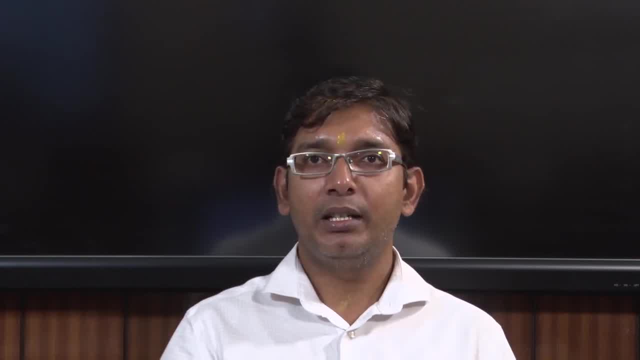 Once the bed is repacked, what will happen? That is going to have a kind of void. space is going to change. It is not going to be same packing as a kind of initial packing. So under such conditions, once the repacking is done, so there would be small changes in. 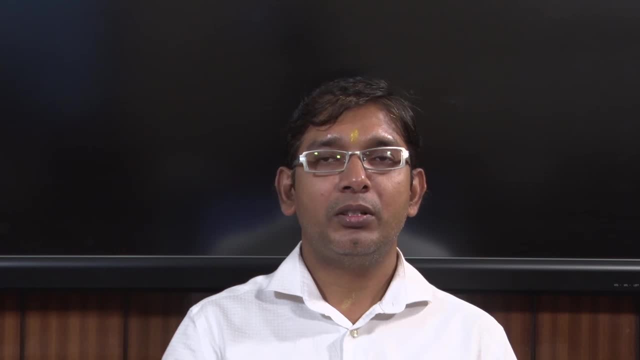 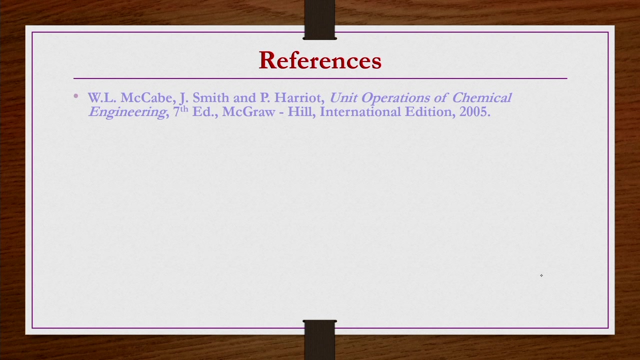 epsilon and then definitely the delta p is going to be strongly being affected by this epsilon. So reproducibility of experimental results are found to be very difficult, especially when the bed is repacked. So the references. the lecture presented here is primarily on the 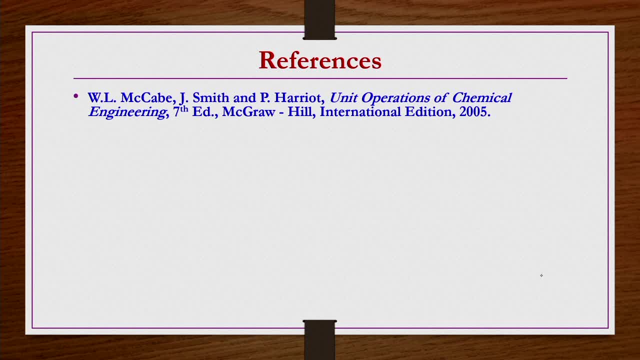 prepared from this reference book. Unit Operations of Chemical Engineering by McCabe, Smith and Harriot. The Unit Operations of Particulate Solids: Theory and Practice. Artiga-Rewas by Artiga-Rewas can also be a good reference book. Coulson and Richardson's Chemical Engineering Series by Richardson and Harker, second volume. 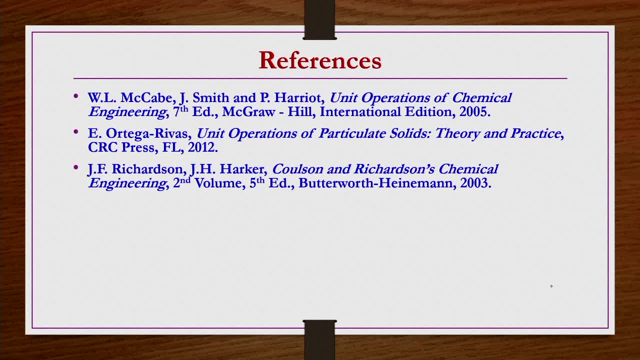 you know, is also a kind of good reference for this kind of this particularly flow through packed beds. Some applications have been taken from this reference book Transport Processes and Unit Operations by John Copliss for this lecture, And then some applications are also taken. 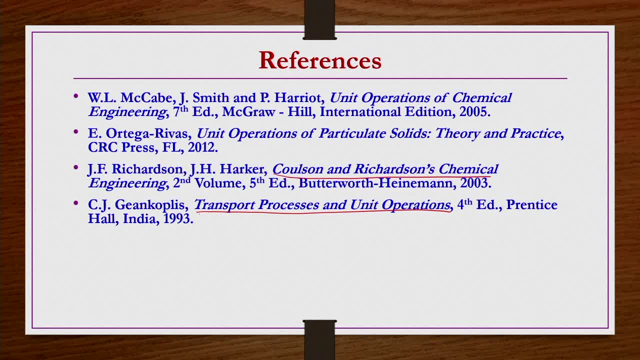 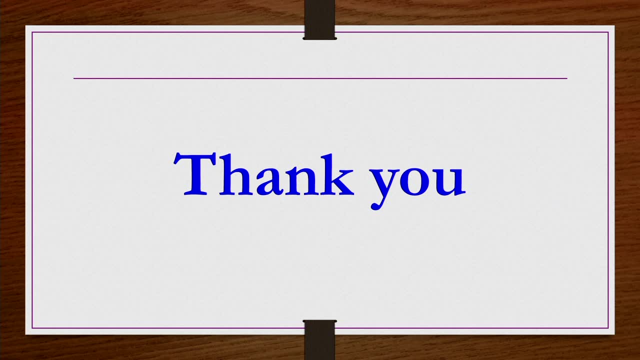 from this Coulson and Richardson's Chemical Engineering Series, second volume. Other reference books could be, like you know, Better Options or Unit Operations by Brown et al, and then Introduction to Chemical Engineering by Badger and Banchero. Thank you, Thank you.